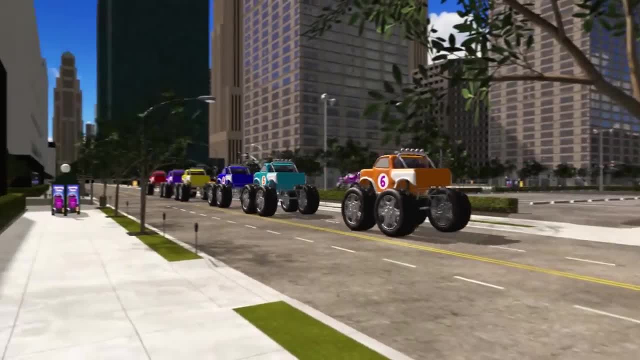 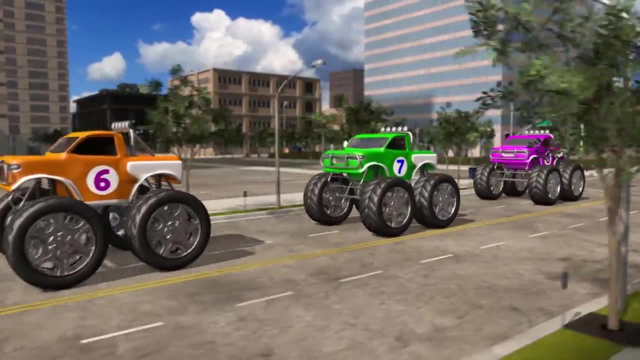 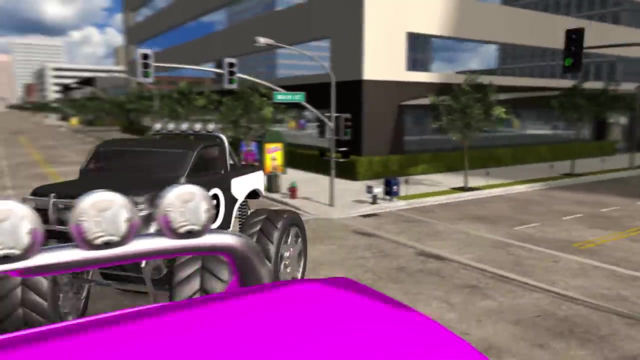 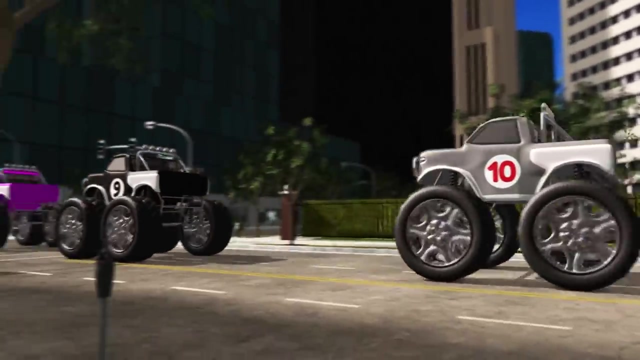 And the orange one is number 6!. Whoa, Look at those huge tires on number 7!. Here's number 7 and number 8! Look out, Here comes number 9 and number 10! Now we have all 10 monster trucks. 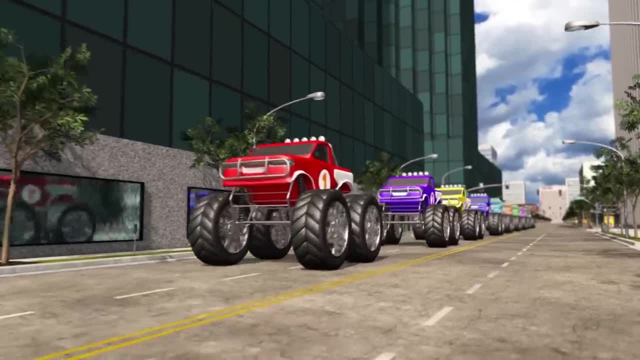 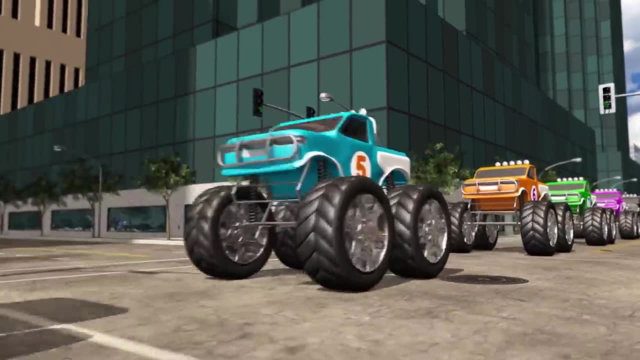 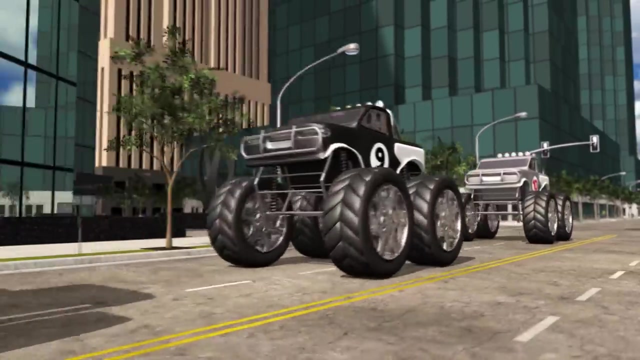 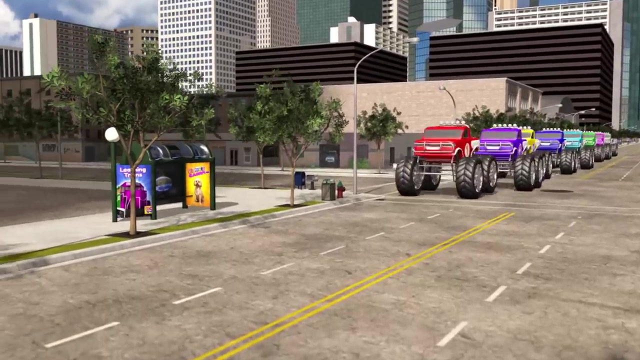 Let's count them as they go by: 1, 2, 3, 4, 5, 6, 7, 8, 9 and 10!. Hey, number 1! You'd better slow down. Oh no, Not that slow. Watch out. 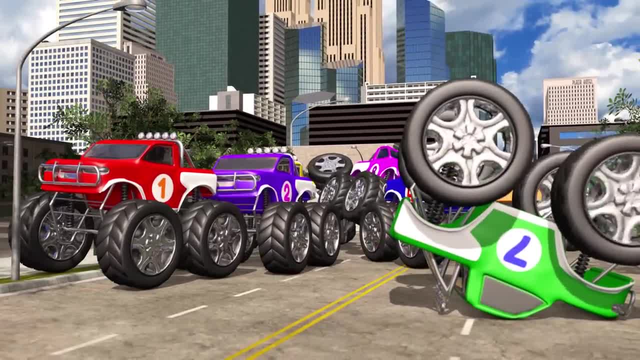 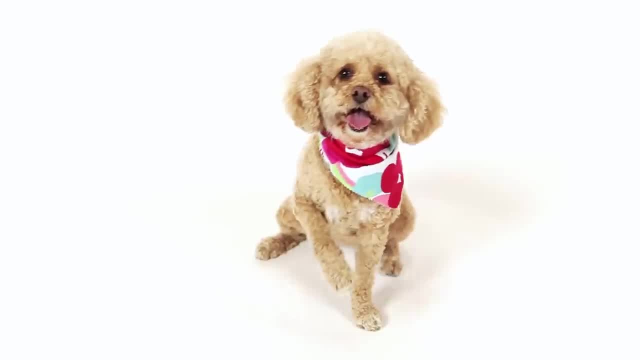 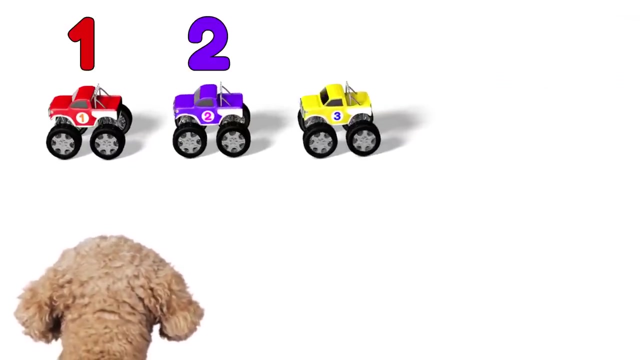 Uh oh, Looks like we're gonna need a tow truck. Hey, Lizzy, Wasn't that fun. Let's review the numbers 1 to 10 with some fun toy monster trucks: 1, 2, 3, 4, 5!. 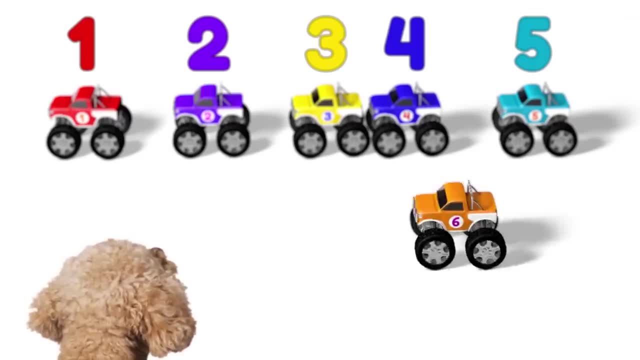 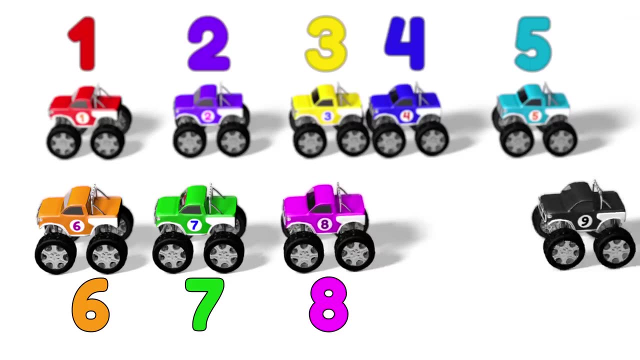 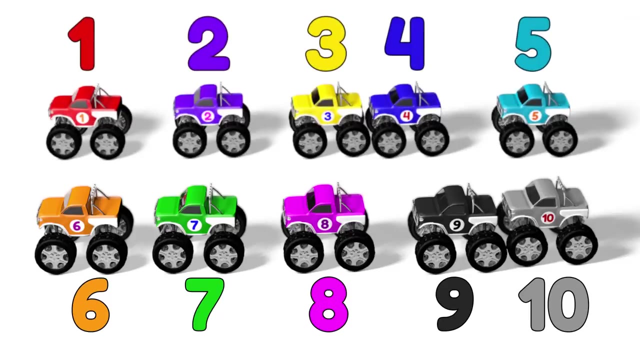 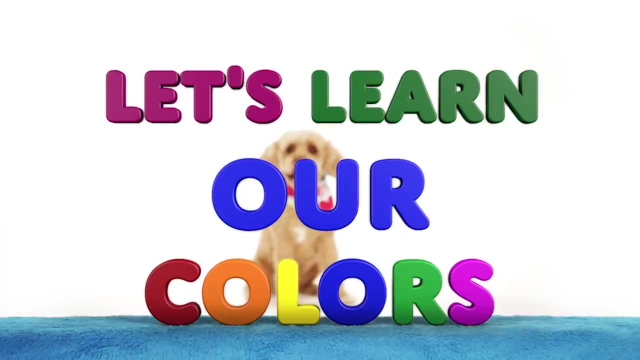 5 monster trucks: 6, 7, 8, 9 and 10!. 10 monster trucks. Hey Brainiacs, Who wants to learn some colors with Lizzy? Ok, Lizzy, stay there now. No, no wait, Lizzy. 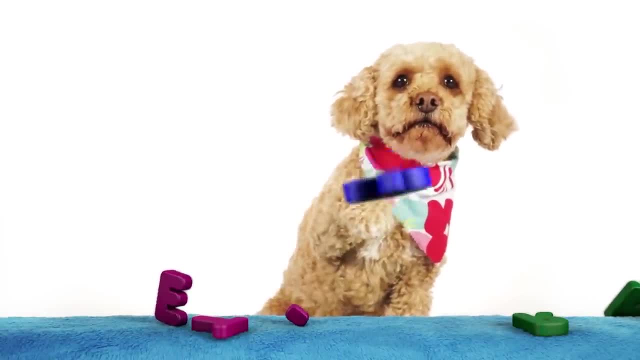 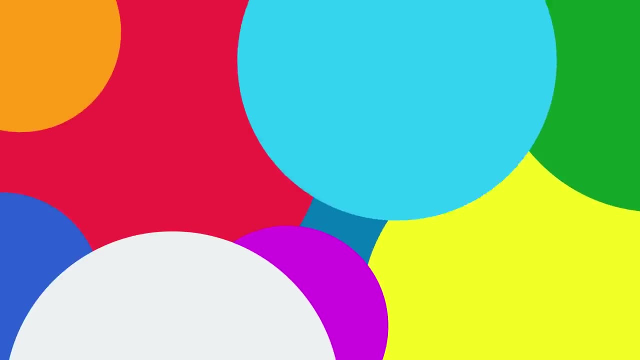 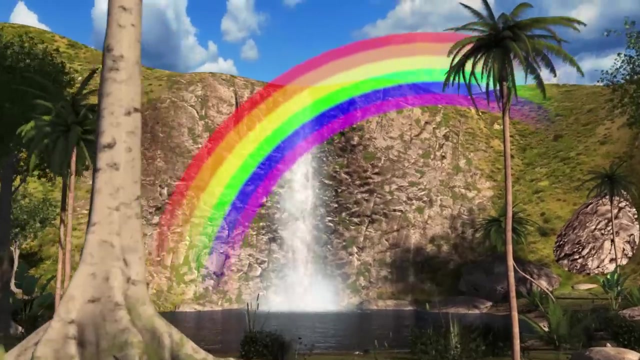 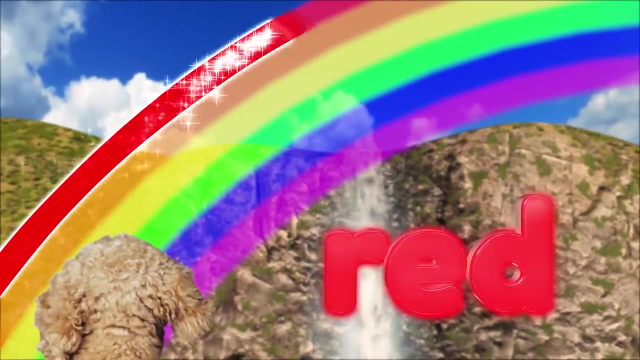 You knocked over all the letters again. Oh well, Let's take a trip to the jungle to see if we can find a rainbow. Whoa, Look at that colorful rainbow. Let's learn all the colors. This part is red, This is orange. 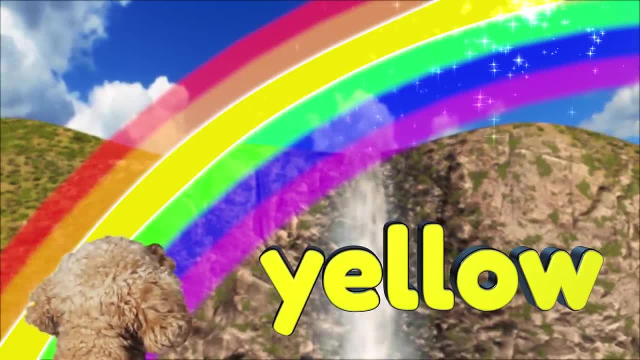 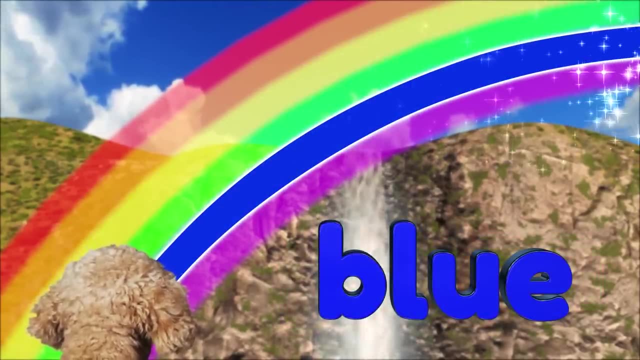 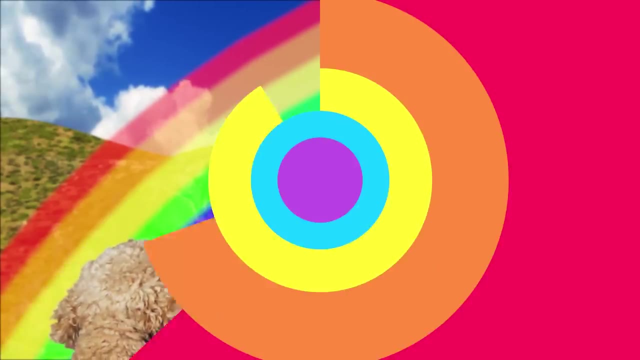 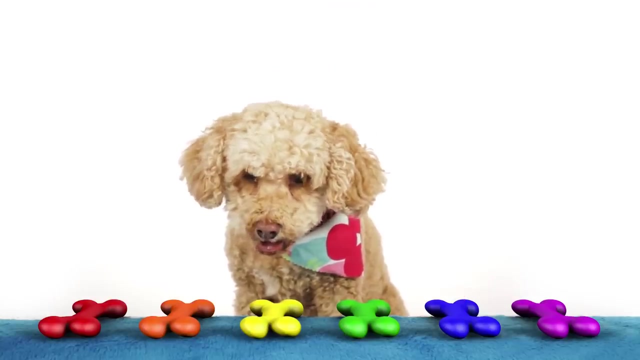 This is the color yellow, This is green, This is blue And this part is purple. Let's see if you and Lizzy can remember all of the colors. Where's the green bone, Lizzy, Red, Correct, That bone is green. 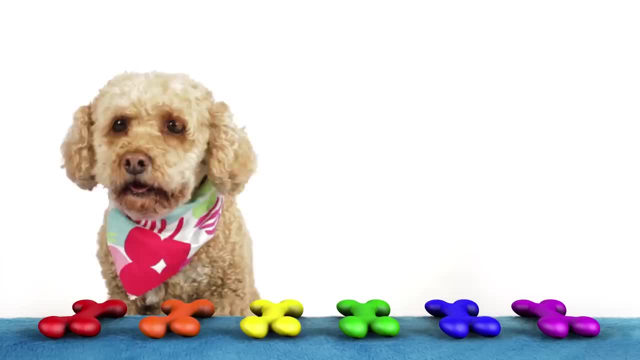 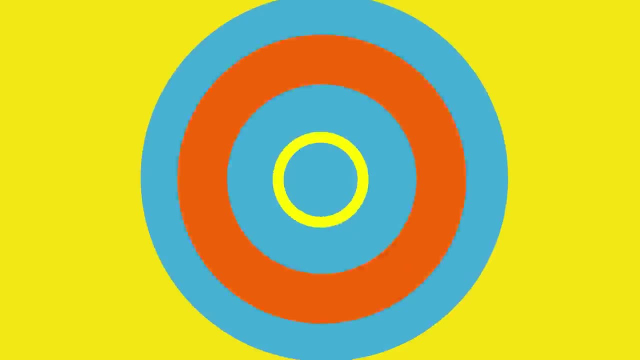 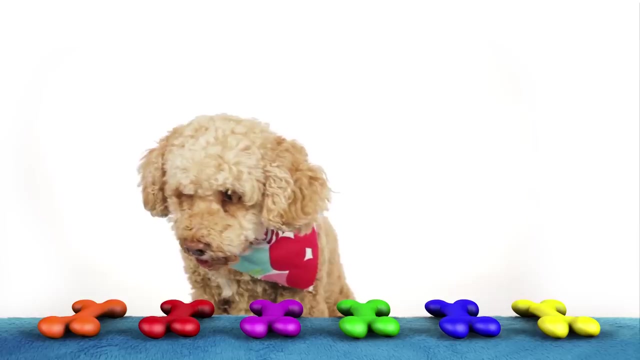 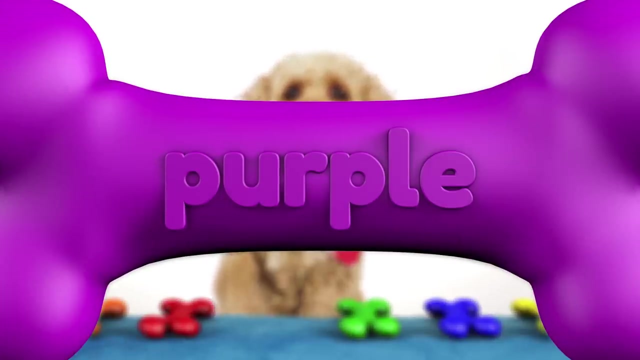 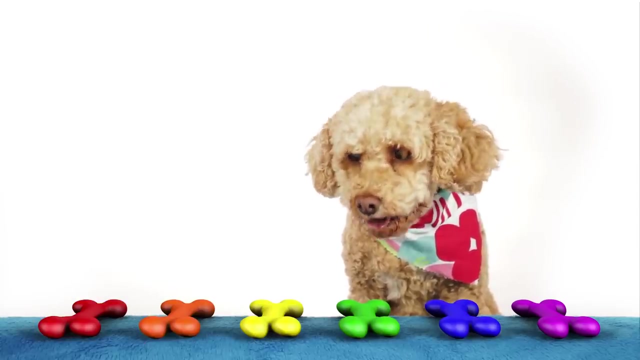 Where's the orange one? That's right Orange. How about the purple one? Can you find it? Red, Blue, Blue. Yes, There it is, The bone is purple. Can you find the blue bone? Show Lizzy, where it is. 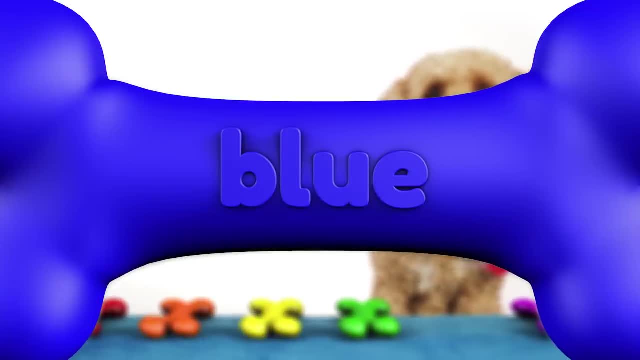 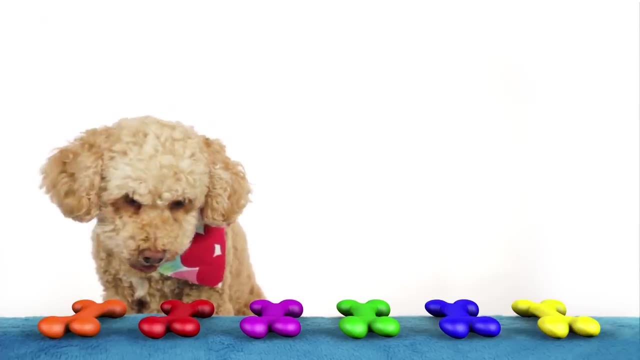 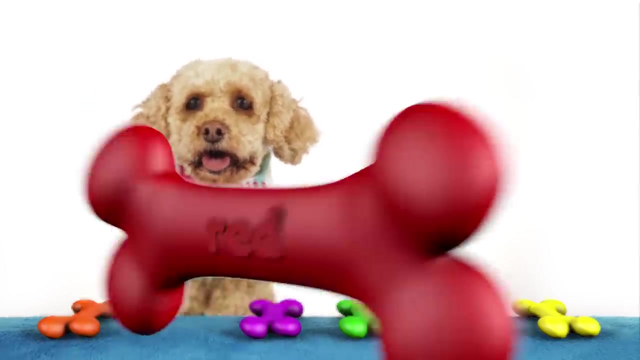 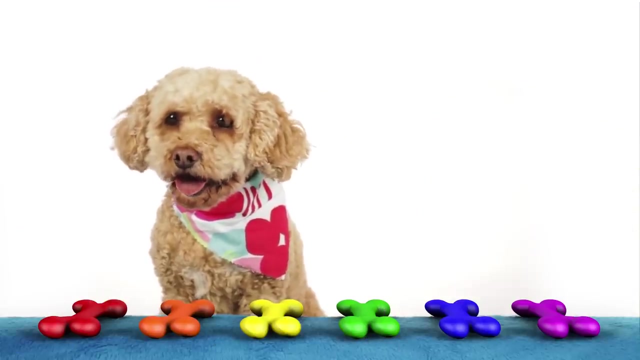 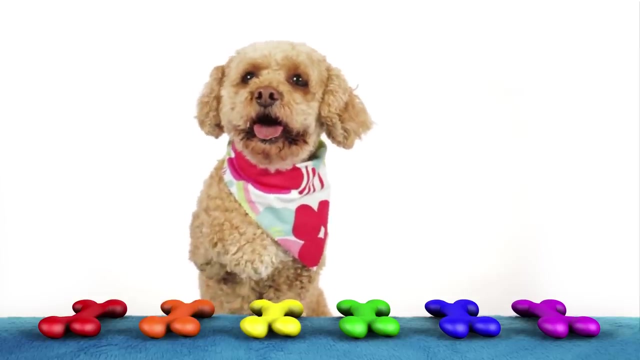 There it is Blue. Ok, Brainiacs, Can you help Lizzy find the red bone. Where could it be Perfect, This one is red. Only one more to go. Which one is yellow? Right on, That's the yellow bone. 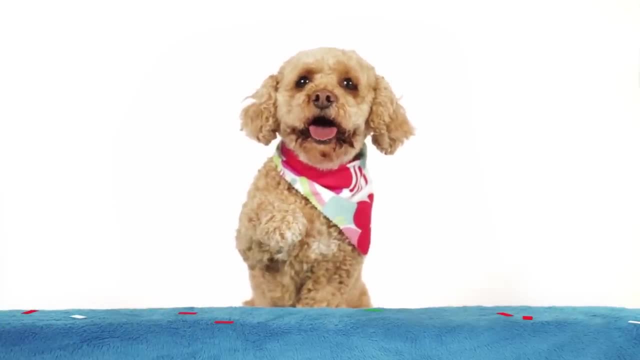 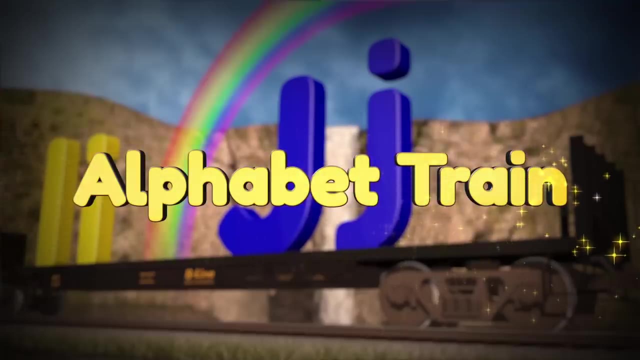 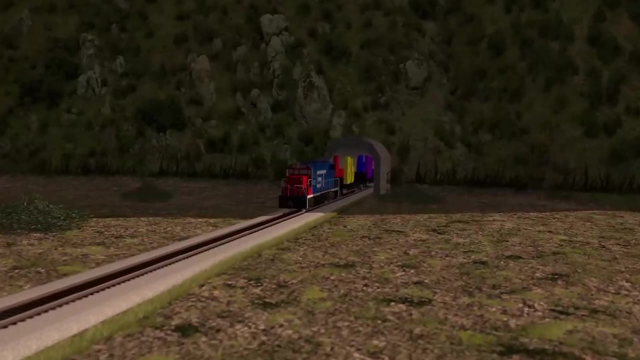 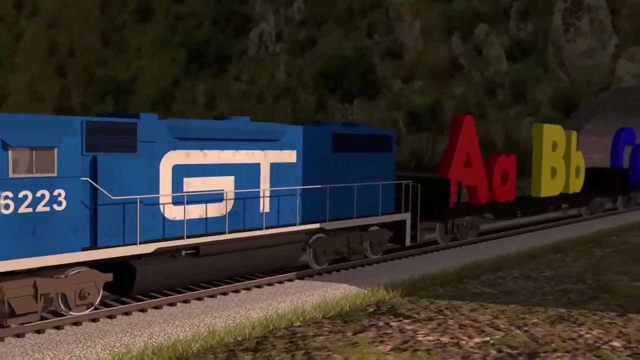 Alright, That was fun. Say bye, Lizzy, Thanks for watching And see you next time. Alphabet Train. Hey kids, Hey Lizzy. Look, Here comes the alphabet train. Look at all of the letters it can carry. It can even carry the uppercase and lowercase of each letter. 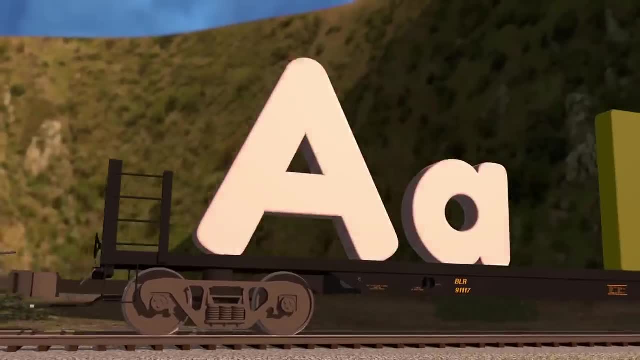 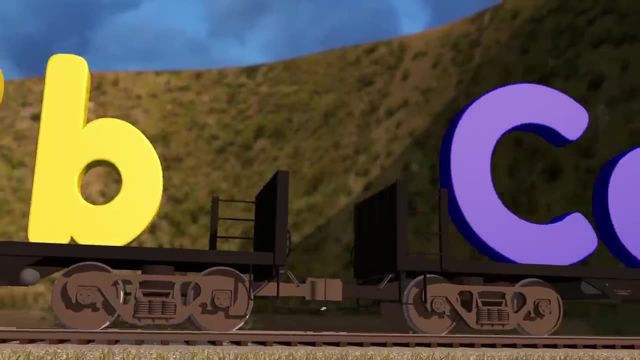 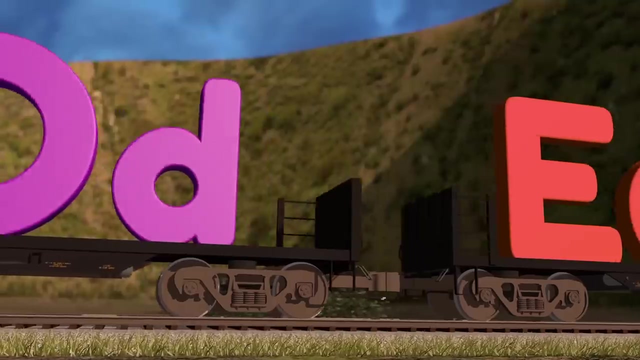 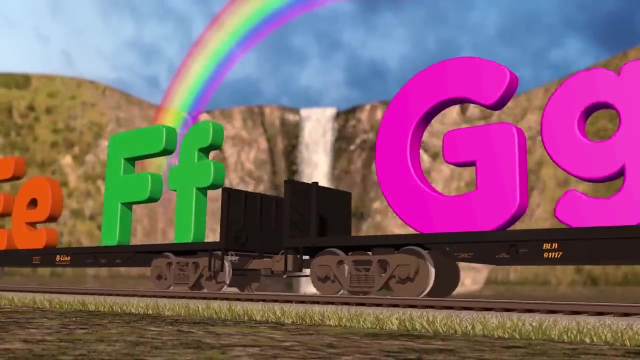 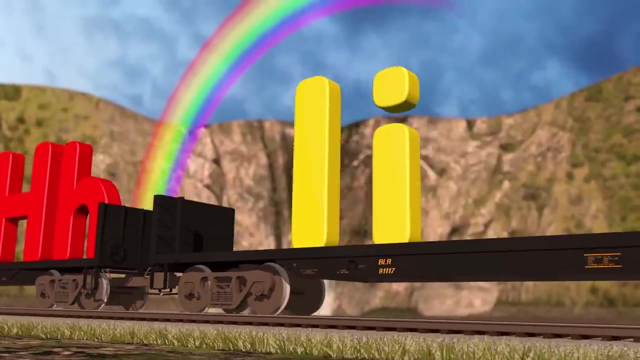 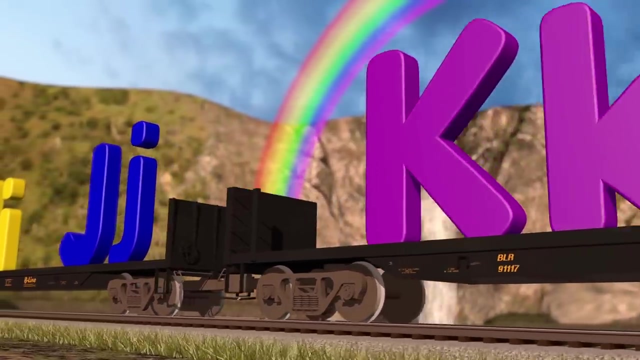 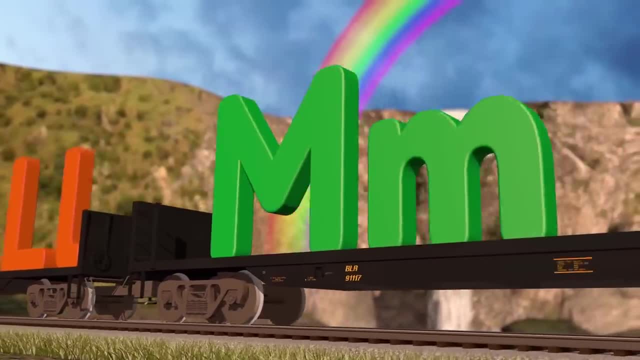 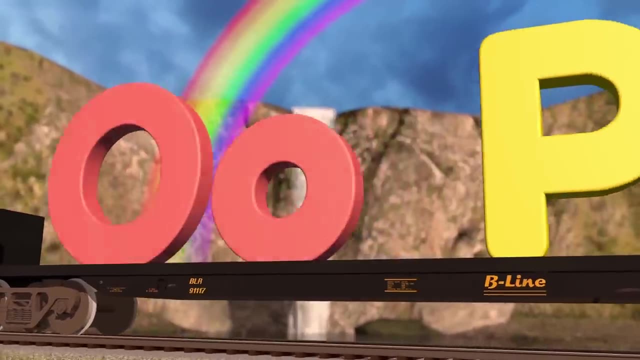 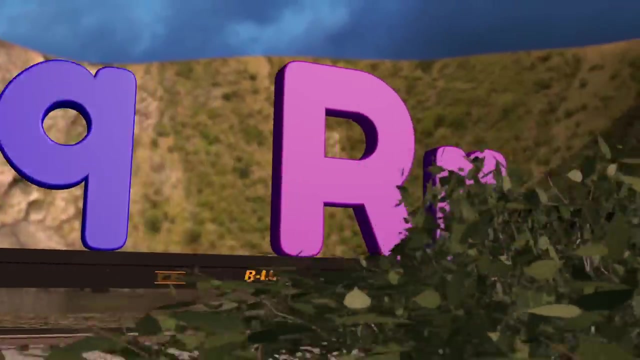 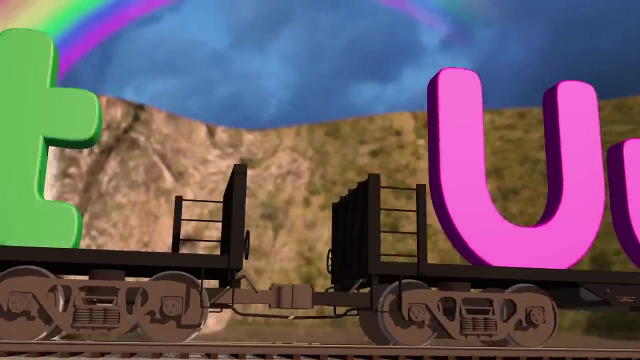 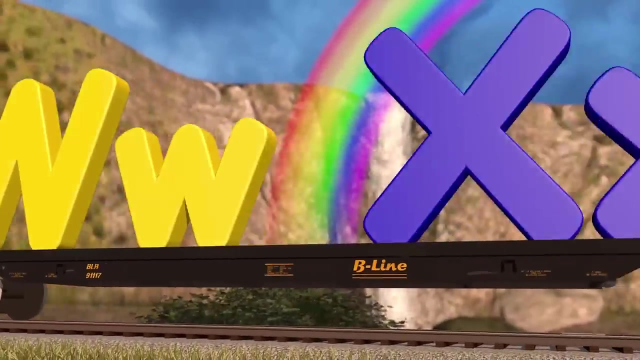 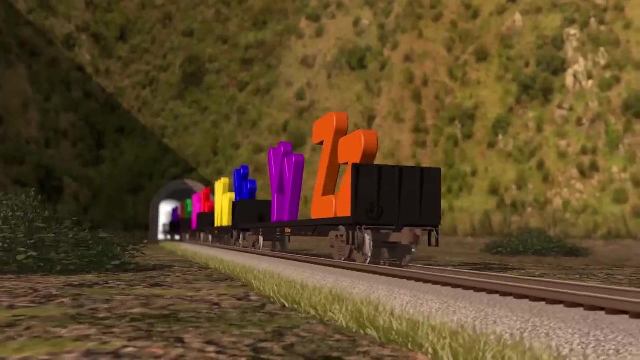 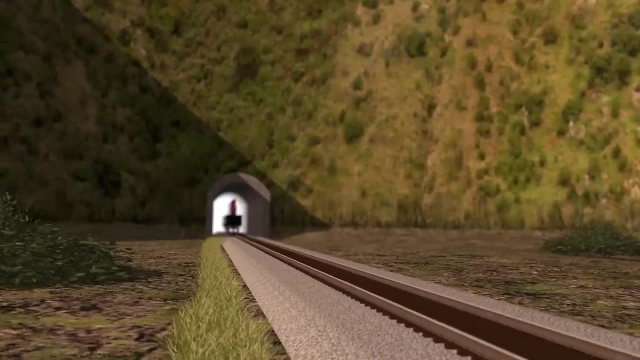 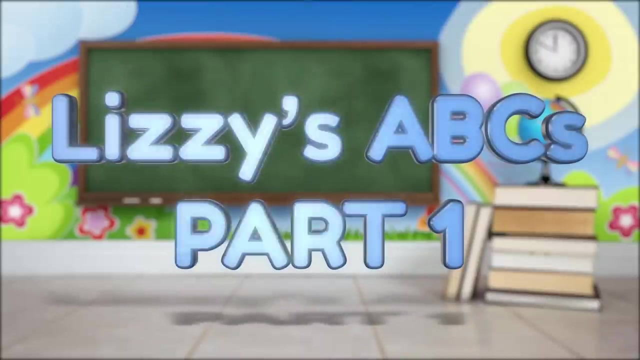 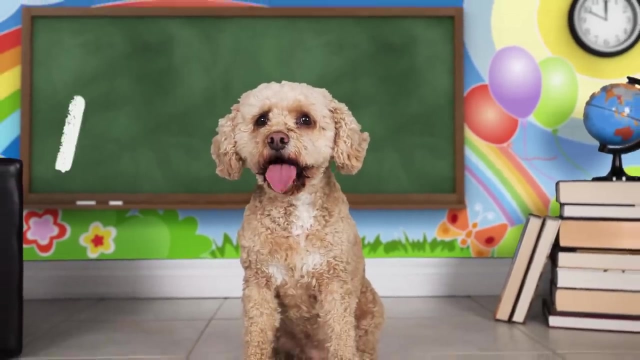 L, L, L, L, M, M, M, N, N, N, O, O, P, O, P, Q, Q, Q, R, S, T, U, V, W, X, Y, Z. Wasn't that fun? Lizzy, Lizzy, Lizzy. where are you, Hey Brainiacs? today we're going to learn our ABCs. 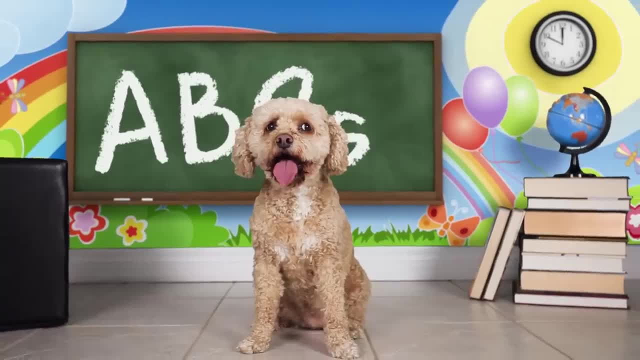 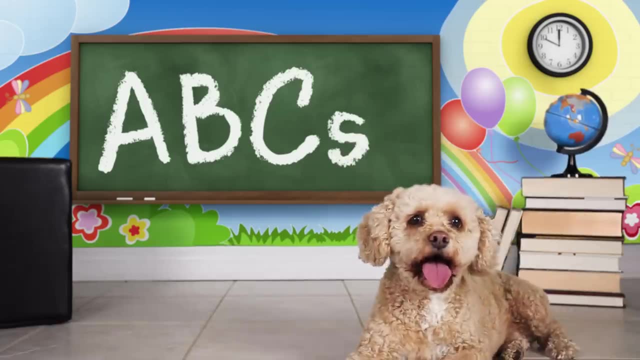 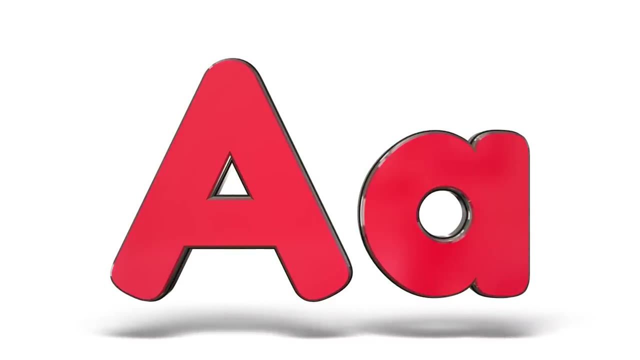 And Lizzy's here to help us find things that start with each letter. What do you say, Lizzy? Do you want to play? Alright, we're going to have so much fun. Let's get started. The first letter of the alphabet is the letter A. 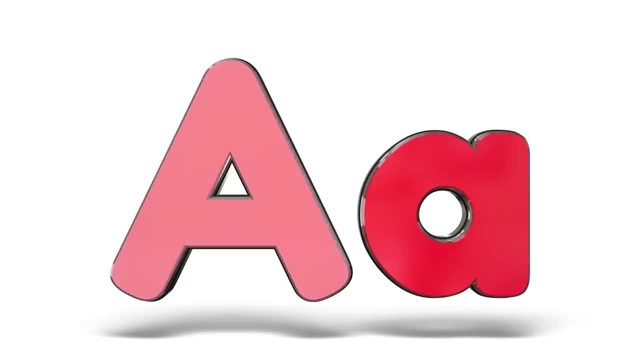 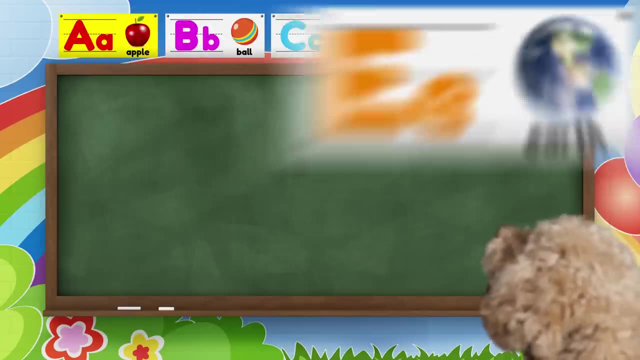 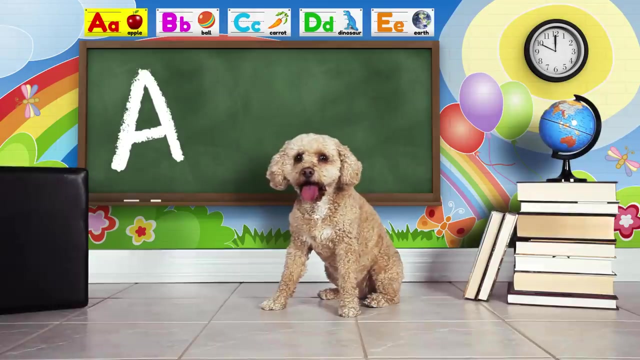 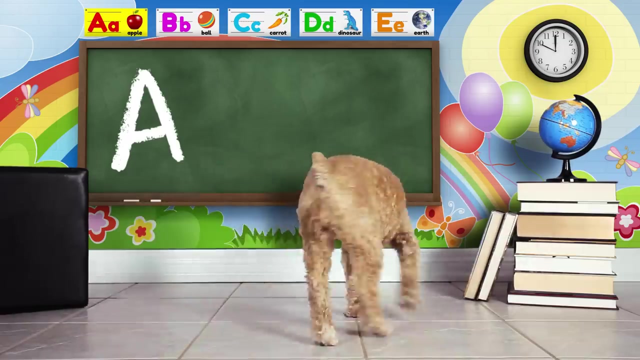 And it looks like this: This is a capital or uppercase A, This is a lowercase a. The letter A sounds like ah. ah. Okay, Lizzy, go get something that starts with the letter A. I bet you can find something in the box. 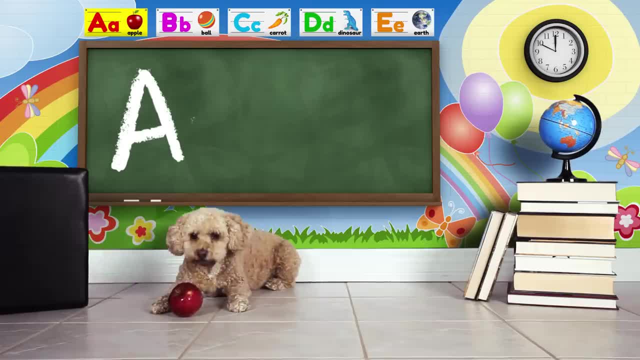 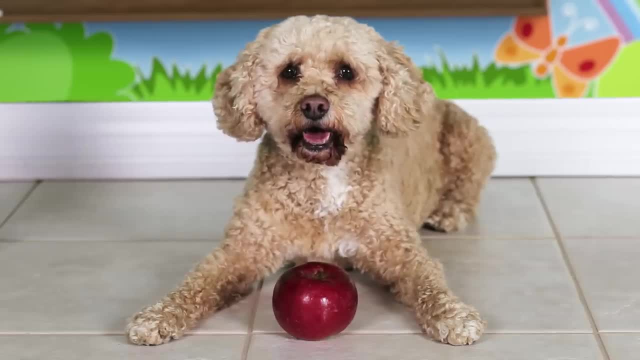 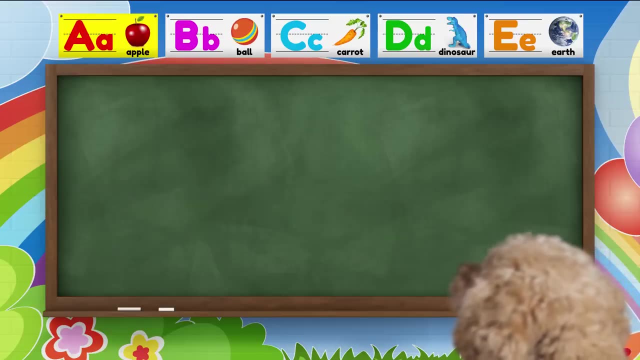 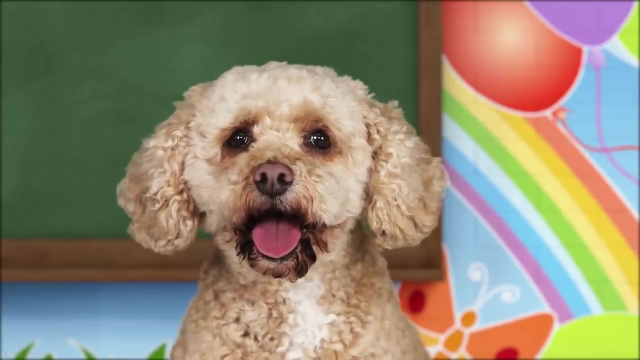 That's right. The word apple starts with the letter A. Great job, Lizzy. What a smart dog. Another word that starts with A is add, Like when you add one plus two to get three. What's another word that starts with the letter A? 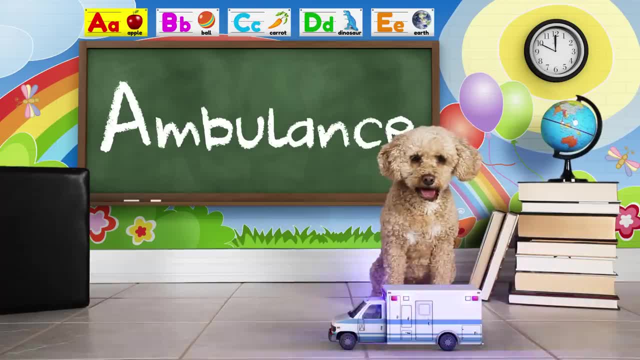 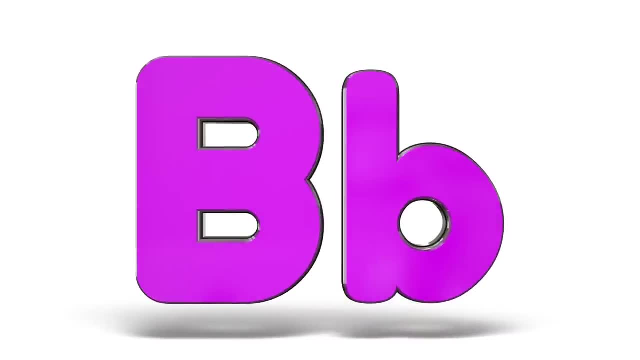 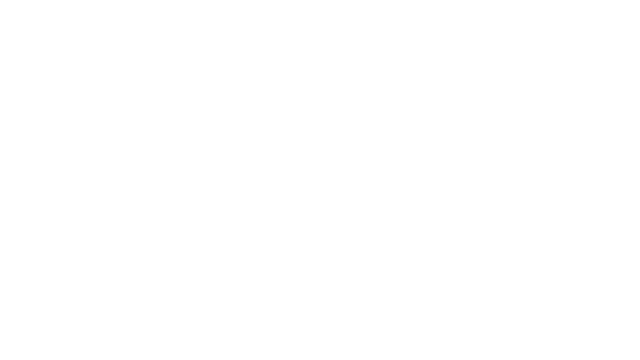 I know ambulance Ambulance starts with the letter A. I know ambulance Ambulance starts with the letter A. The next letter of the alphabet is B And it looks like this: The letter B sounds like buh buh. 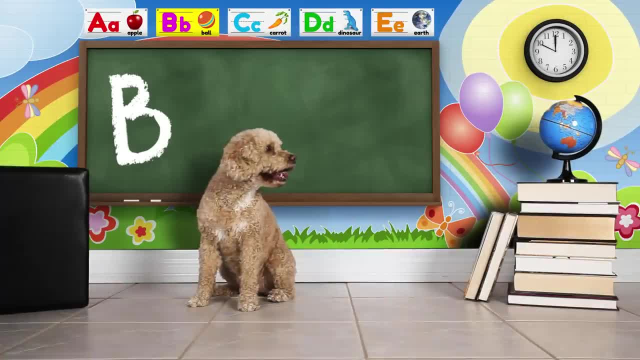 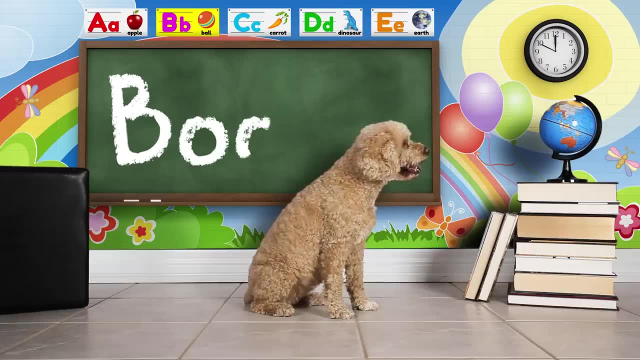 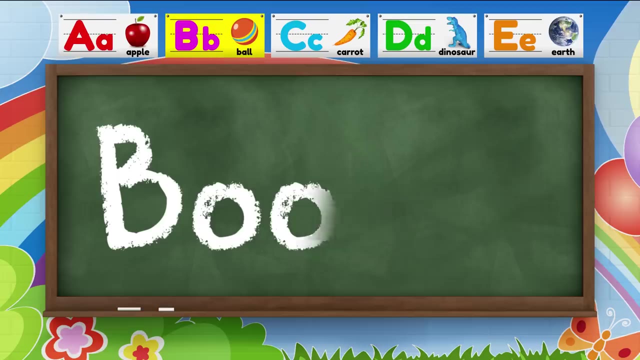 Can you see anything here that starts with B? That's right, The book starts with the letter B. Maybe, when you learn your alphabet, you'll be able to read books all by yourself. Maybe, when you learn your alphabet, you'll be able to read books all by yourself. 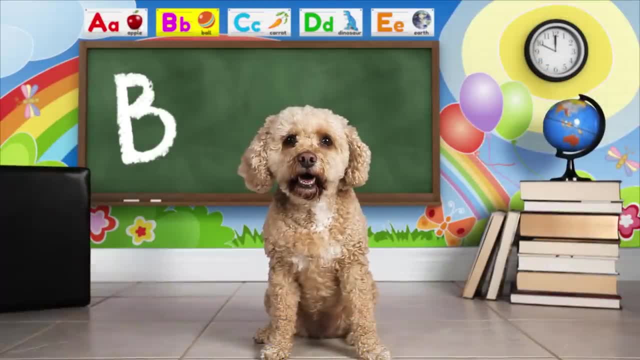 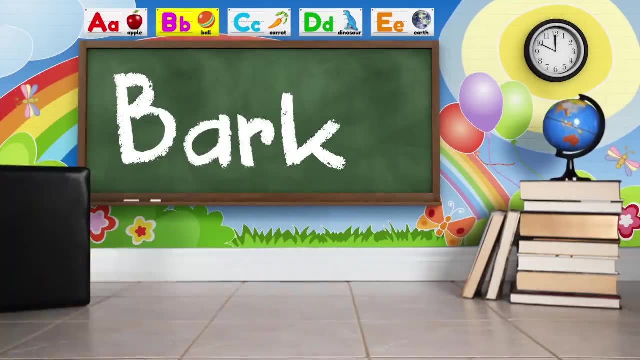 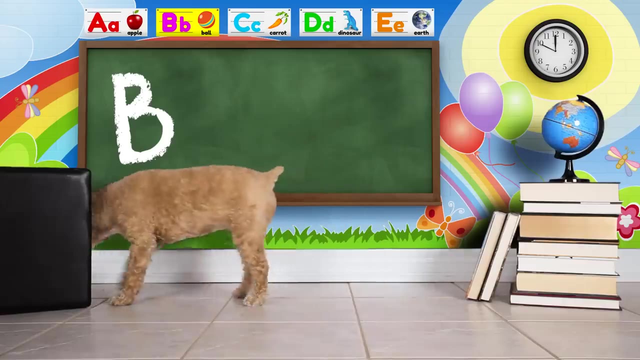 What else starts with B? I know What sound does a dog make: Bark, Haha, you're right, A dog barks. Bark starts with the letter B. Okay, Lizzy, go get a toy that starts with B. Yes, 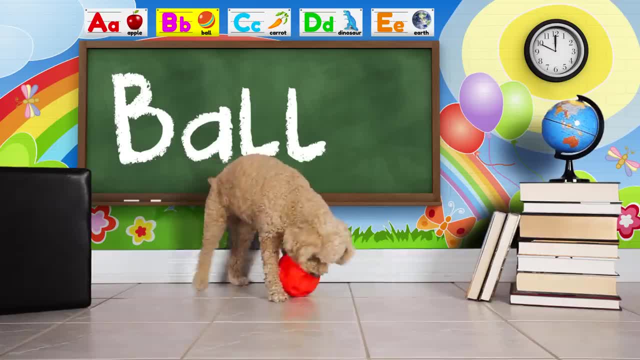 Ball starts with B. Yes, Ball starts with B. Yes, Yes, You're like me when I speak. It is a nice thing for a small thing to do. Wait, come back. we're not done yet. No, no, this way. 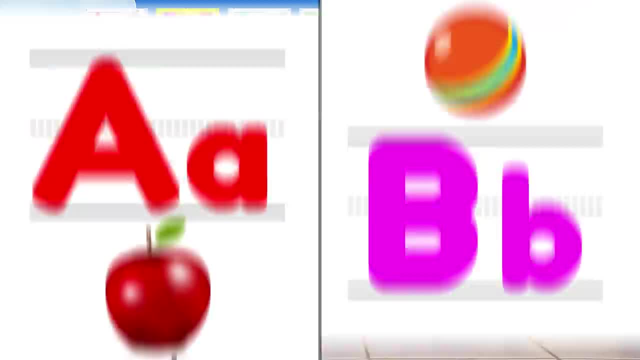 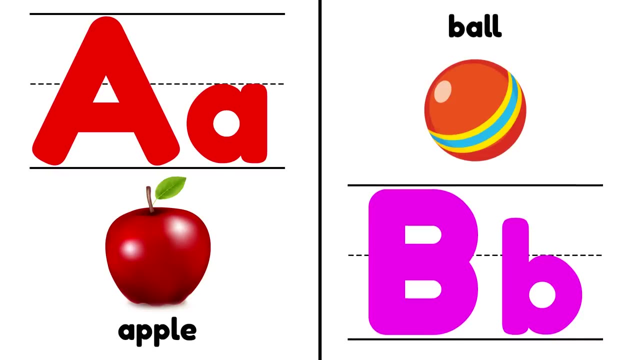 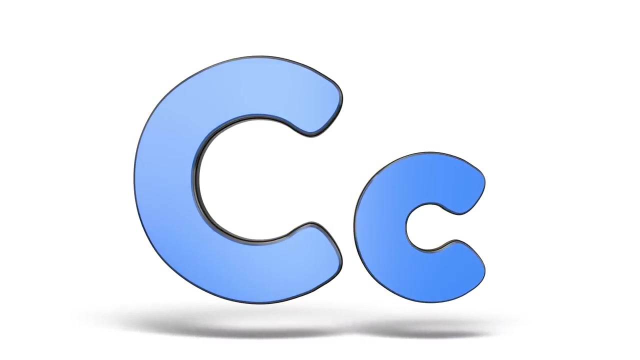 Uh A-paw E tylko buh A for apple, Buh buh B for ball. Next up is the letter C And it looks like this: C C. The letter C sounds like ku ku. 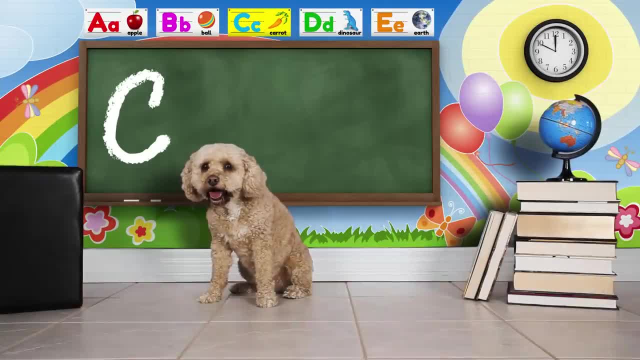 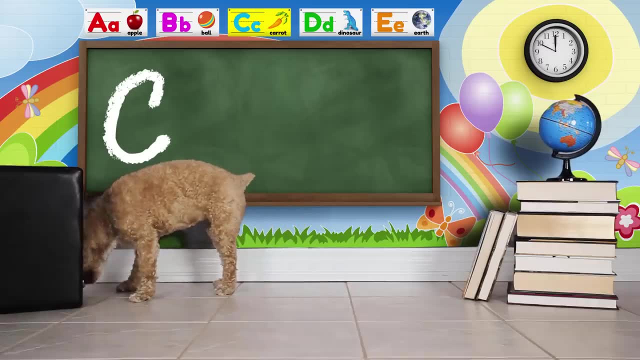 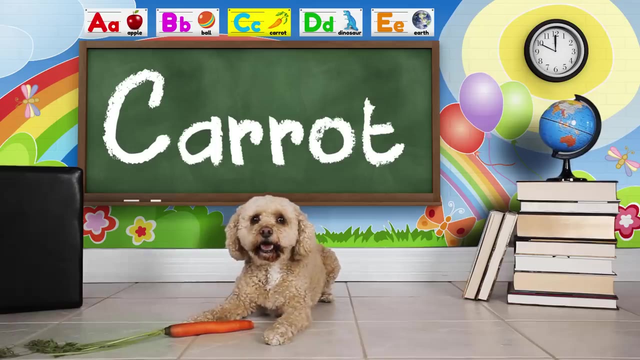 Hey Lizzy, Why don't you film the book today? Why don't you show them what your favorite vegetable is? I bet there's one in the box. It's a carrot. Carrot starts with the letter C. I like carrots too, but not as much as Lizzy. 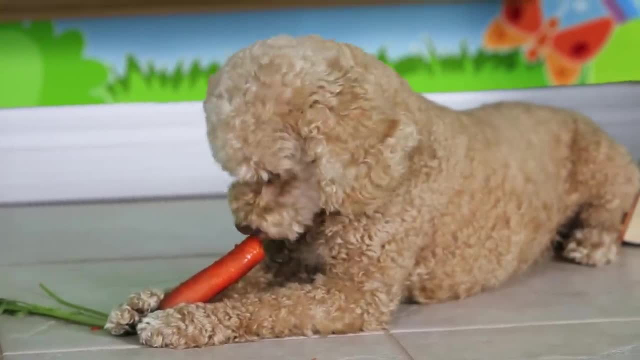 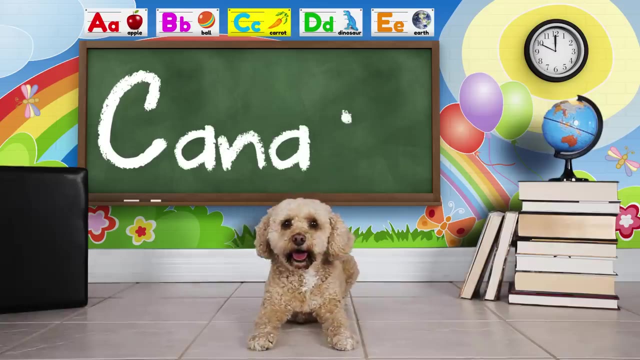 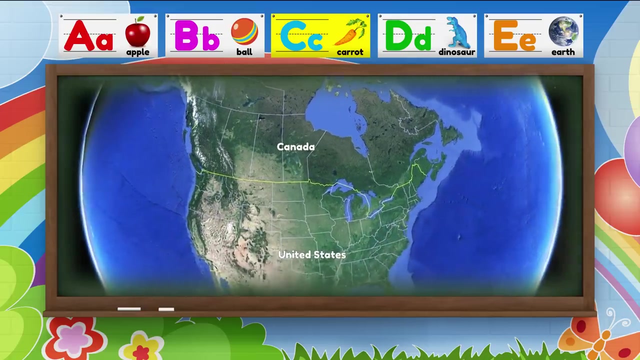 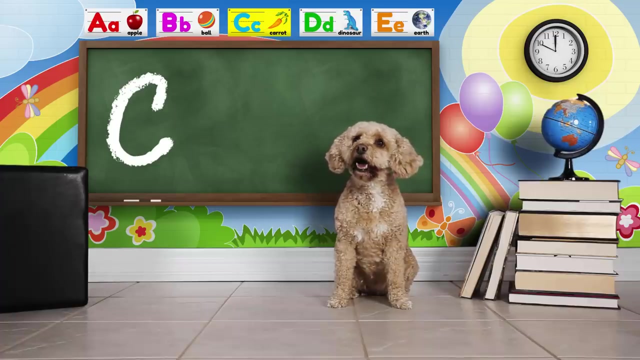 She could eat them all day. Hey, do you know what country Lizzy is from? Lizzy lives in Canada. Canada is in North America, just above the United States, and Canada starts with the letter C. Lizzy's good at playing catch. 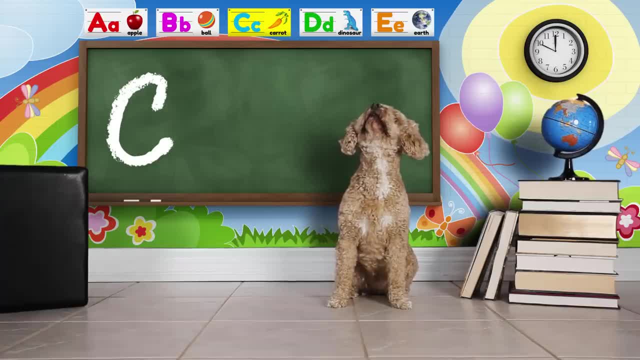 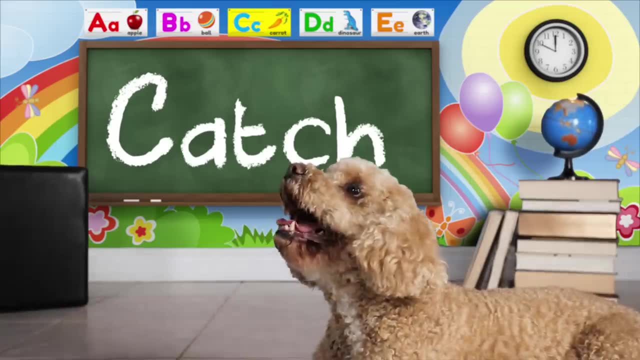 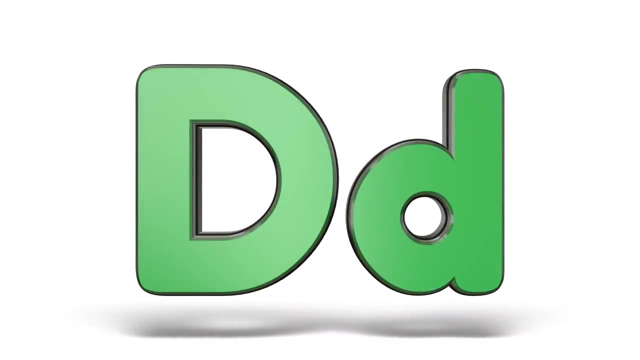 Let's see if she can catch her ball Ready Lizzy. One, two, three, Nice catch. The word catch starts with C. The next letter we have is the letter D and it looks like this. D sounds like duh duh. 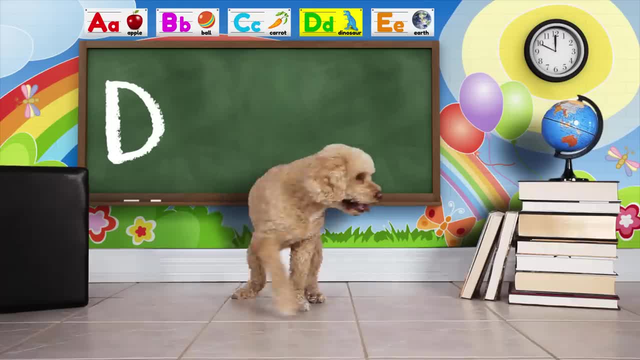 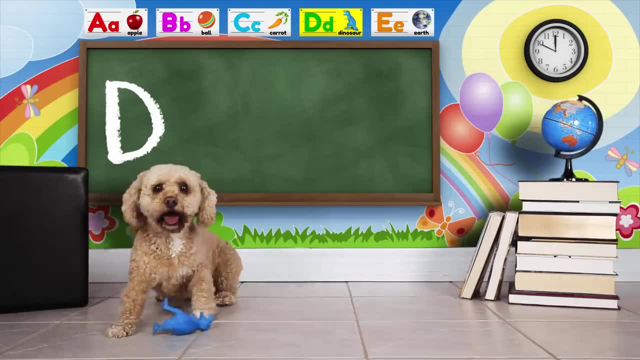 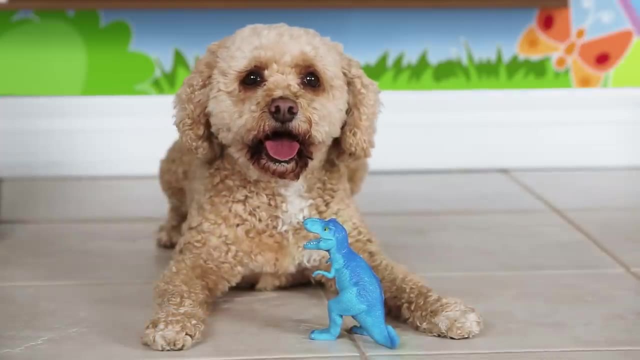 Alright, Lizzy, can you find something that starts with the letter D? Good girl, That's right. Dinosaur begins with D. That looks like one of my favorites, a Tyrannosaurus Rex. I know something else that starts with D. 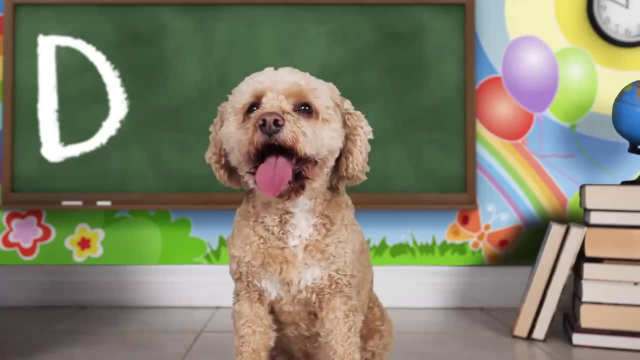 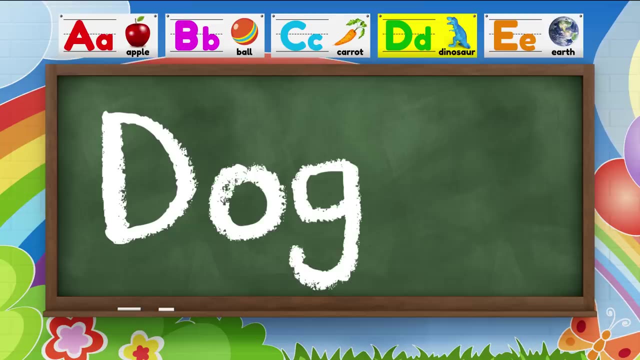 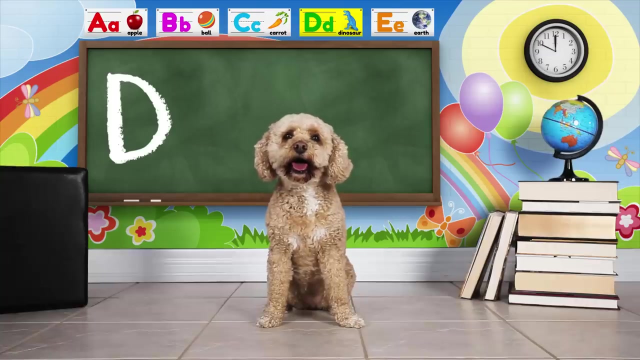 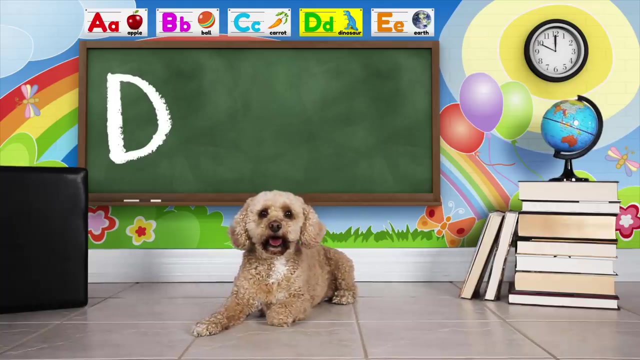 Let's see what it is. Do you know what it is? That's right, Lizzy is a dog, And dog starts with the letter D. Ok, Lizzy, why don't you show them something else that starts with D? Good job. 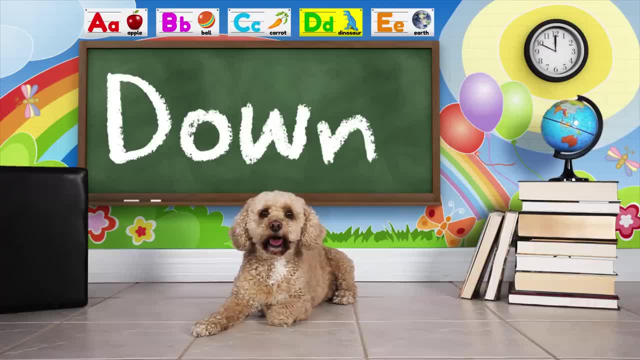 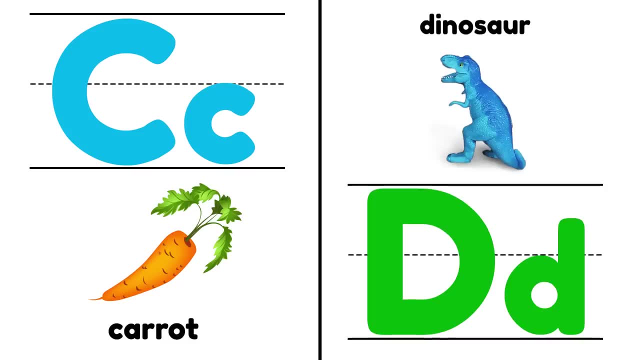 You're so smart, You know the trick. down And down starts with the letter D. Good job, Kuh kuh. C for carrot, Duh duh D for dinosaur. Do you know what letter comes after D? 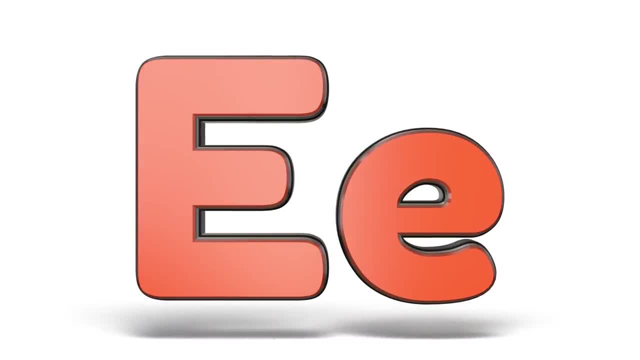 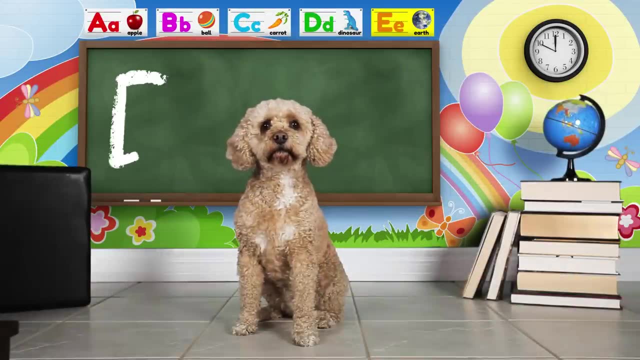 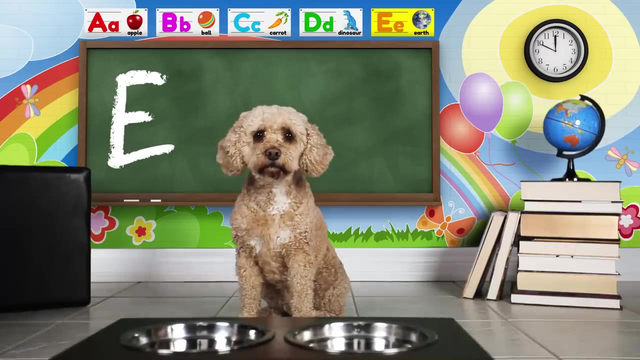 It's the letter E and it looks like this. E sounds like eh. eh, Lizzy's been working really hard and I bet she's hungry. Let's give her something to eat. Here you go. Okay, eat up. 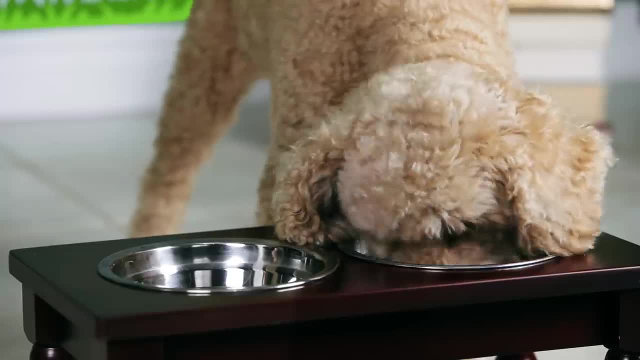 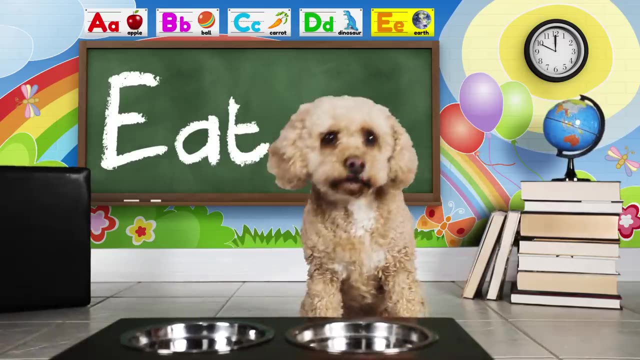 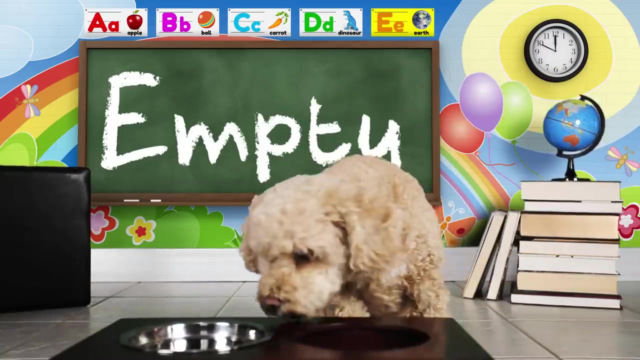 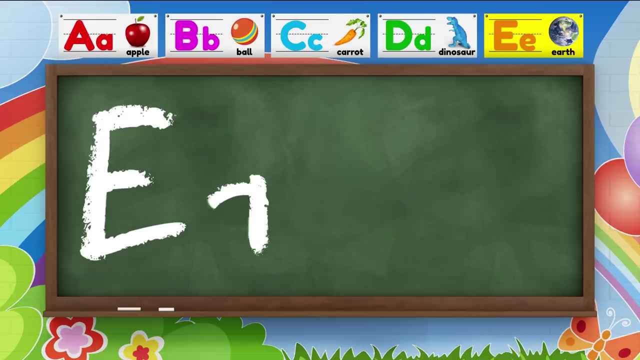 The word eat starts with the letter E. All done, I guess she was hungry. Her bowl is empty. Hey, empty starts with the letter E too. Do you know the name of the planet we all live on? Our planet is called Earth. 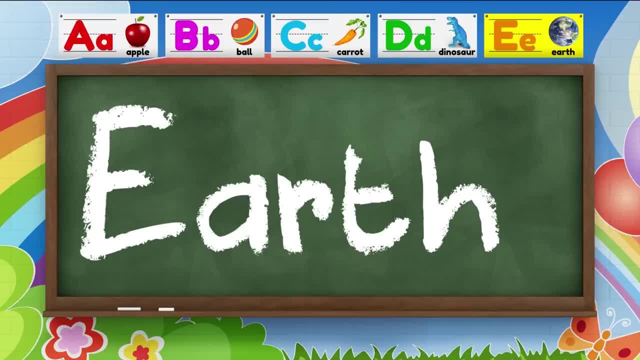 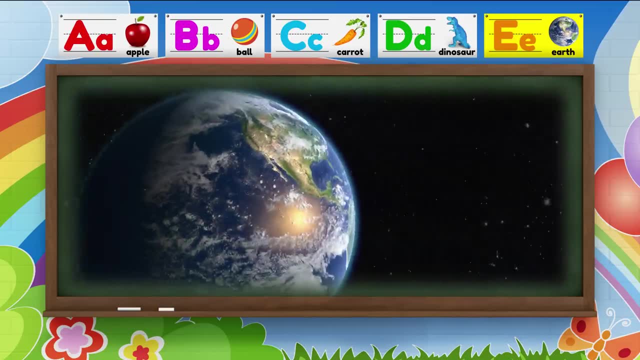 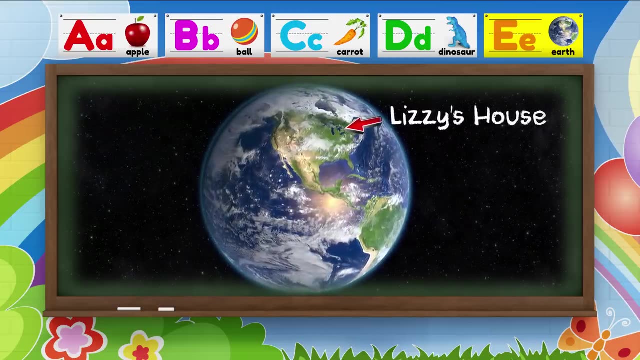 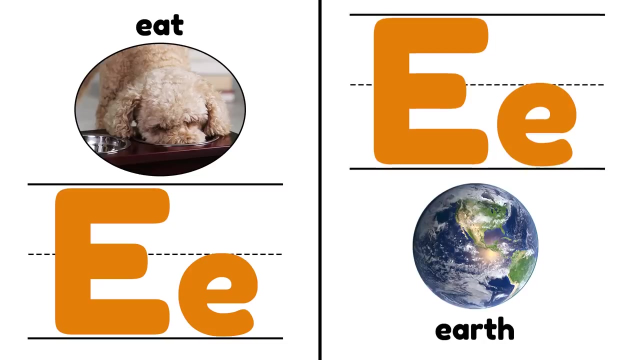 and Earth starts with the letter E. Earth is one of the eight planets that go around the sun. Wow, isn't it beautiful? Look that's where Lizzy lives. E, E, E for eat, Eh, eh, E for Earth. 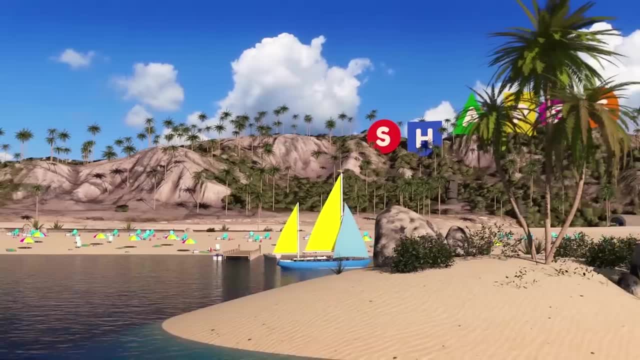 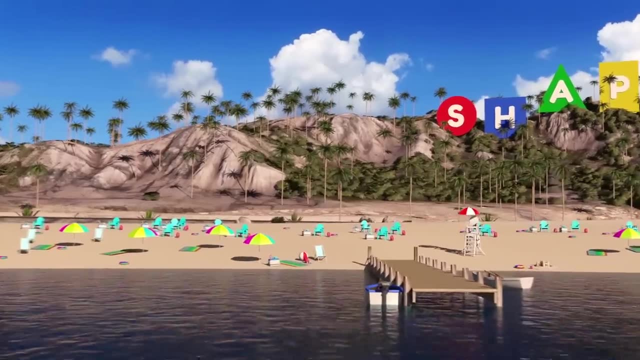 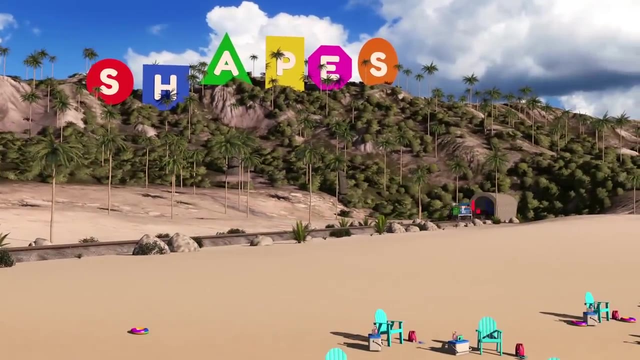 Shapestring. Hey, Brainiacs, welcome to Shapes Island. Today we're going to learn about shapes and how to find them all around you. Hey, look, here comes Lizzy and the Shapestrain to teach us all about the different shapes. 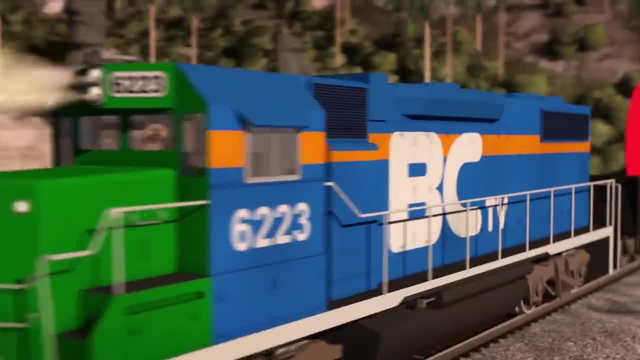 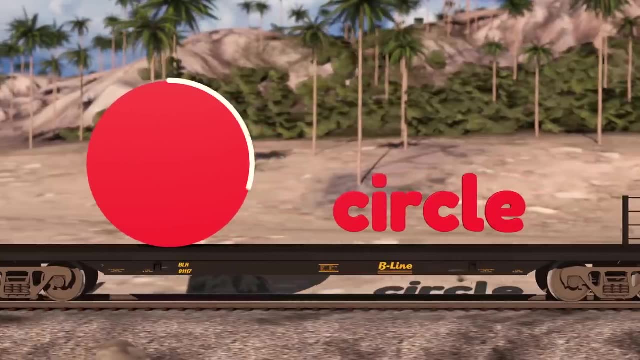 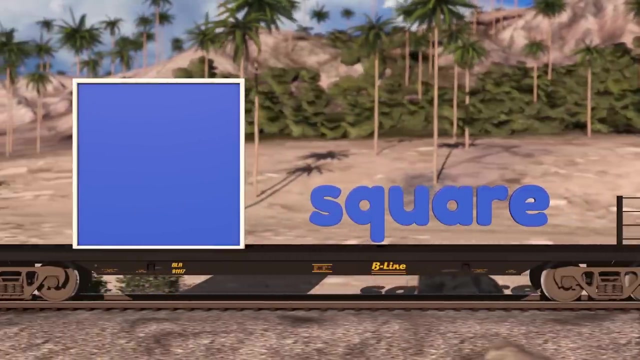 Hi Lizzy. Okay, are you ready to start? Let's go. This is a circle. A circle is round, so it doesn't have any sides. This is a square. A square has four sides that are all the same. Here is a triangle. 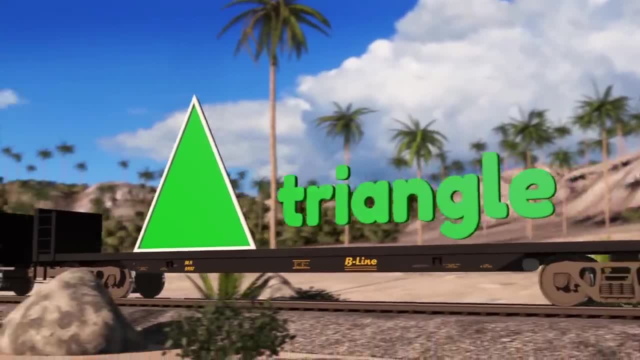 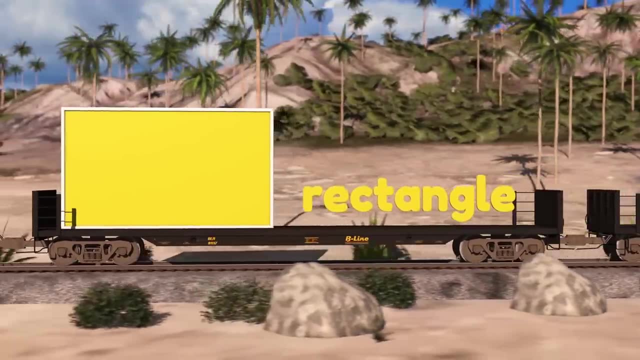 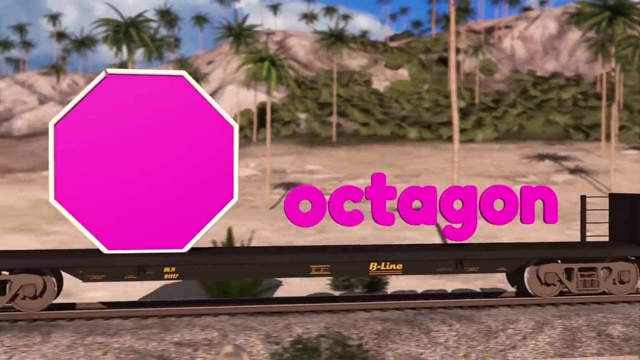 A triangle has three sides. A square has four sides ofely the same. This is called a rectangle. A rectangle has four sides, like a square, but two sides are longer than the others. Pianos have four sides, like squares. This shape is an octagon. Octagons have eight sides. 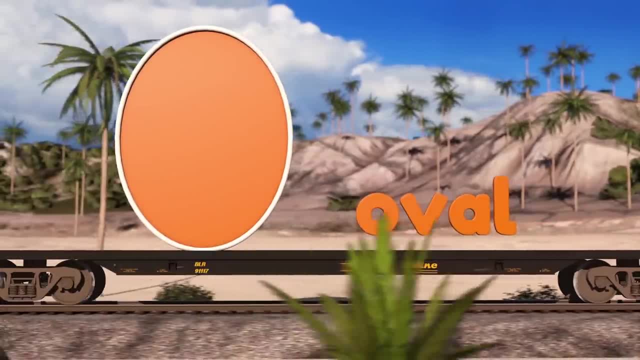 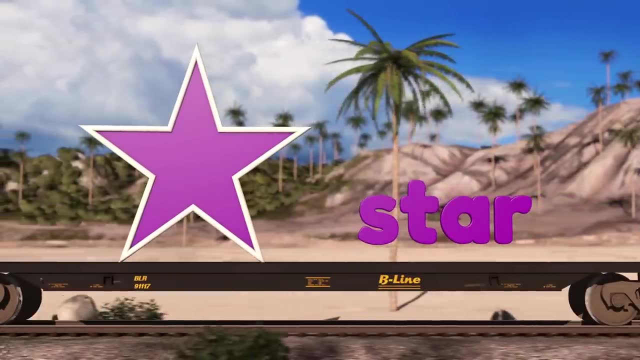 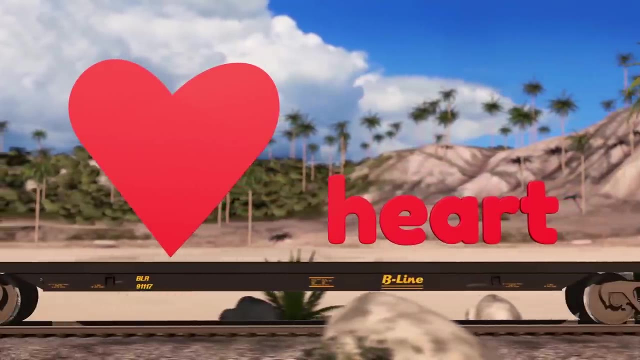 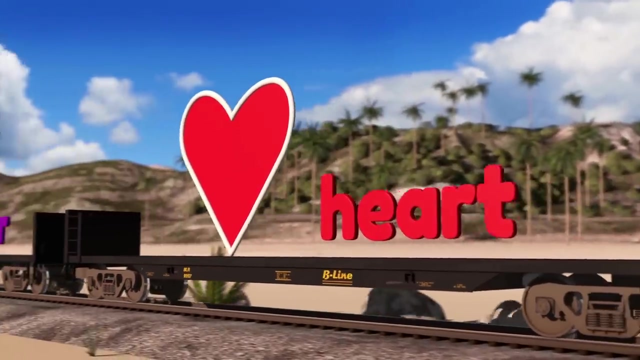 Next up is an oval. An oval looks like a circle but it's stretched. This shape is called a star. A star shape has five pointy arms And finally we have a heart. Heart is the symbol of love And we love learning about shapes. 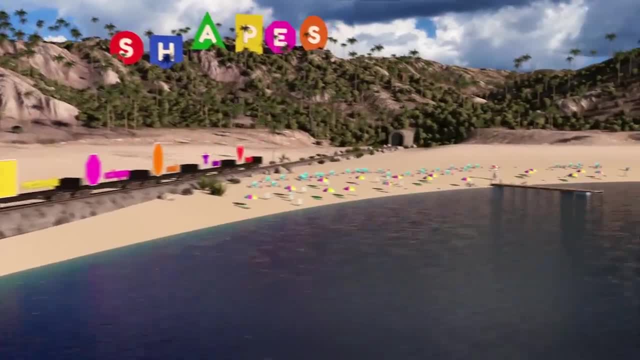 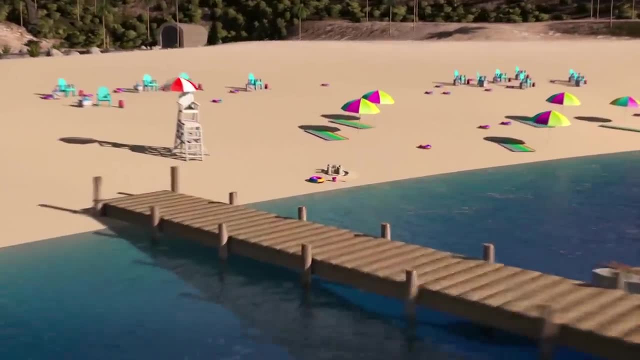 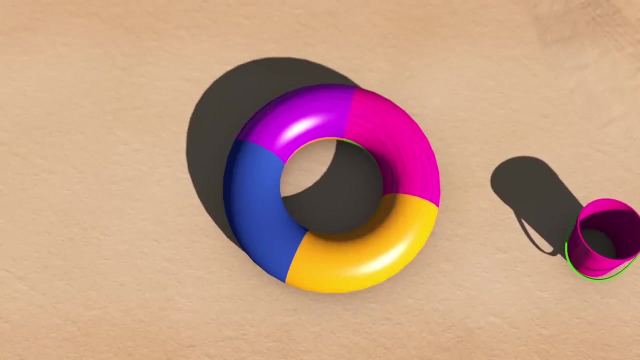 Hey, now that we've learned about some shapes, let's explore the beach to see if we can find those shapes in some fun objects. Can you spot a circle anywhere? I see one. That colorful swim tube is in the shape of a circle. 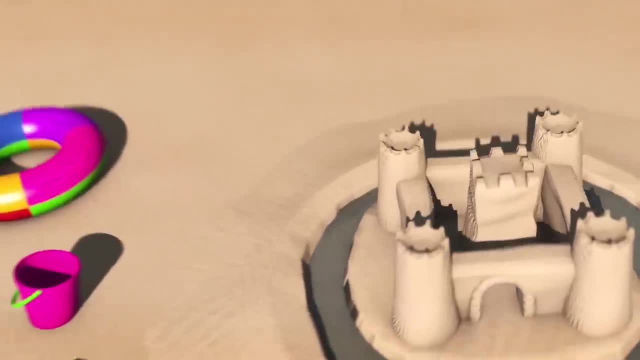 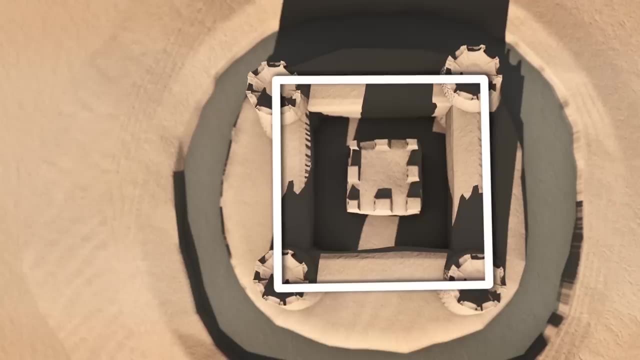 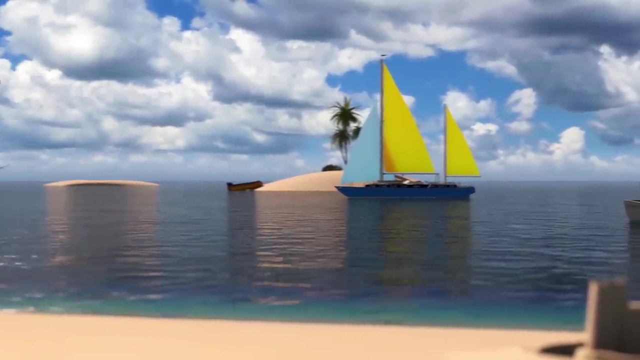 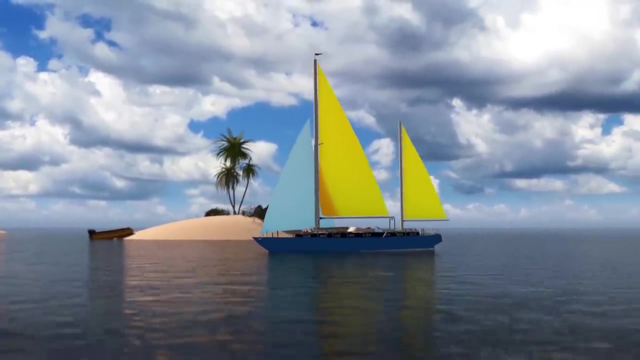 Let's see if we can find a square. Hmm, maybe the sand castle? Aha, The sand castle is in the shape of a square. Can you see any triangles? I wonder where we could find a triangle. Oh, look Over there at that sailboat. The sailboat's sails are triangles. 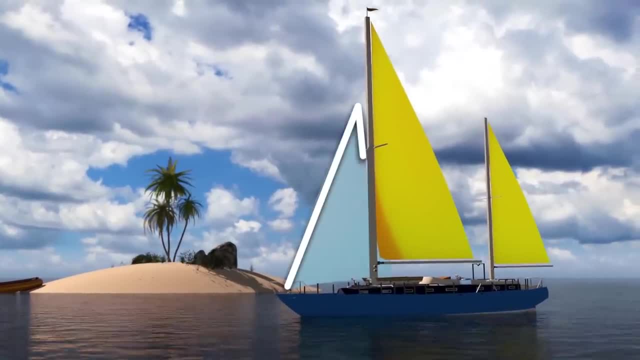 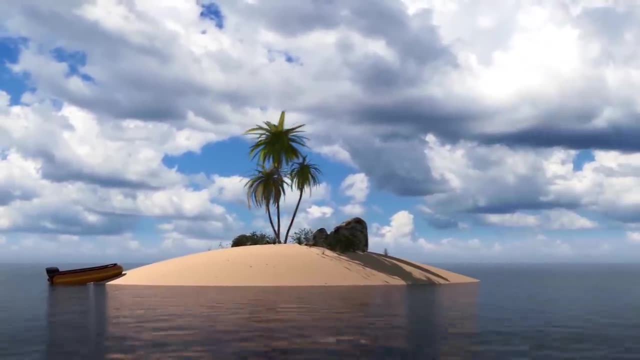 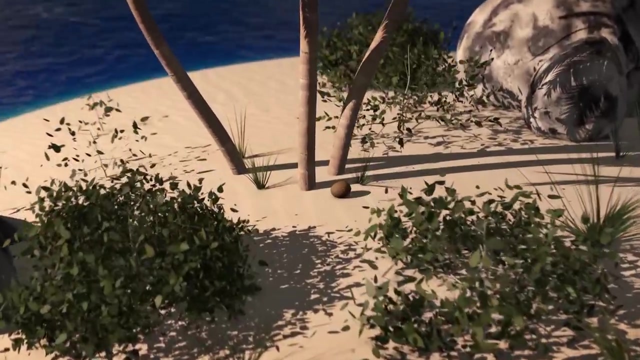 Here's one, two, three triangles. Why don't we check out that little island to see if we can find some more shapes? Hey, what are those things up in the tree? Oh, it's a coconut. It looks like a stretched circle. 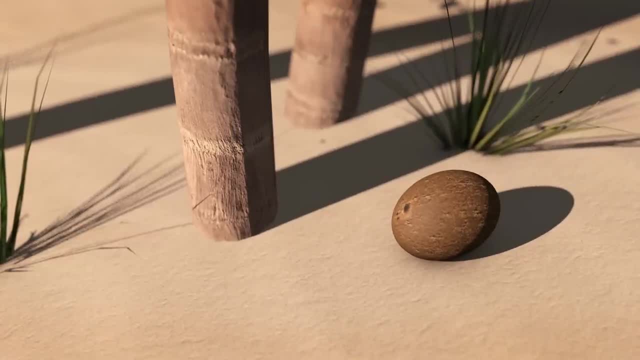 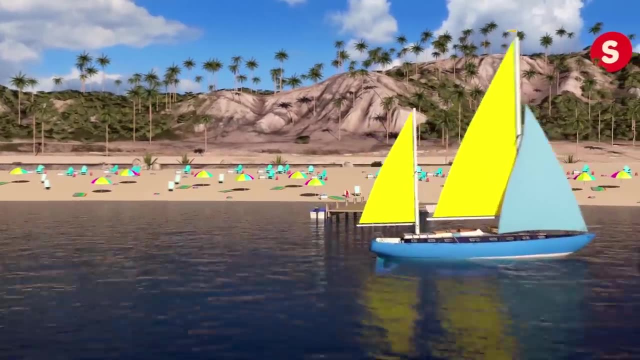 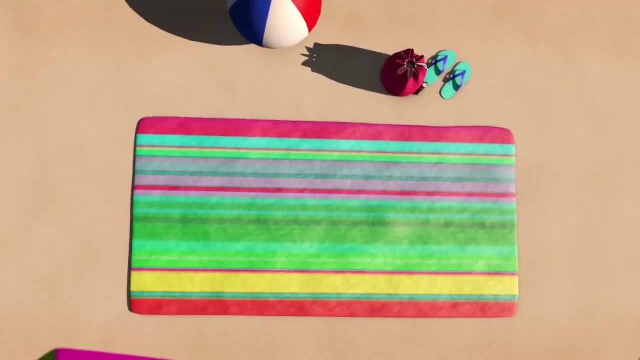 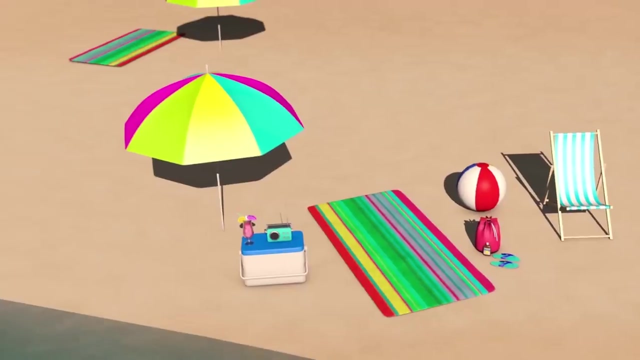 What's that shape called again? Oh yeah, that's right, It's an oval. Let's see if we can find a rectangle somewhere. Can you see any? There's one: The beach towel is in the shape of a rectangle. I wonder where we could find an octagon. 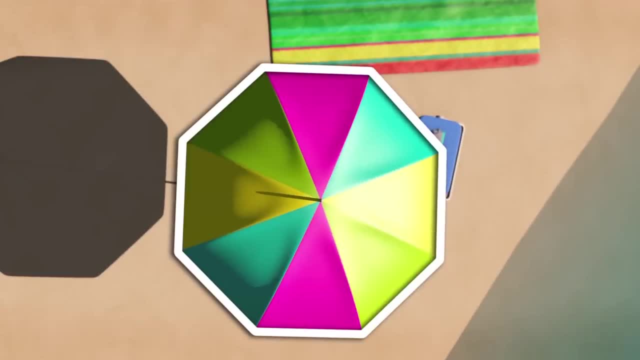 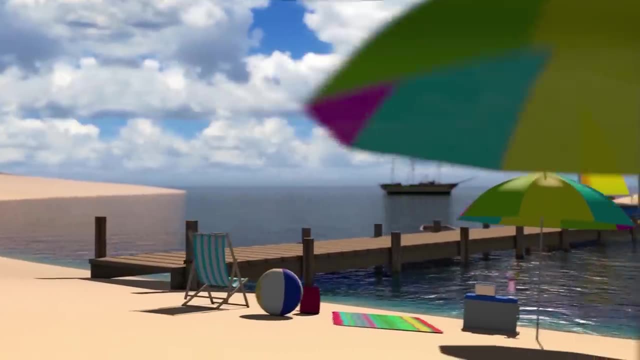 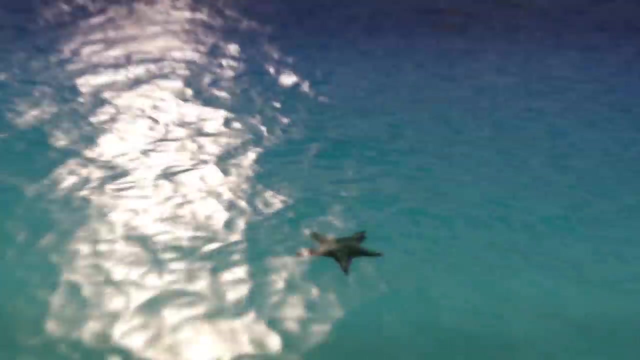 Aha, From above, this beach umbrella looks like an octagon with eight sides- Cool. I think I saw something in the water earlier that might be another shape. Let's try to find it. There it is, It's a starfish. 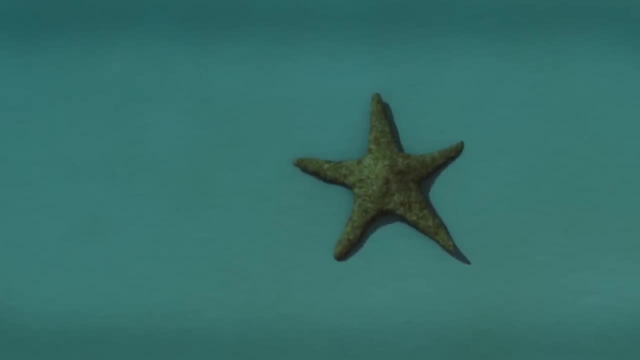 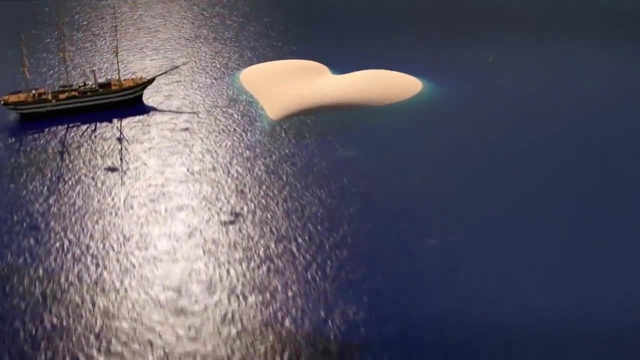 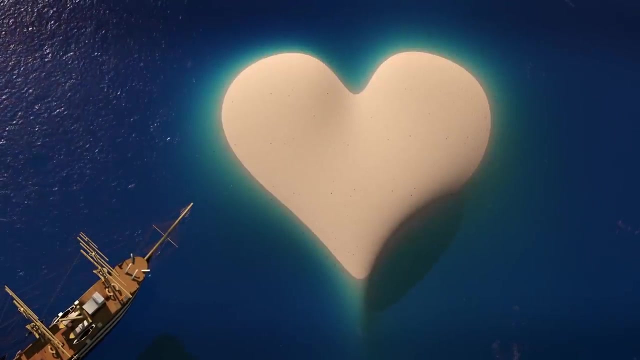 And a starfish is in the shape of a five-pointed star. Now all we have to find is a heart. Yeah, we found it. That little island is shaped just like a heart. Now we've found all of the shapes we learned about on the shapes train. 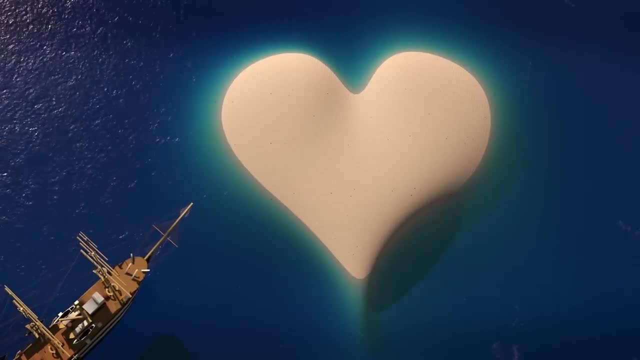 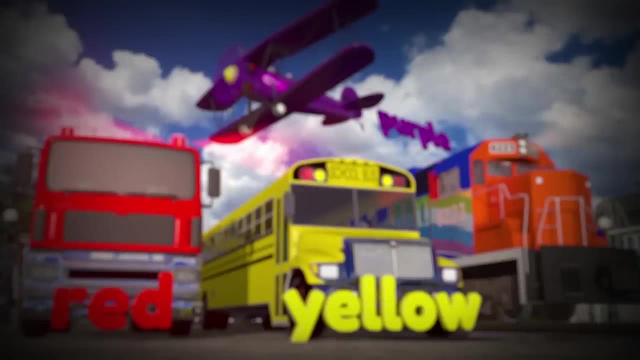 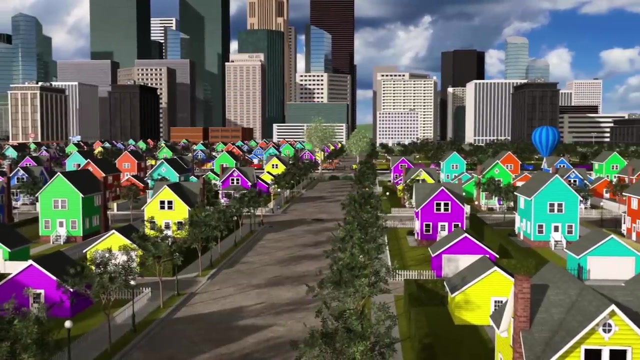 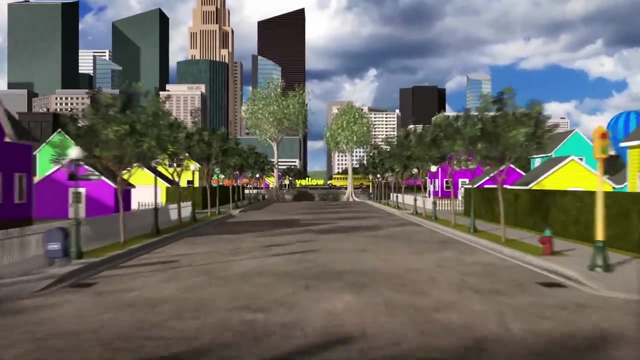 You did great. You're getting so smart. Thanks for watching Brainiacs and see you next time. Colour Train. Hey, Brainiacs, welcome to Colour Town. Colour Town is famous for all of its colourful houses. Hey, do you want to learn about some colours with me and Lizzy? 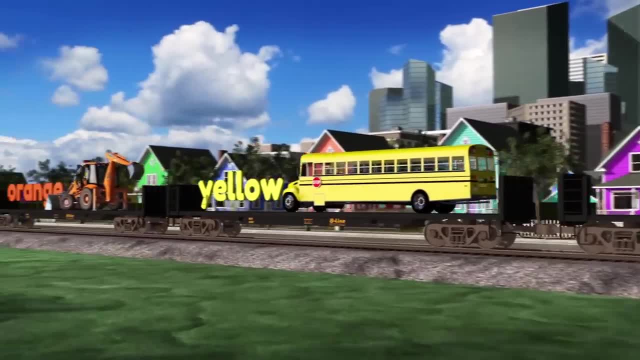 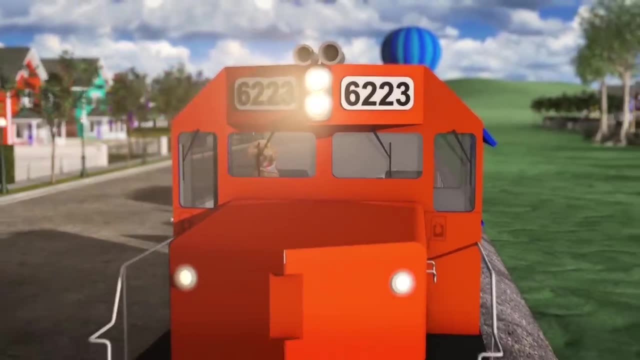 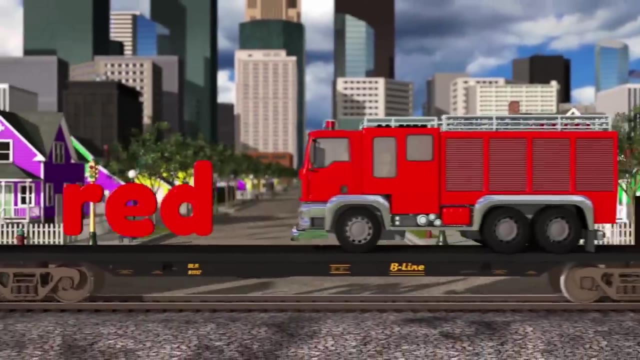 Look, Here comes Lizzy and the Colour Train and is carrying some cool stuff to help us learn, Hi, Lizzy. OK, let's go see what we have on the train. It's a red fire truck. The fire truck is red. 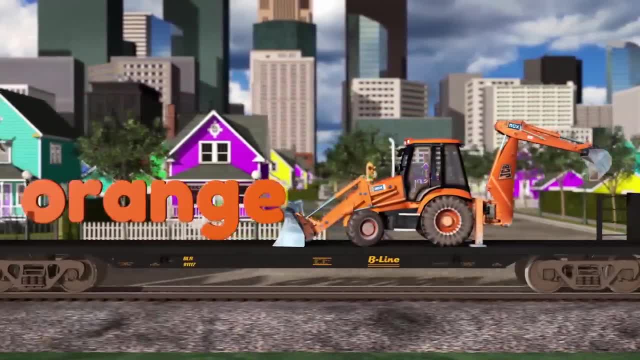 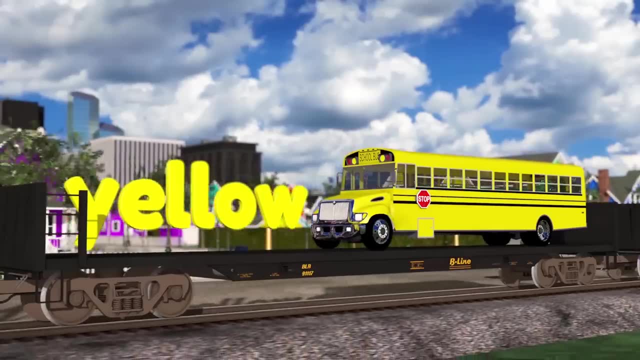 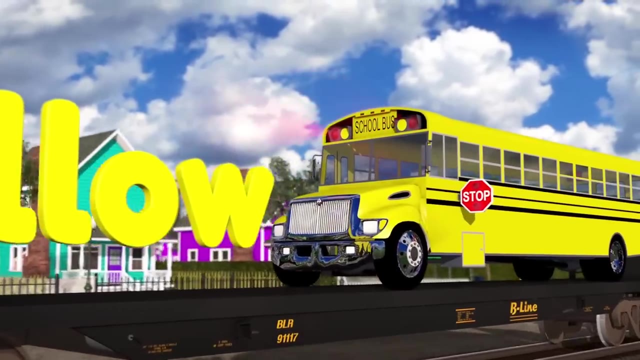 Red. Here is an orange backhoe. The backhoe is orange, Orange, Yellow. This is a yellow school bus. When you're ready to go to school, maybe you'll get to ride on a yellow school bus like this. A school bus is yellow. 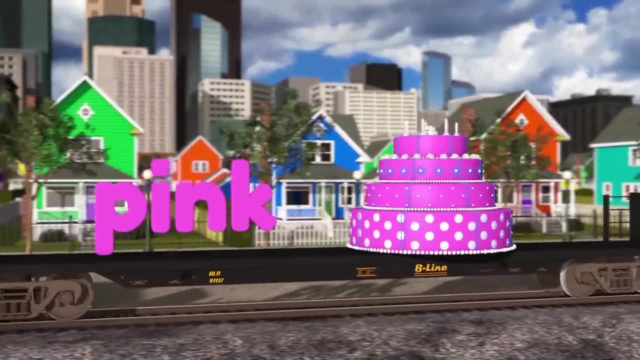 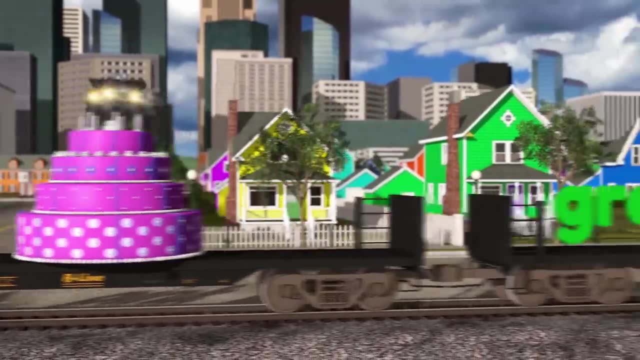 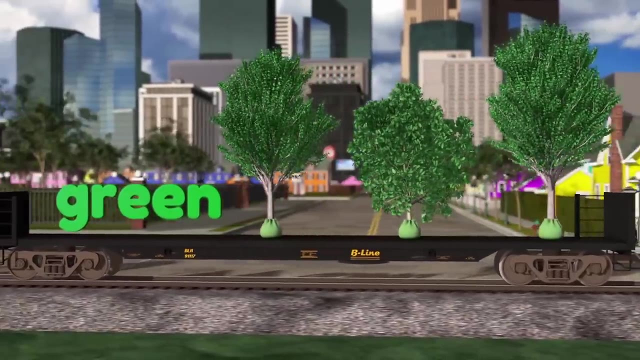 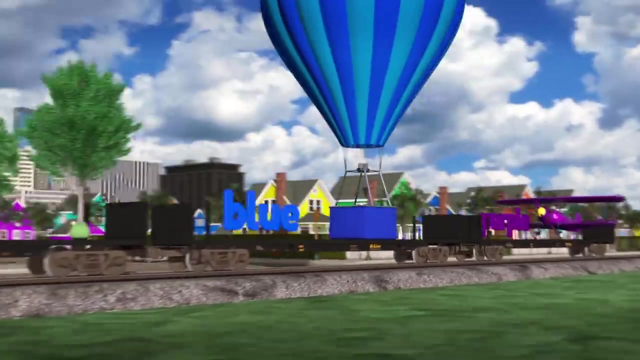 Pink. Whoa, That's a big pink birthday cake. The birthday cake is pink Green. Can you count how many green trees we have? The trees are green. Check out that blue hot air balloon. The hot air balloon is blue like the sky. 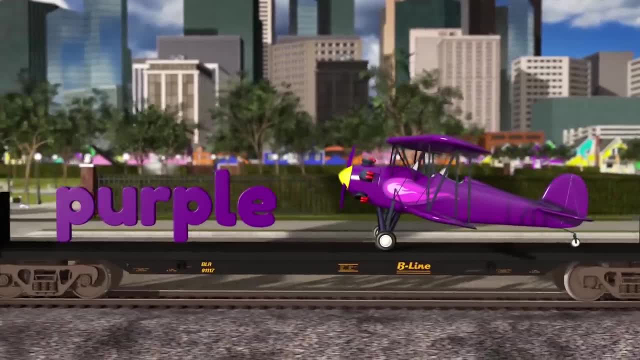 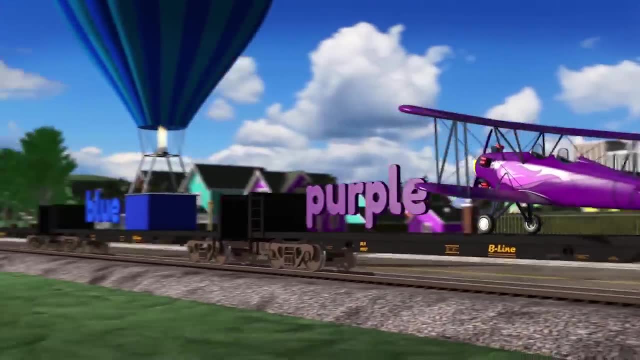 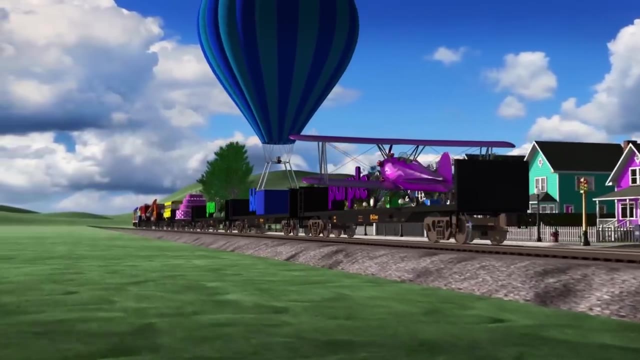 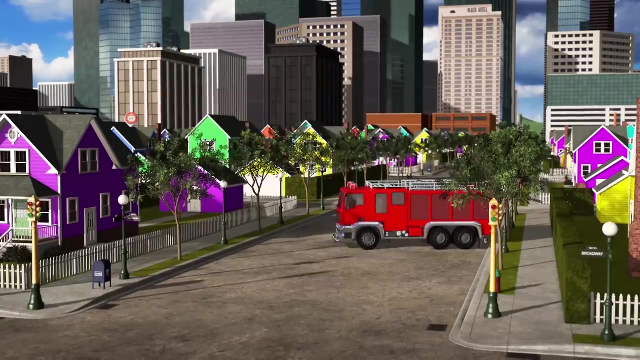 Blue Purple. This airplane is the colour purple. Wouldn't it be fun to fly up and away in this purple airplane? Alright, We've learned a whole bunch of colours. Let's see how many you can remember. What colour is the fire truck? 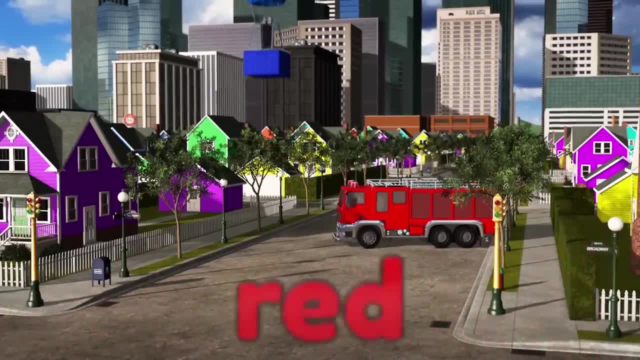 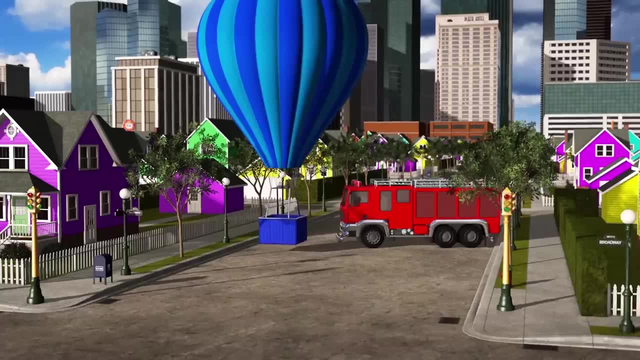 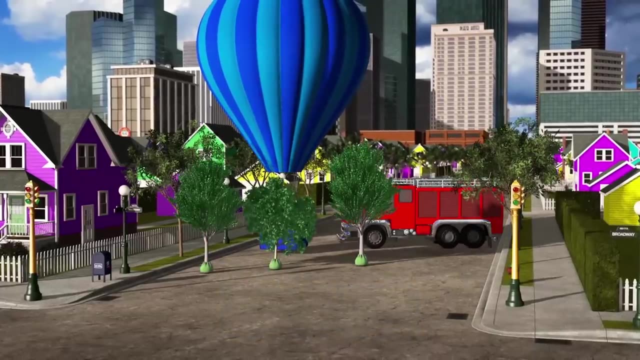 That's right, The fire truck is red. What colour is the hot air balloon? It's the same colour as the sky. Yes, It's the colour blue. Do you remember what colour the trees are? Right on, The trees are green. 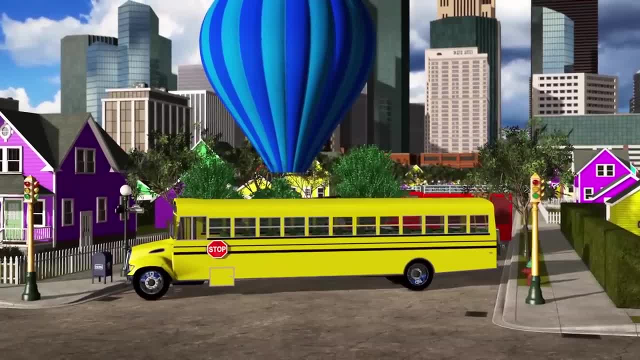 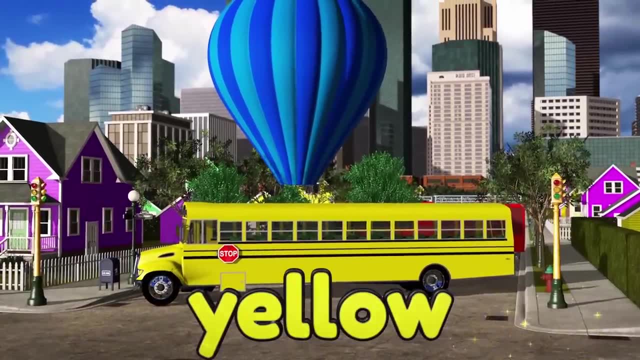 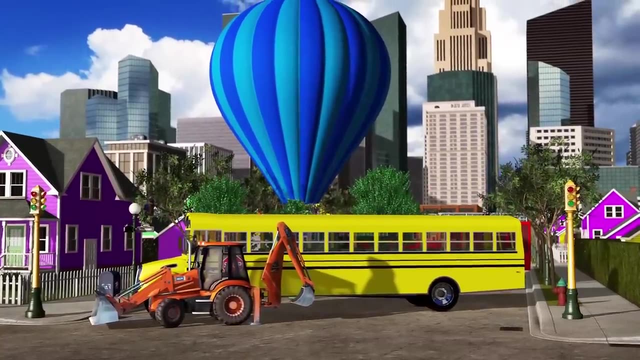 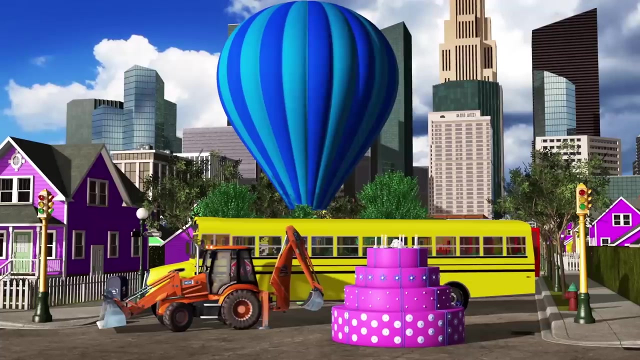 What colour is this school bus? Good job, The school bus is yellow. What colour was that backhoe again? Oh yeah, The backhoe is orange. There's the yummy birthday cake. Can you guess what colour it is? Perfect, The cake is pink. 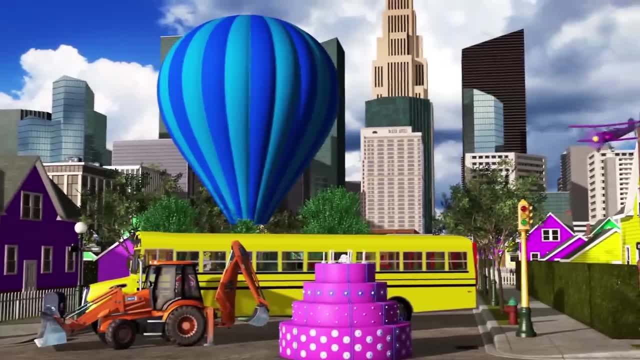 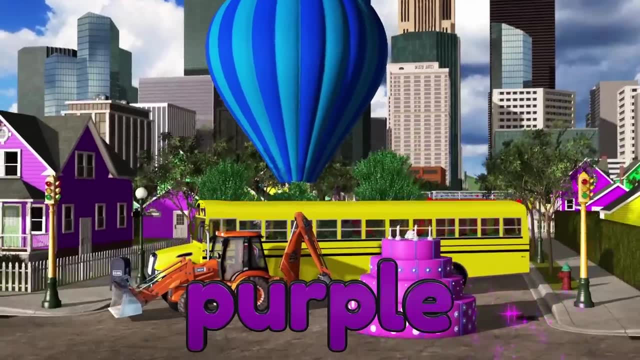 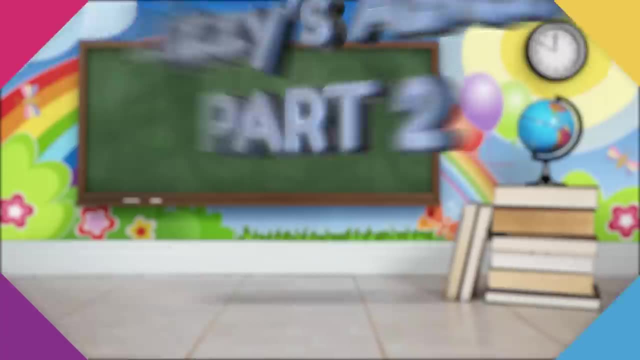 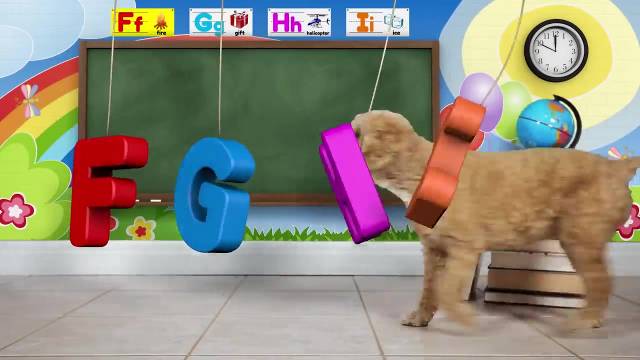 Now, where is that airplane? Here it comes, And what colour is the airplane? The airplane is purple, Right on. Thanks for learning colours with us. I hope you had a lot of fun. Hey, Brainiacs, It's time to learn more of the alphabet with Lizzy. 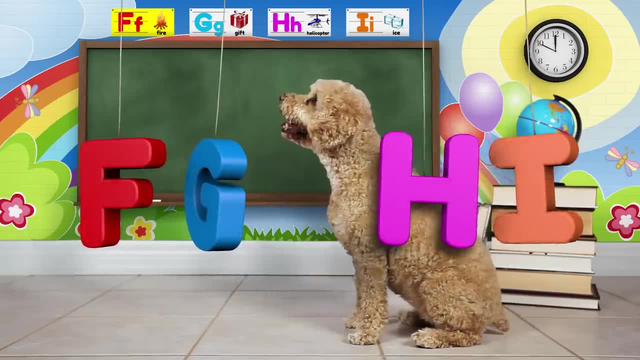 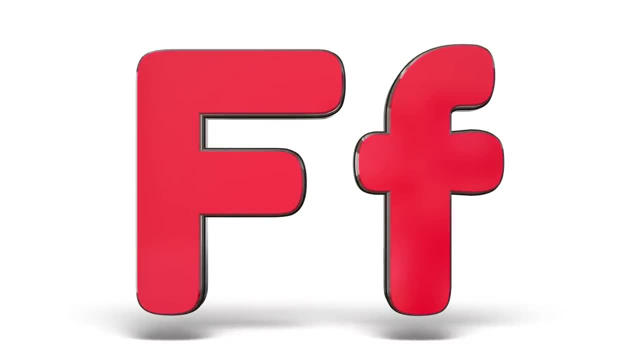 Today we're going to learn about the letters F, G, H and I, G, H and I. Alright, let's go. First up is a letter F and it looks like this: This is a capital F. This is a lowercase f. 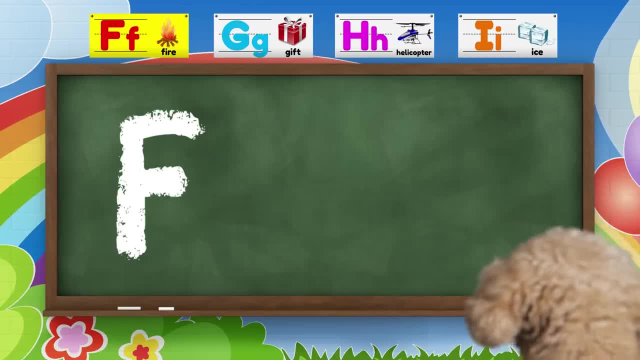 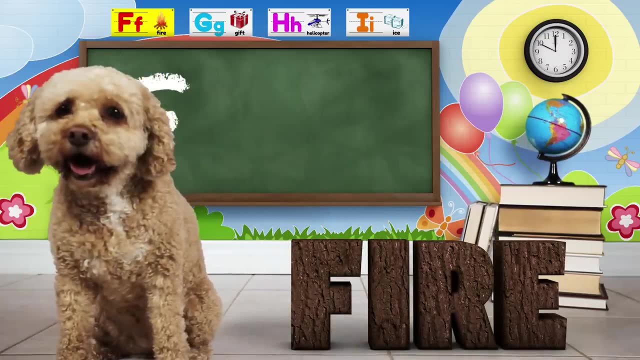 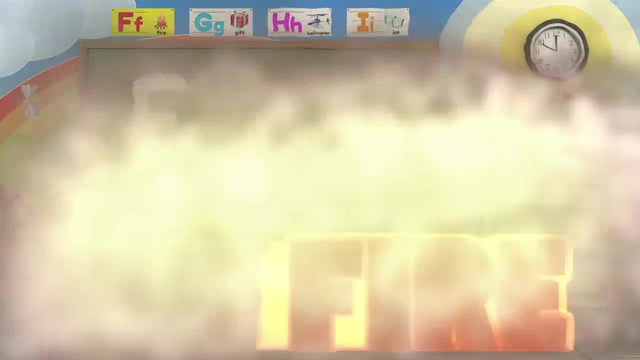 The letter F sounds like fuh fuh. One word that starts with F is fire. Be careful, Lizzy Fire is very dangerous and very hot. We'd better put this fire out. Another word that starts with F is fast. 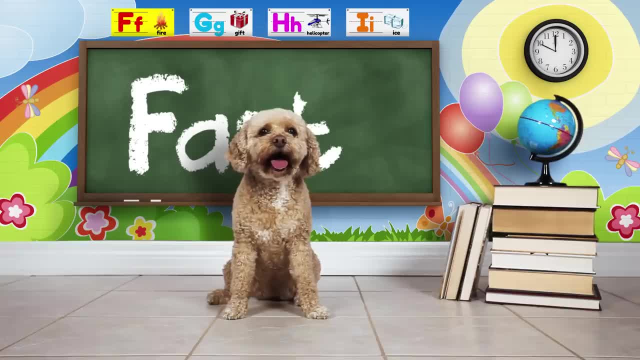 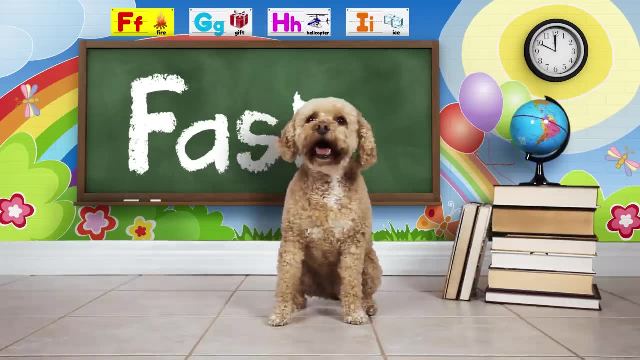 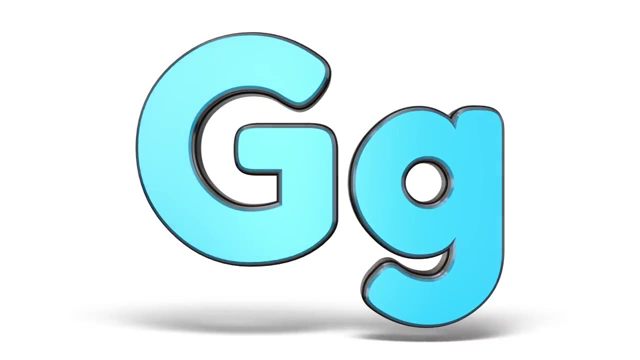 Lizzy can run very fast. Want to see how fast she can go. Whoa, that sure was fast. That was awesome. The next letter we have is the letter G and it looks like this G sounds like guh guh. 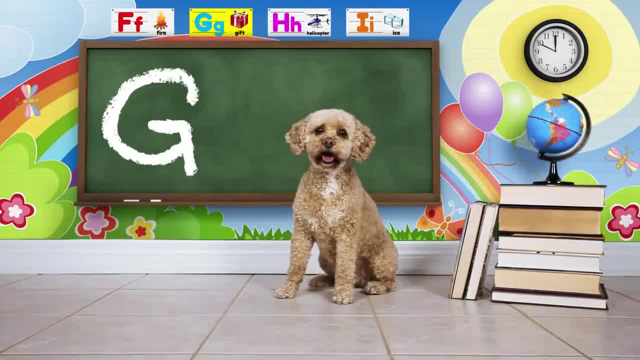 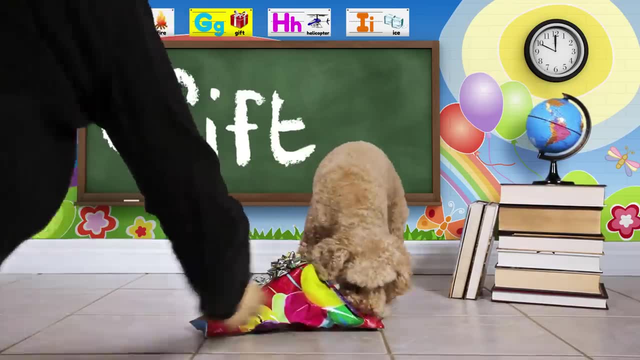 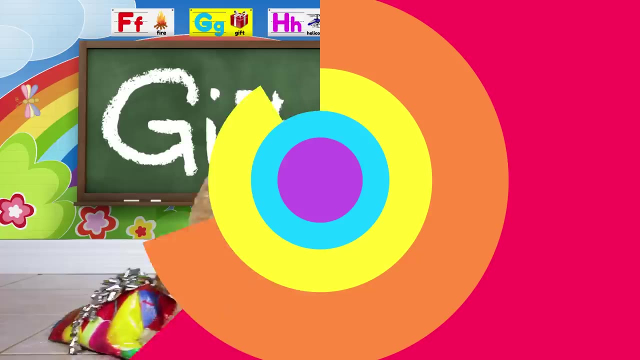 The word gift starts with the letter G. Do you like opening gifts? Lizzy sure does. Here you go, Lizzy. I wonder what's inside. Go on, open it up, Lizzy. It's a stuffed bear. Lizzy's going to have so much fun with this gift. 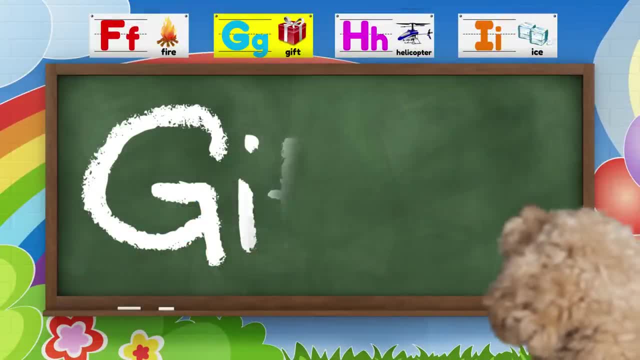 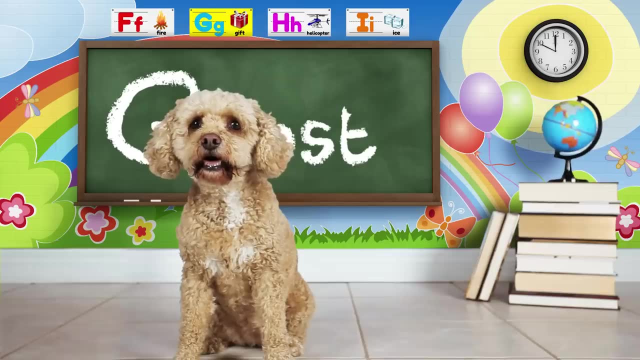 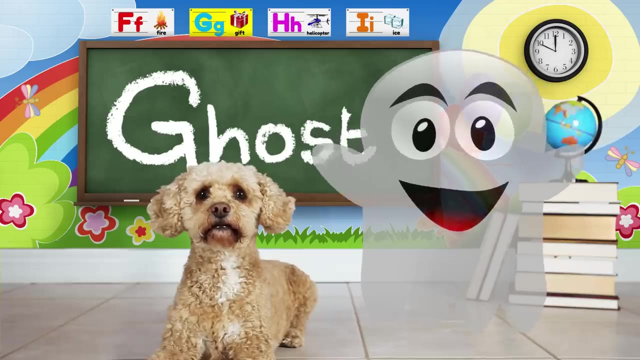 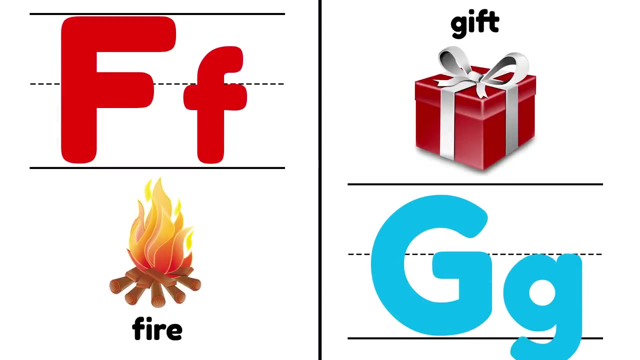 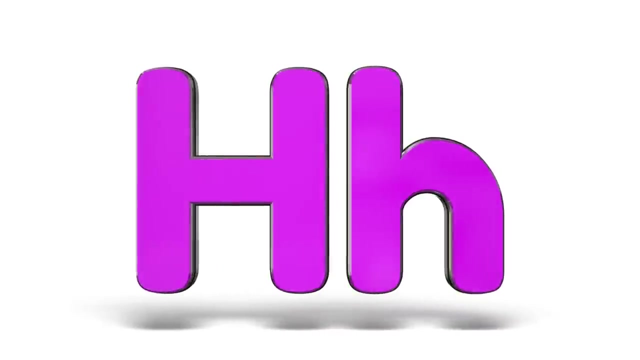 Another word that starts with G is ghost. Look, here comes a friendly ghost. now Go get the ghost. Lizzy Fuh fuh- F for fire. Guh guh- G for gift. The next letter of the alphabet is H, and it looks like this: 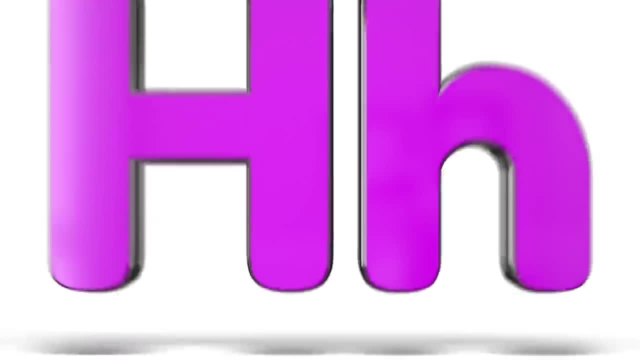 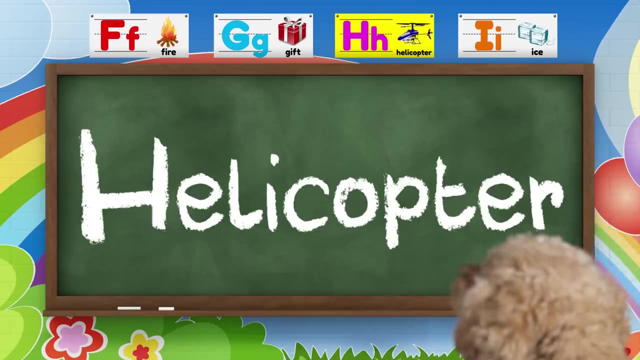 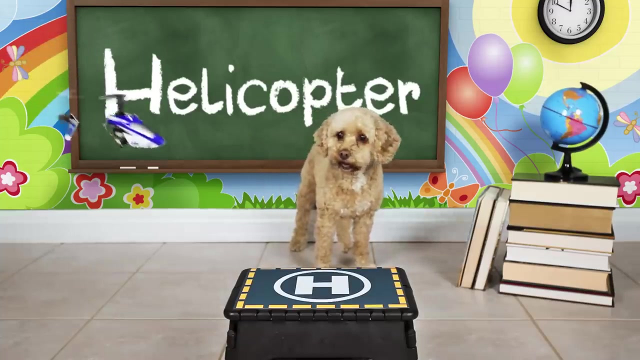 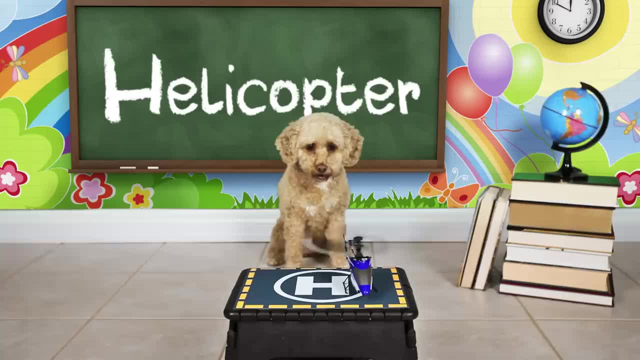 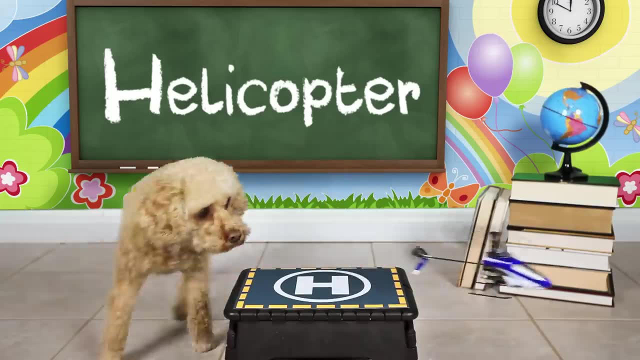 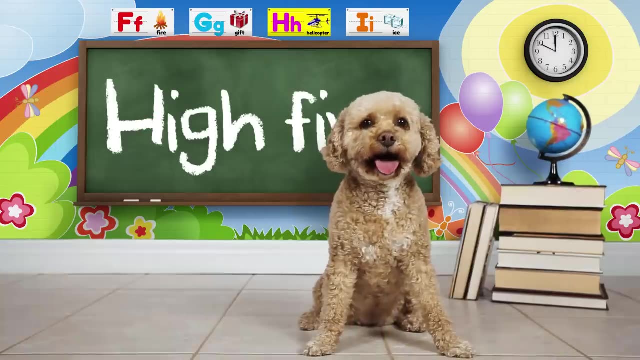 Let's try again. Let's try again, Let's try again. Yeah, touchdown, Uh oh, I think Lizzy has her eye on our helicopter. That's not a dog toy, Lizzy. Lizzy's been doing a great job so far. 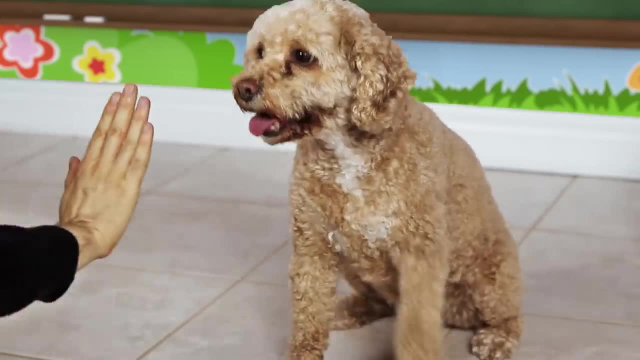 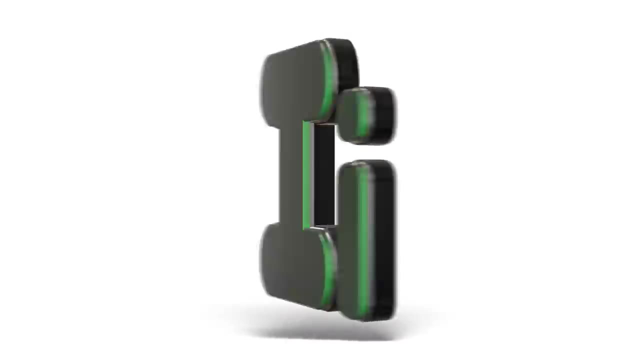 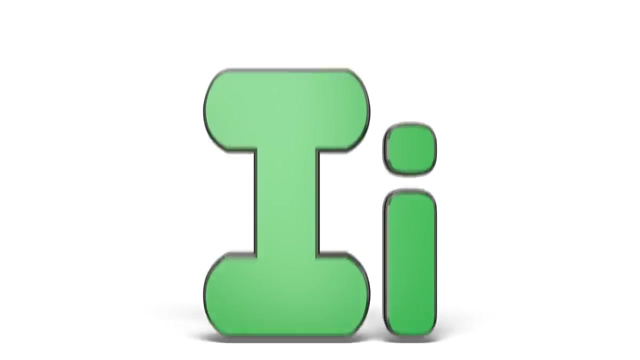 She deserves a high five, High five, Good job. High five starts with the letter H. Next up is the letter I and it looks like this. The letter I sounds like IH or I. Do you know what happens when water gets really cold? 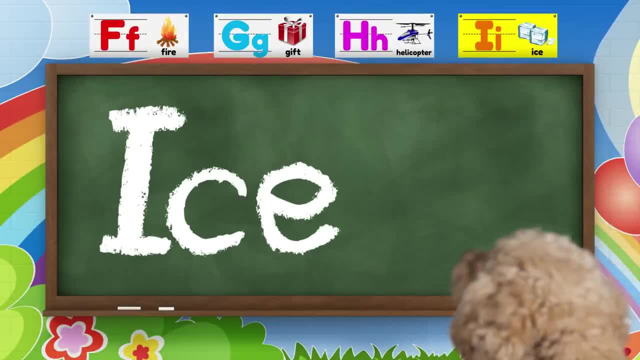 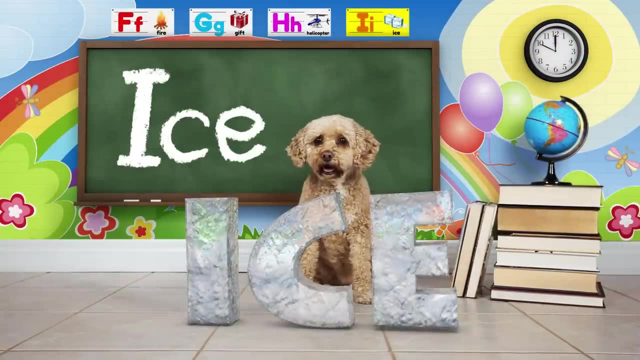 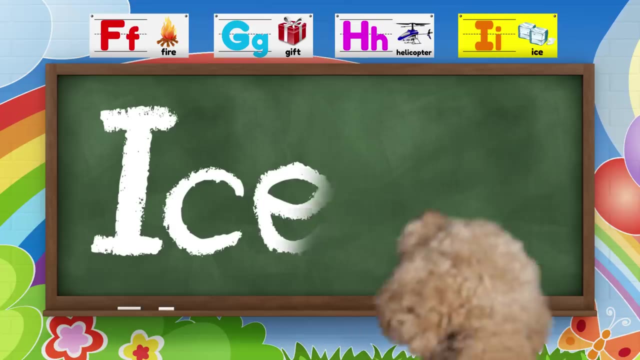 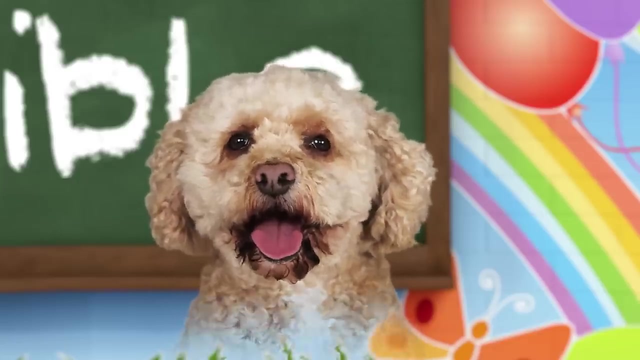 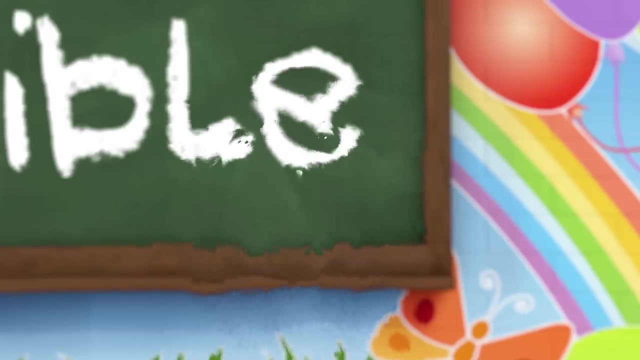 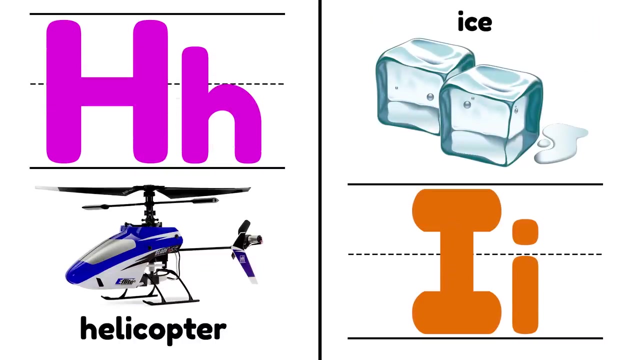 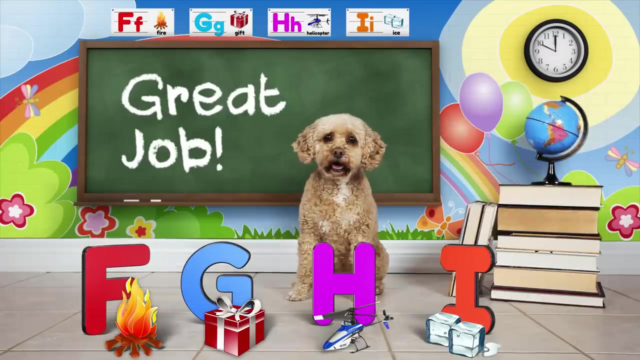 It turns to ice, and ice starts with the letter I Look out below. Another word that starts with I is Invisible. Hey, Lizzy, where did you go? Oh, no, She's invisible. H, H, H for helicopter, I, I, I for ice. great job everyone. I hope you had fun learning with Lizzy again. let's. 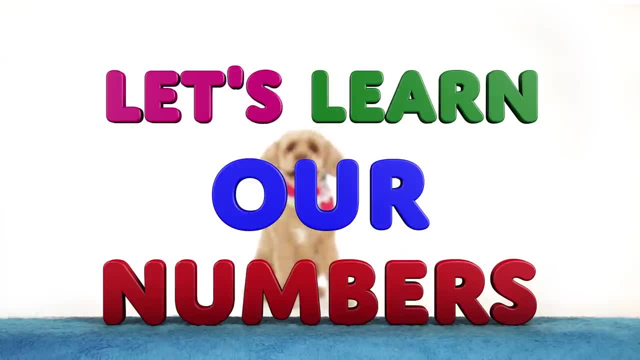 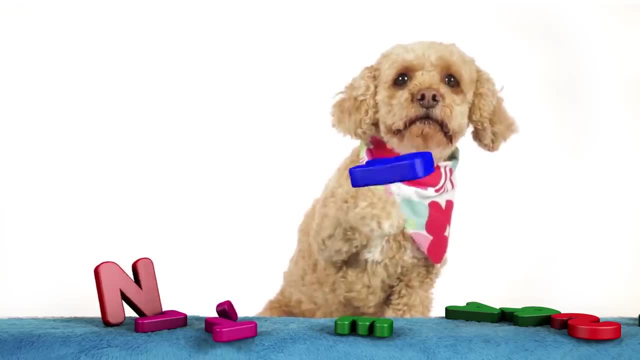 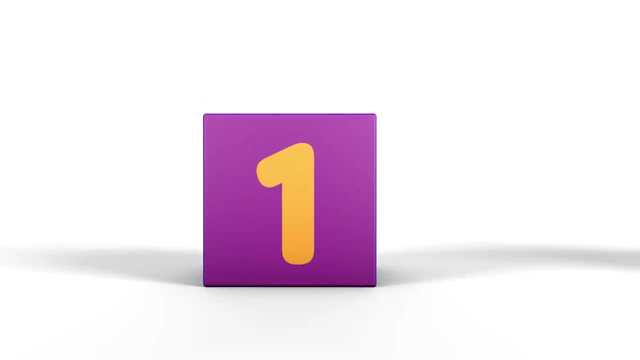 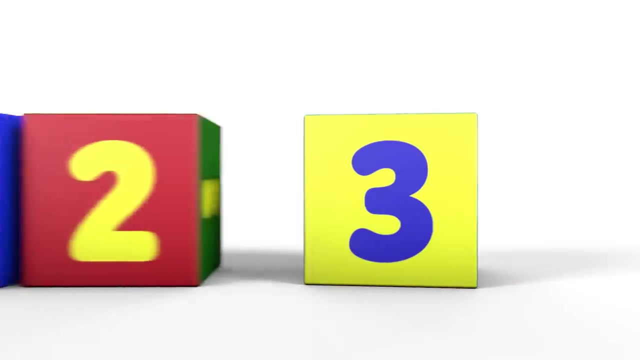 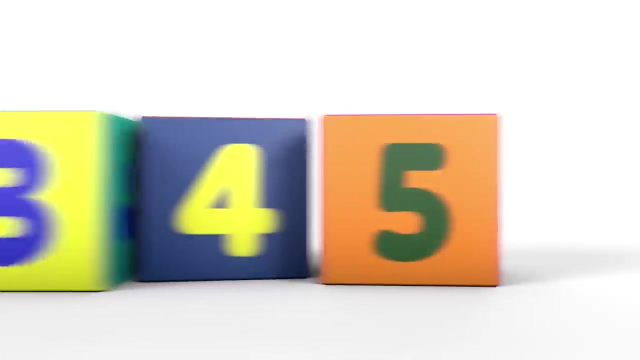 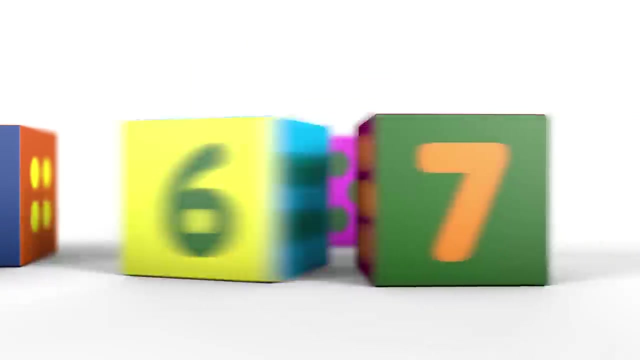 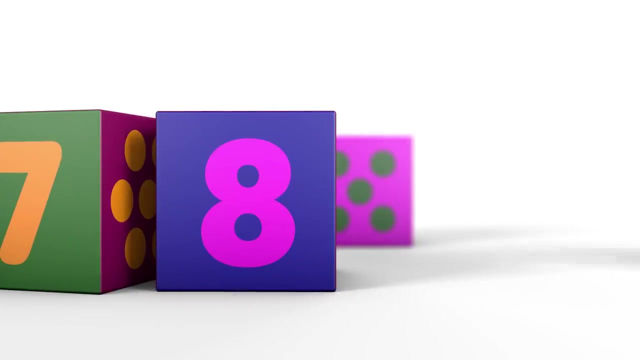 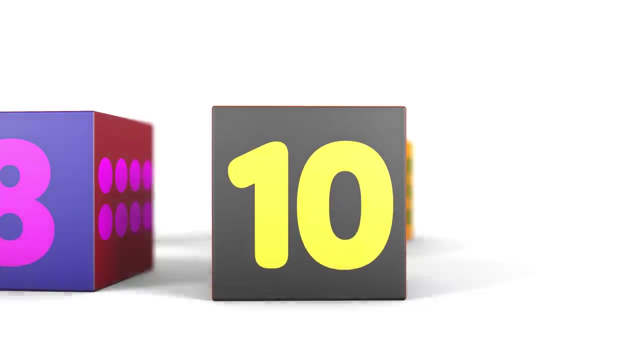 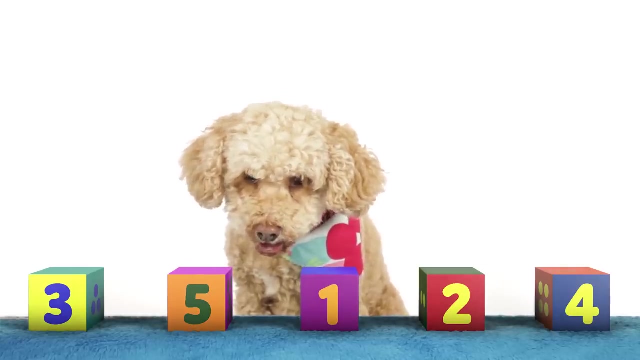 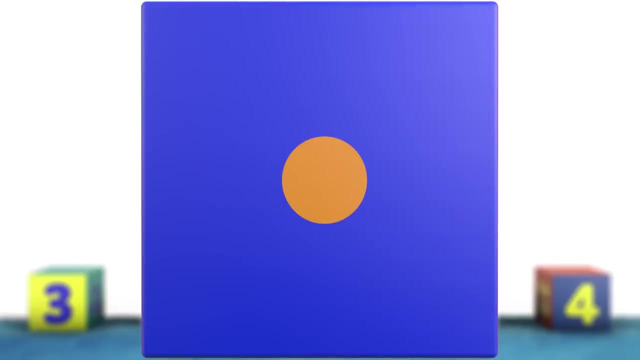 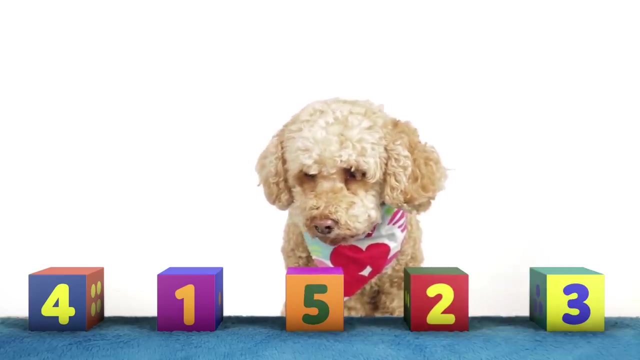 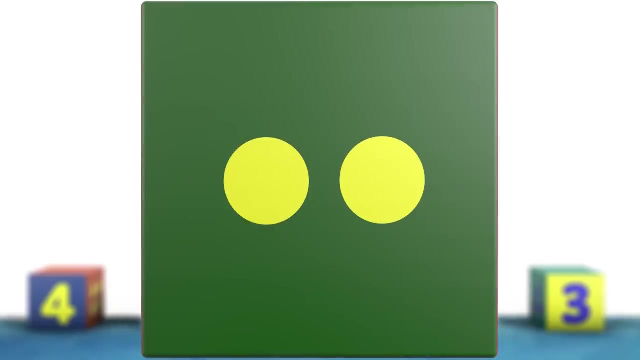 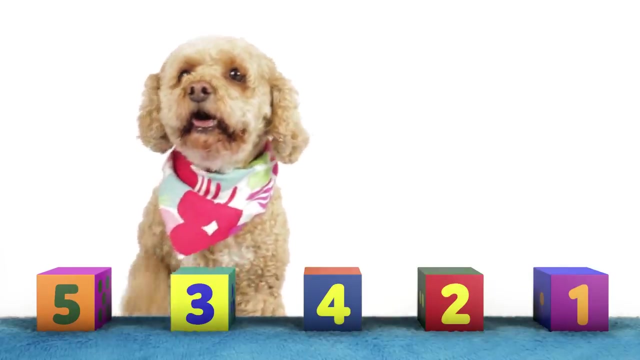 learn our numbers one, two, three, four, three, four, Five, six, seven, eight, nine and ten. OK, Lizzy, where's the number one? That's right. Where's the number two? Two, Can you find number three, Two? 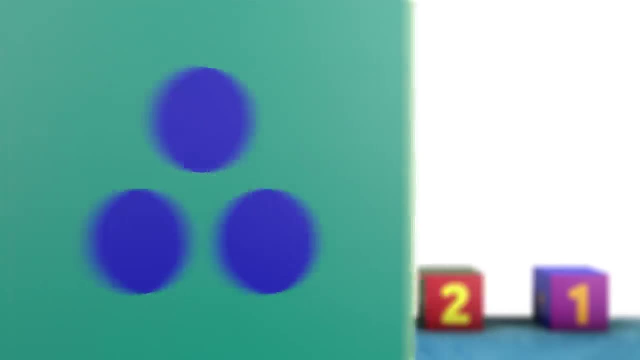 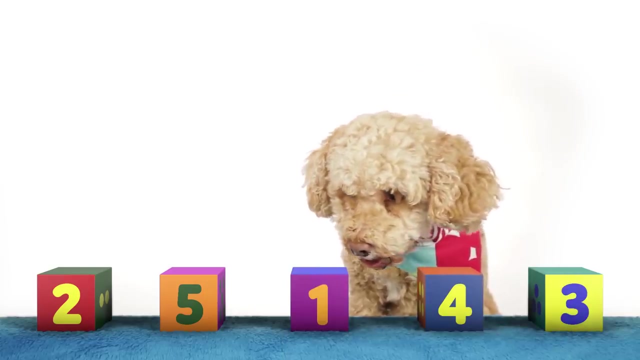 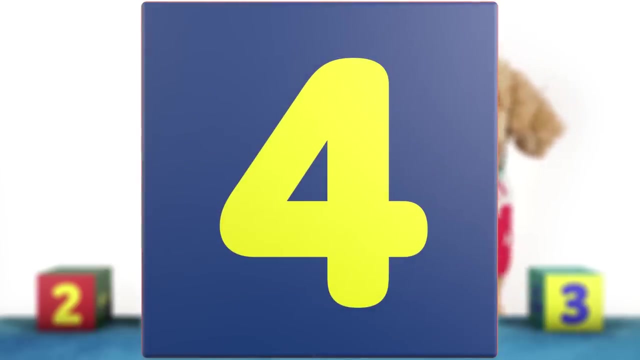 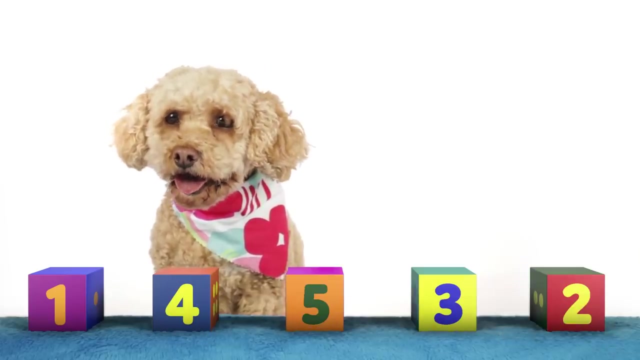 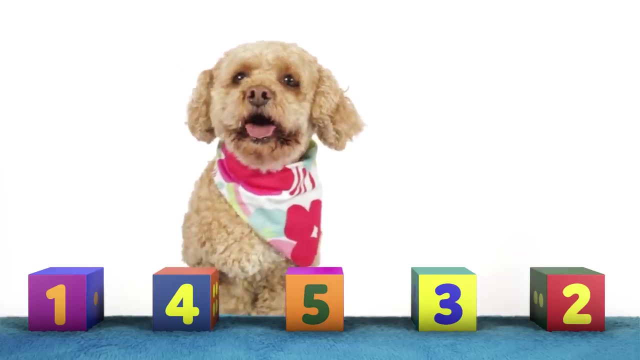 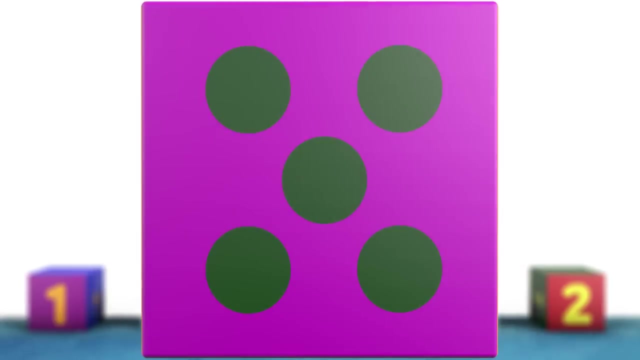 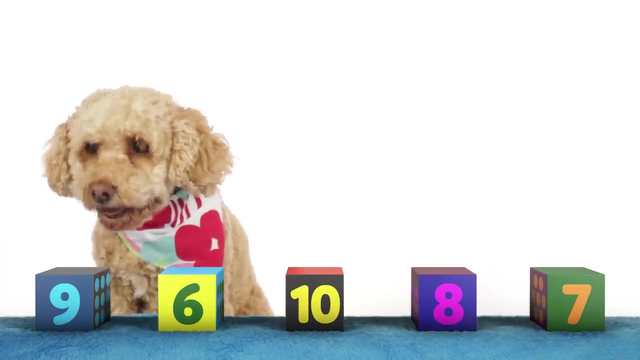 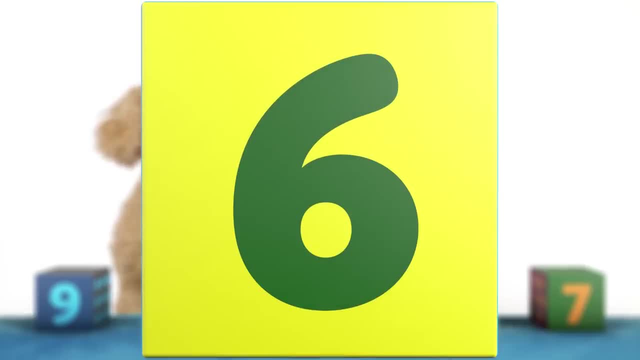 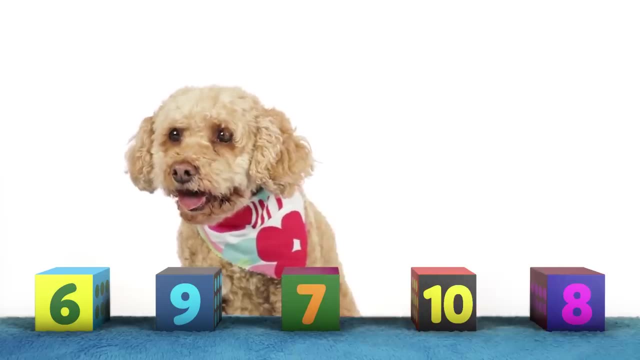 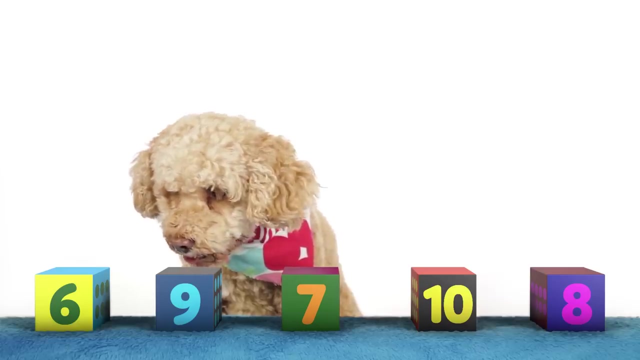 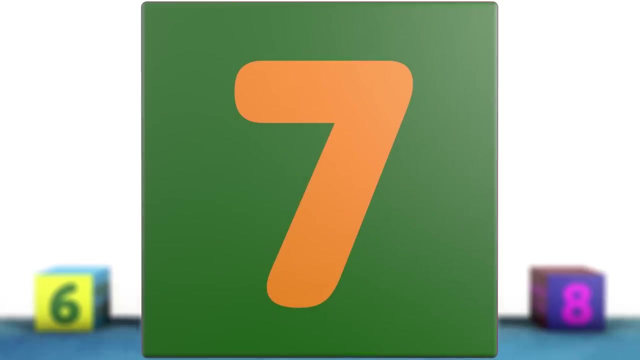 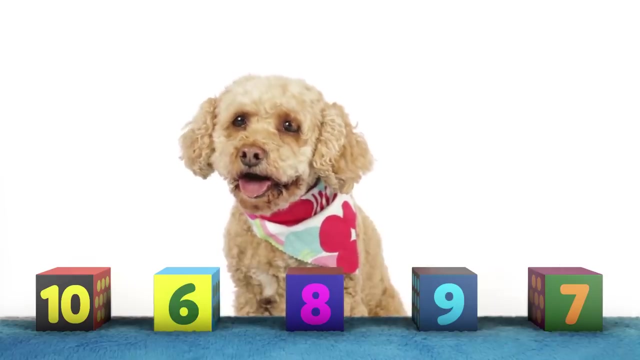 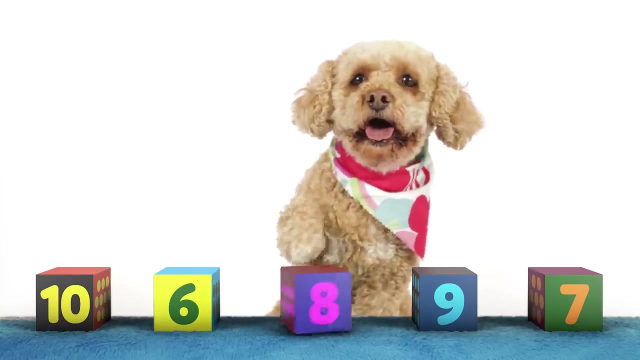 I found it: Six. What about the number seven? Six, No way. What about the number seven? What about the number seven? Perfect, I found it. I found it. OK, Lizzy, Great job, Great job, The eight. 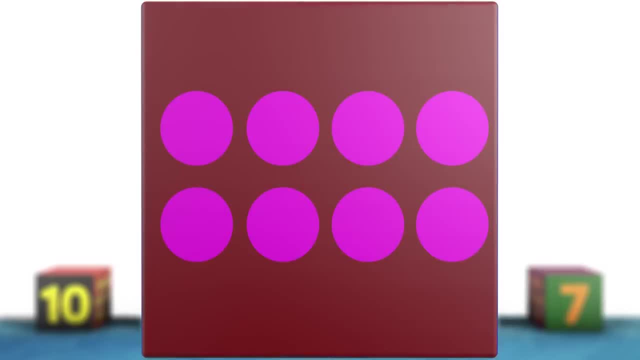 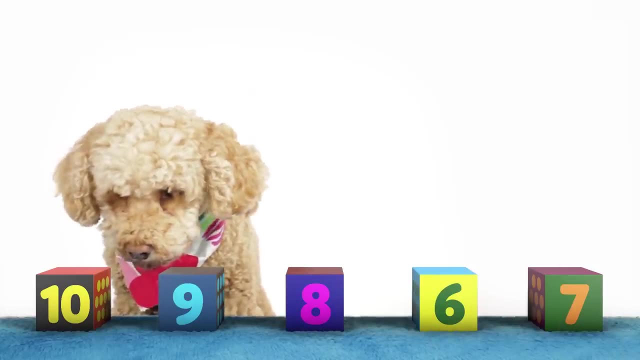 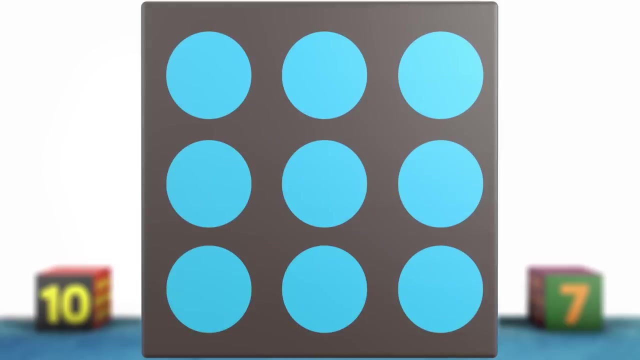 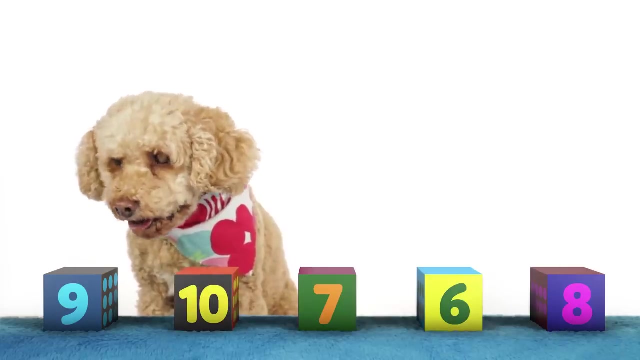 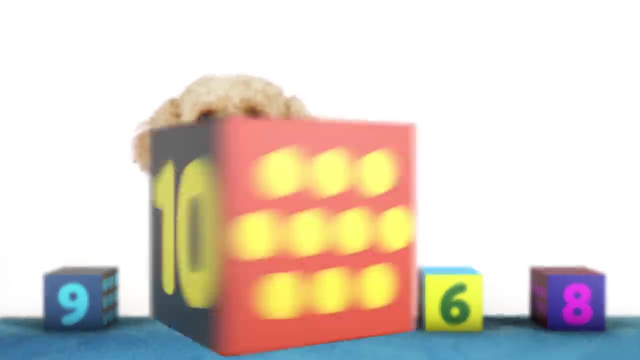 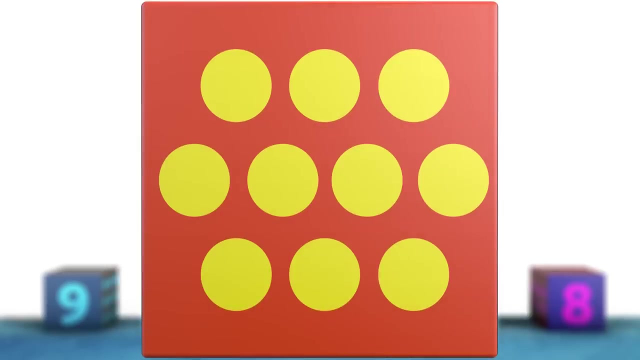 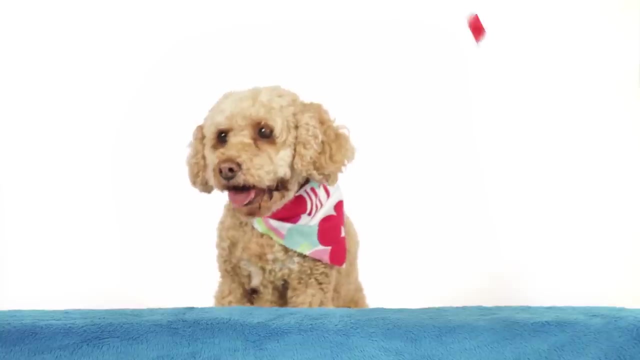 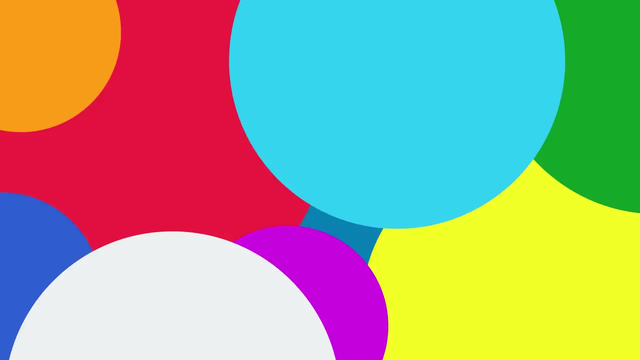 You're doing great. Show me number nine. That's right, nine. You're doing so well, but can you find number ten? Way to go. That was amazing High five. Say goodbye, Lizzy Number Train. Hey, Brainiacs, check it out. 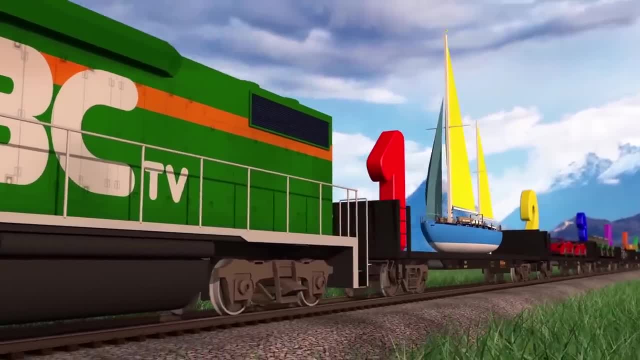 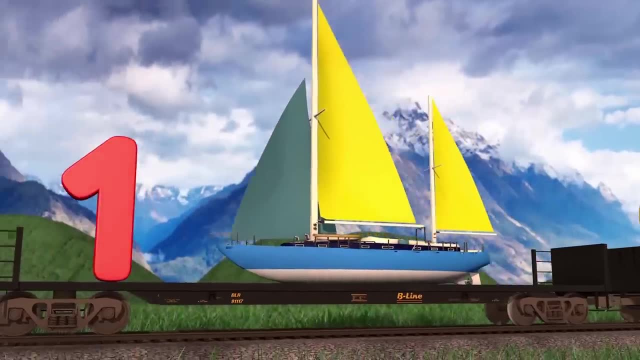 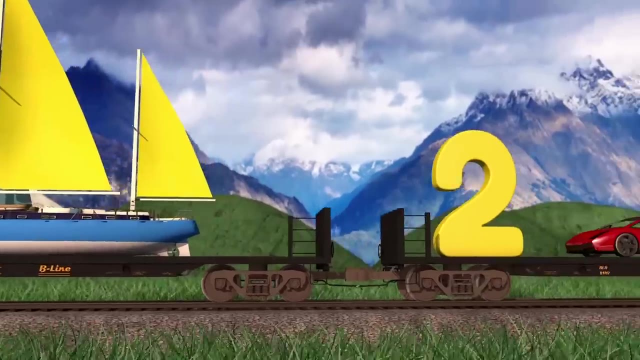 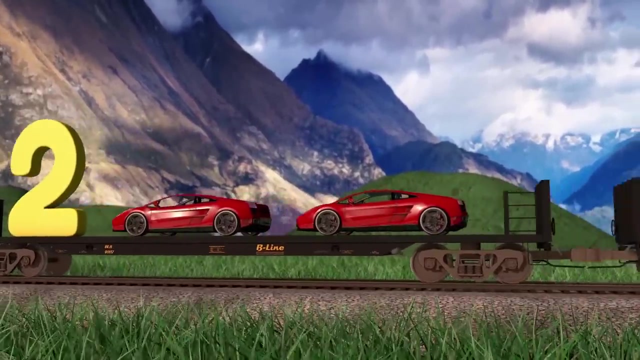 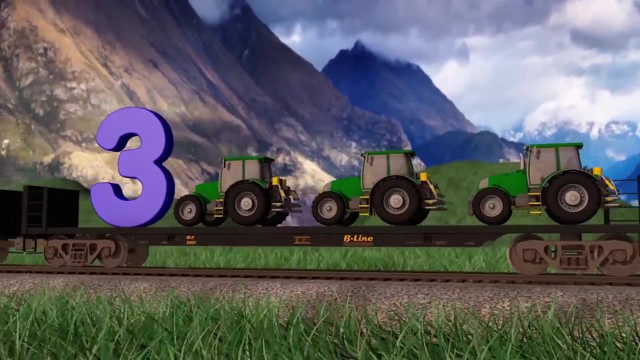 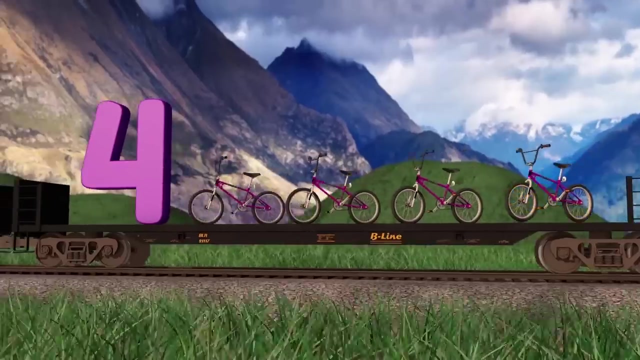 Here comes the numbers: train. Let's read the numbers and see if we can count all the objects on the train: One: One sailboat Two: One two sports cars Three: One two, three tractors. Four: One two, three, four bicycles. 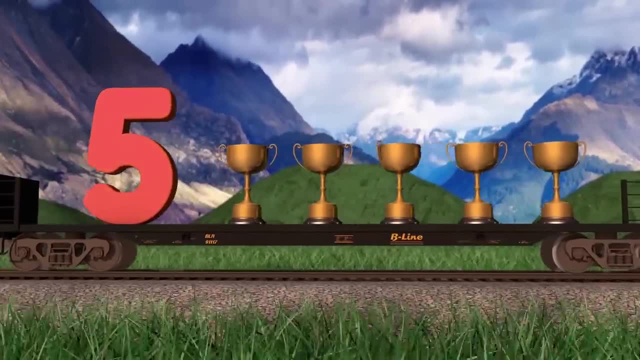 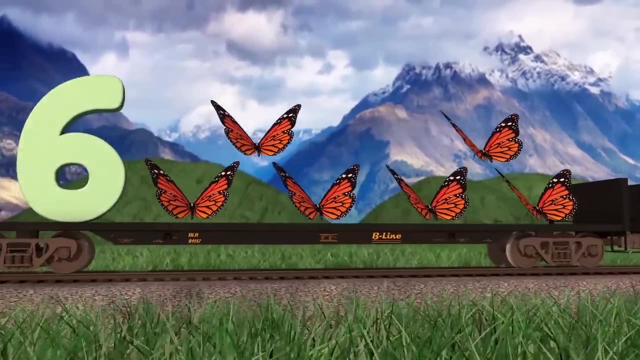 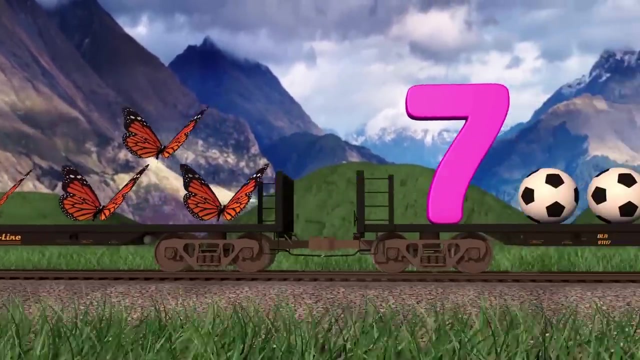 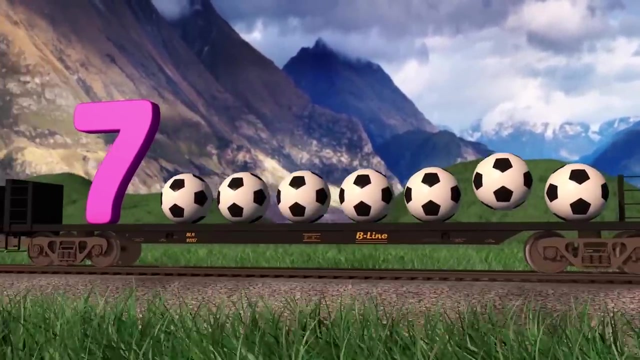 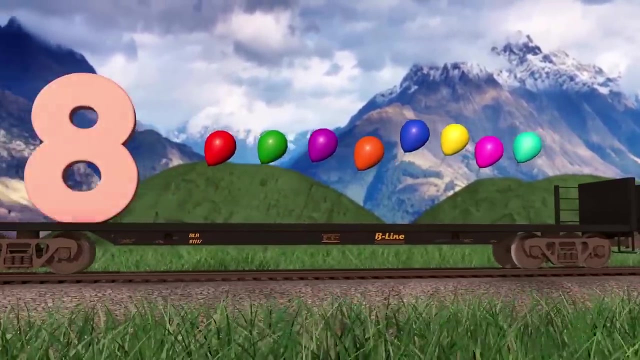 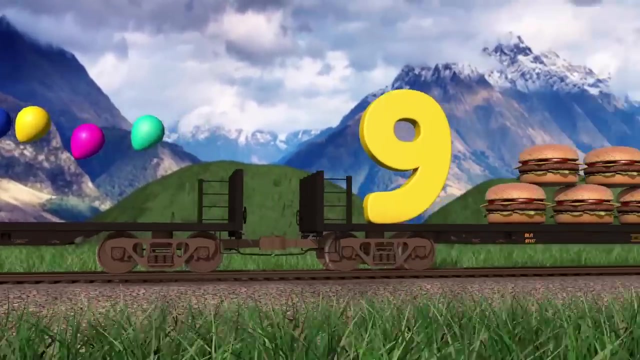 Five, One, two, three, four, five. trophies: Six: One, two, three, four, five, six butterflies: Seven: One, two, three, four, five, six, seven soccer balls: Eight One, two, three, four, five, six, seven, eight balloons: 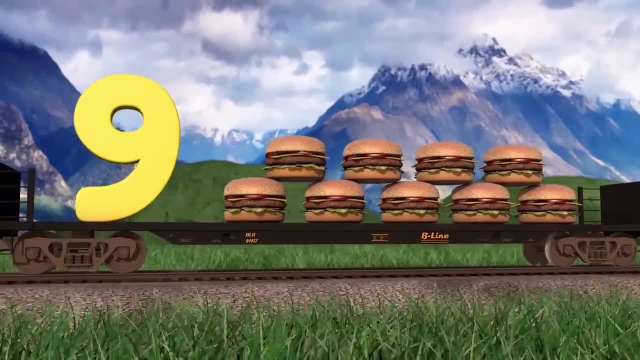 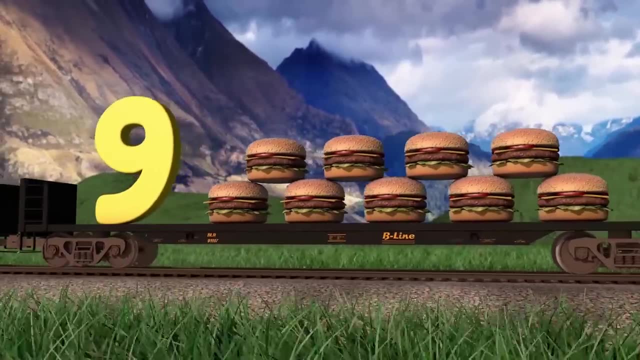 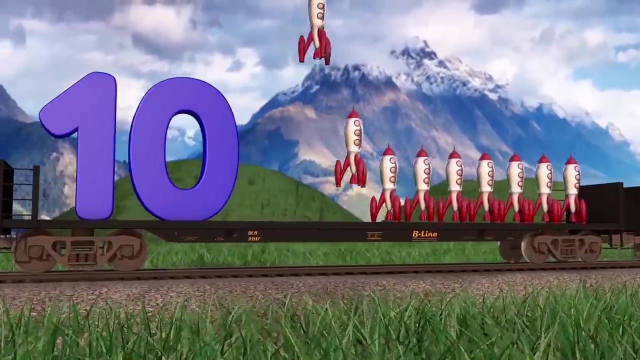 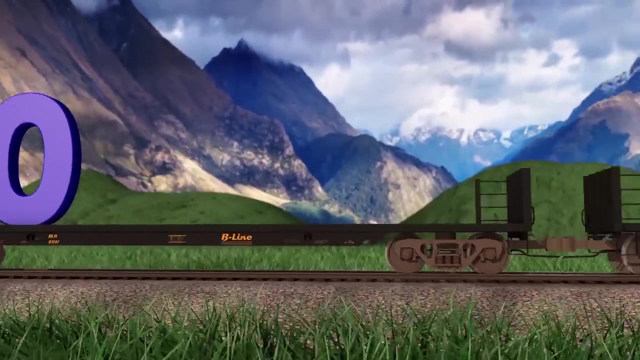 Nine. One, two, three, four, five, six, seven, eight, nine hamburgers. Ten One, two, three, four, five, six, seven, eight, nine, ten rockets, Great job. Now let's count up to twenty. 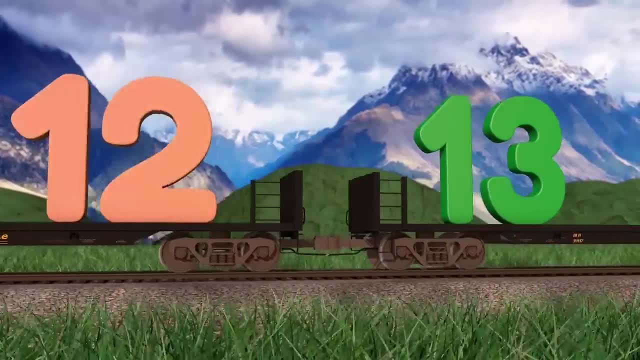 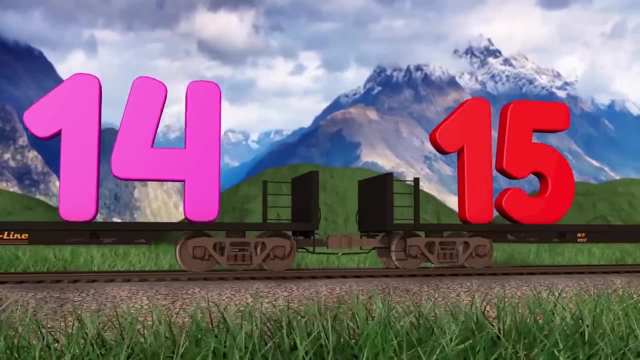 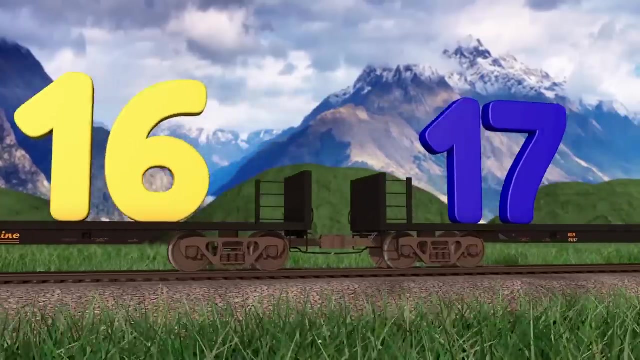 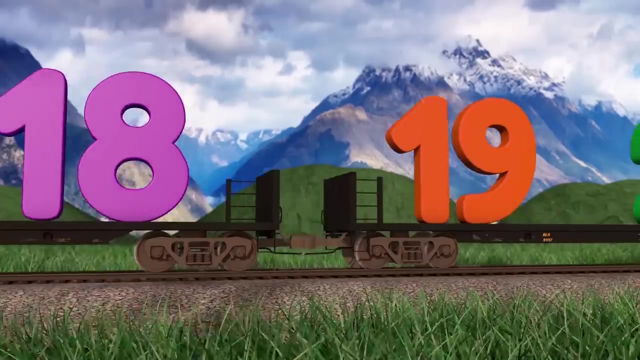 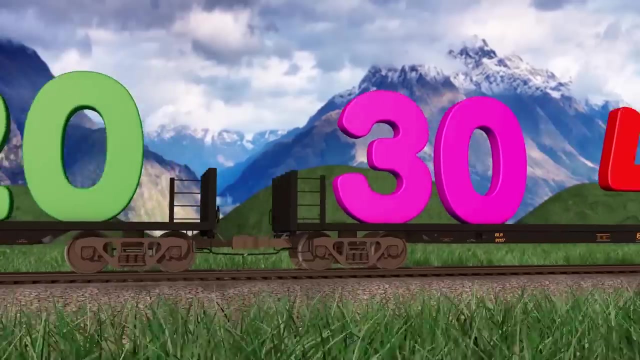 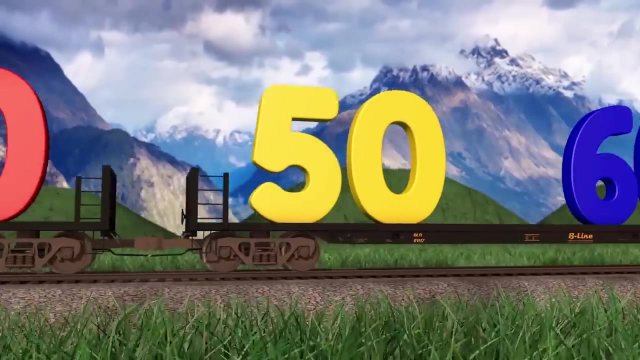 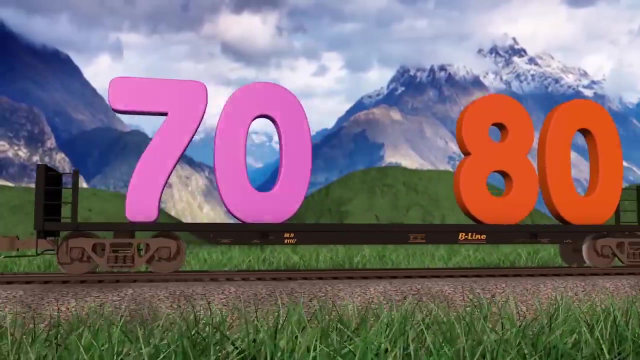 Eleven, Twelve, Thirteen, Fourteen, Fifteen, Sixteen, Seventeen, Eighteen, Nineteen And twenty. Now let's count up by tens, Thirty, Forty, Fifty, Sixty, Seventy, Eighty, Ninety. One hundred. Nice work, We did it, Great job. 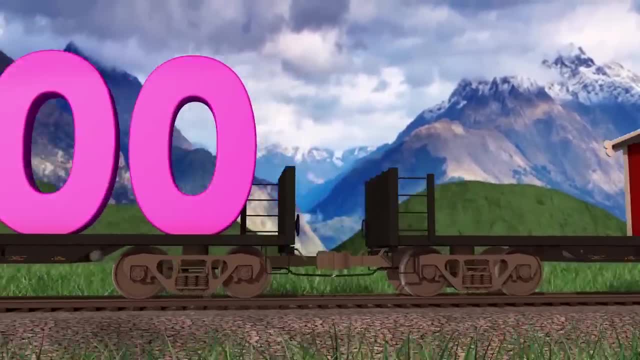 Wow, That was so much fun. OK, Lizzy, Let's review the numbers by tens. Here's ten balls. Hold on, Lizzy, You have to wait until we finish the lesson. You're going to have to wait until we finish the lesson. 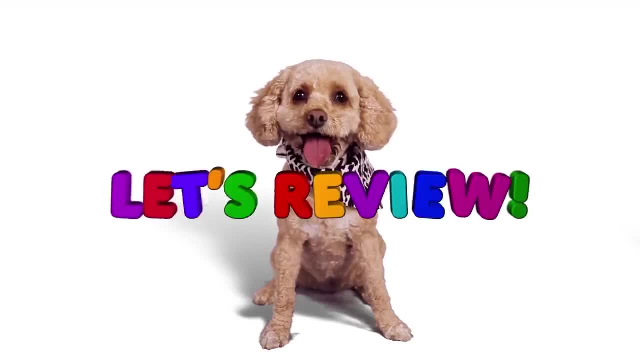 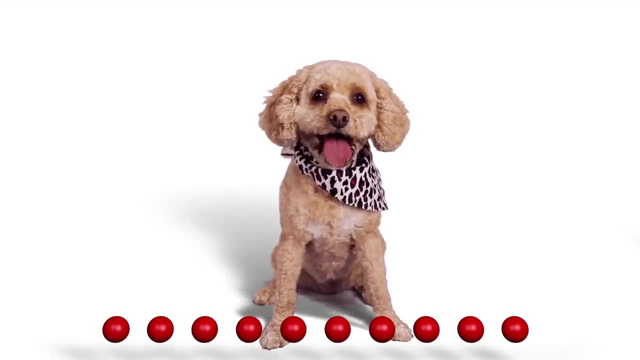 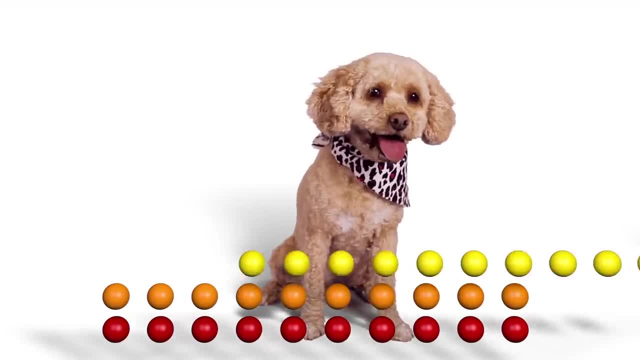 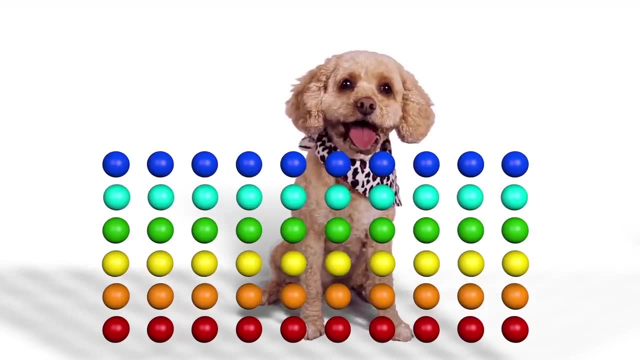 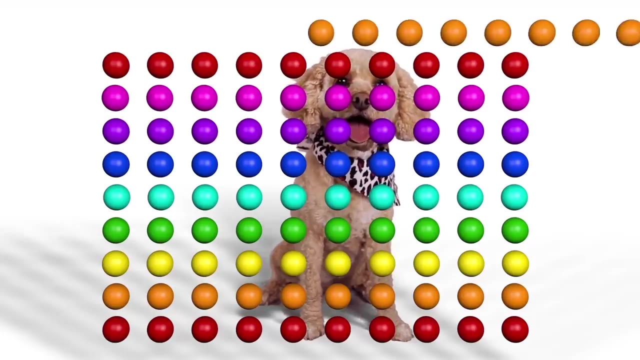 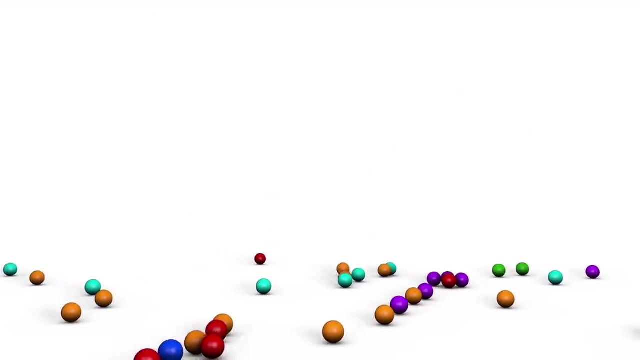 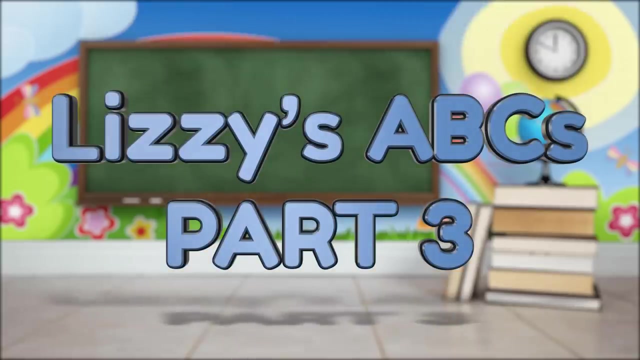 Before we finish the lesson: This is twenty. Here is thirty, Forty balls. This is fifty, Sixty, Seventy. Now we're up to eighty, Ninety, One hundred balls. OK, Lizzy, Go get them. Hey, Brainiacs, It's time to learn more of the alphabet with Lizzy. 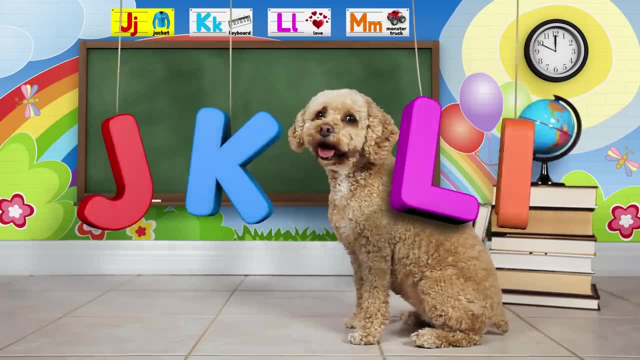 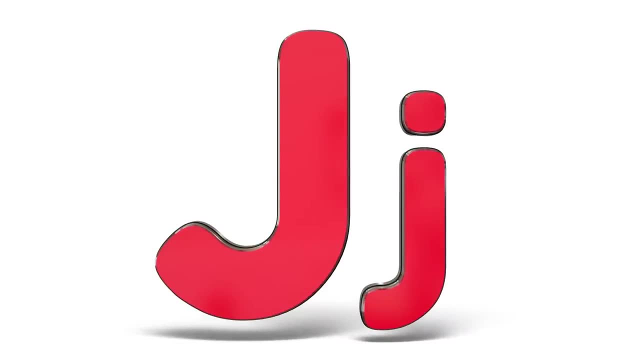 Today we're going to learn about the letters J, K, L and M. Alright, let's go. Our first letter for today is the letter J, and it looks like this: This is a capital J. This is a lowercase j. 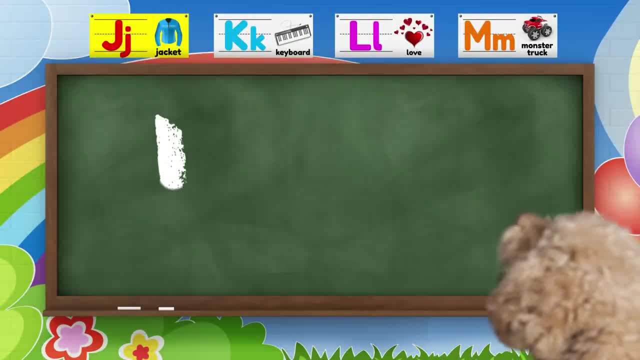 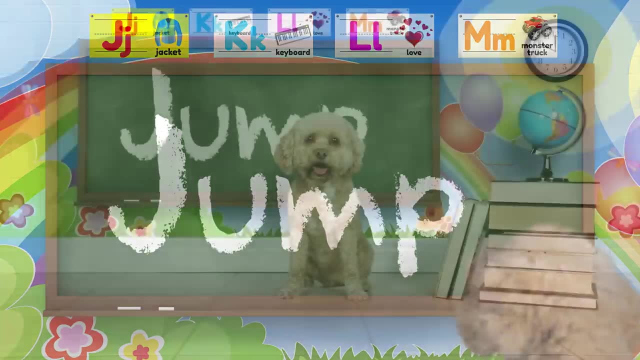 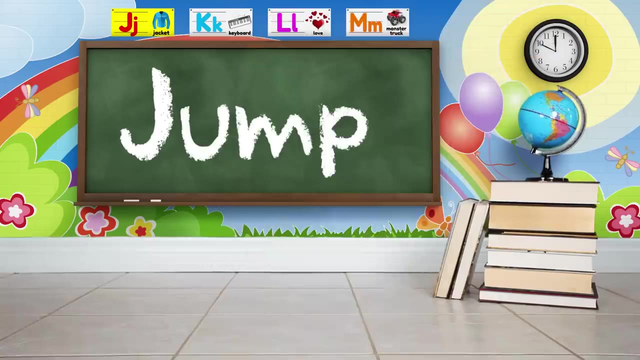 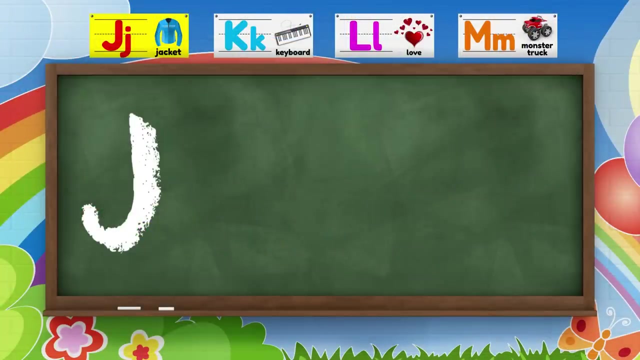 The letter J sounds like j. j like the word jump. Lizzy can jump really high. Show them how high you can jump. Lizzy, Jump really high. Oh, no, not that high. Another word that starts with J is jacket. 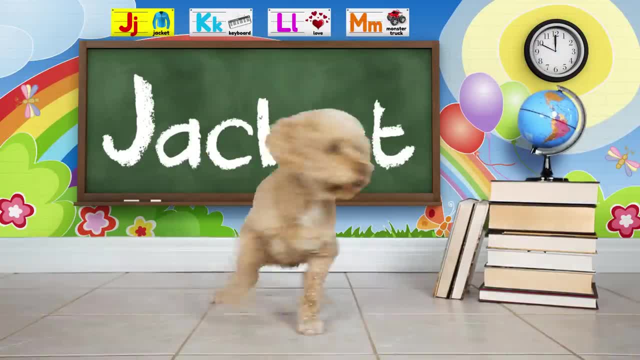 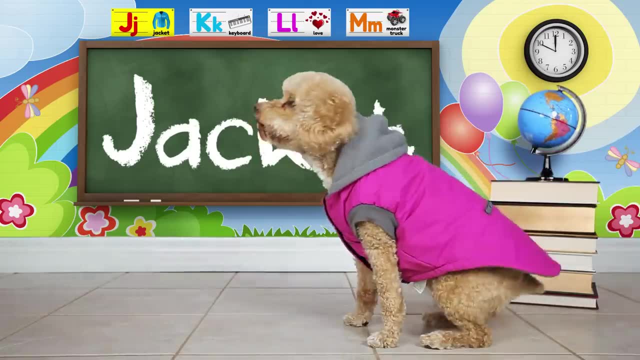 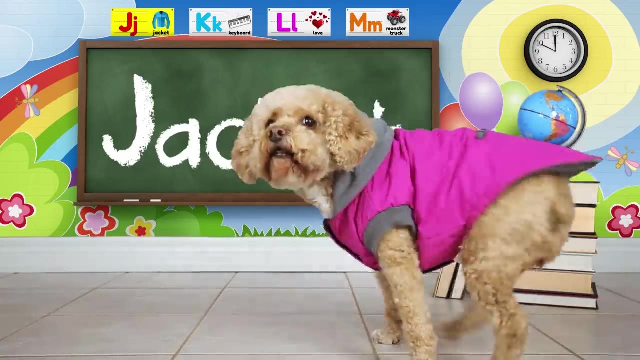 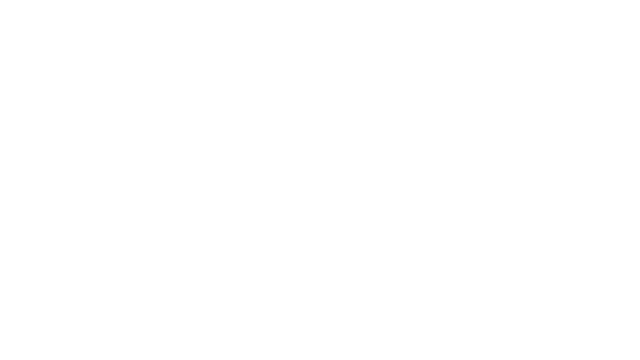 Why don't you show them how to jump? Show them your new jacket, Lizzy Good girl. Wow, that's a nice pink jacket. Next up is the letter K and it looks like this: Did you know that the word keyboard starts with K? 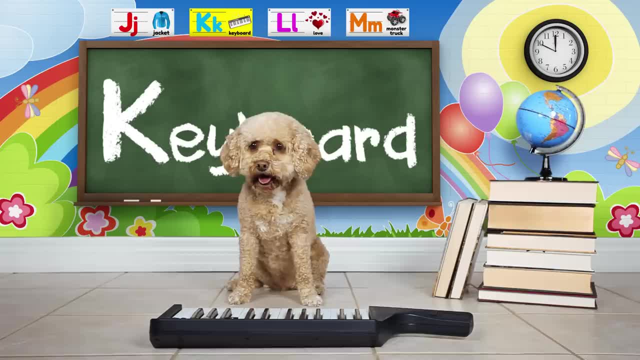 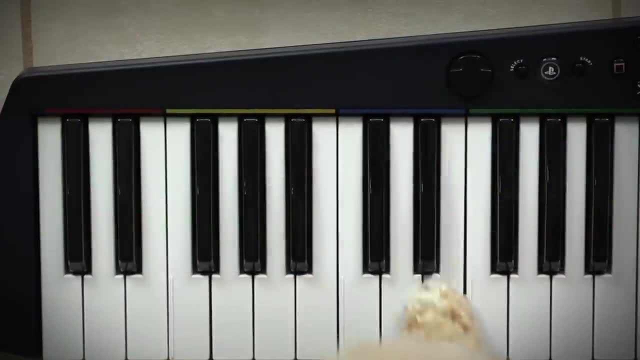 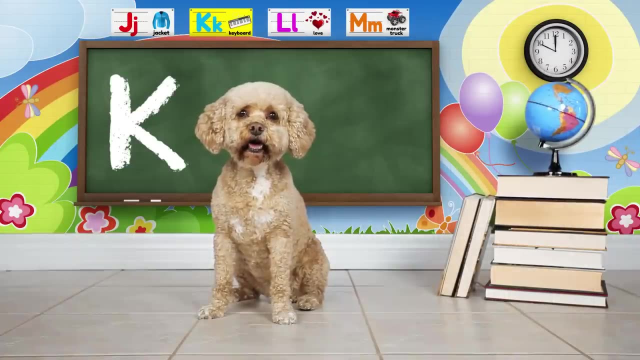 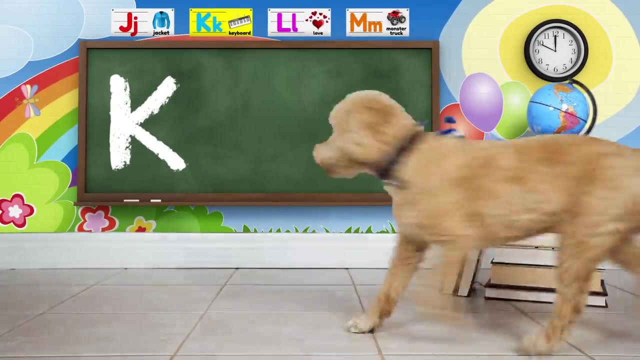 I wonder if Lizzy could play the keyboard. Wow, that's awesome. Okay, Lizzy, go get something else. that starts with the letter K. That's right, Good job, Kite. starts with K. It starts with the letter K. 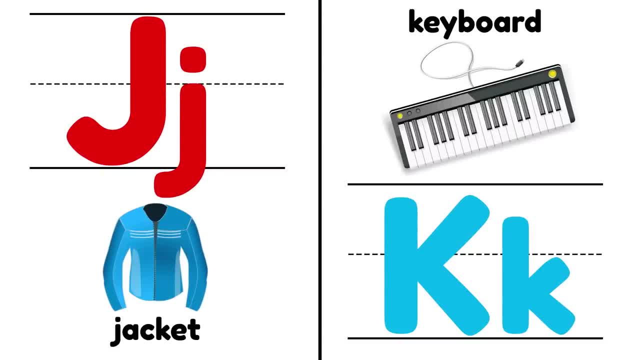 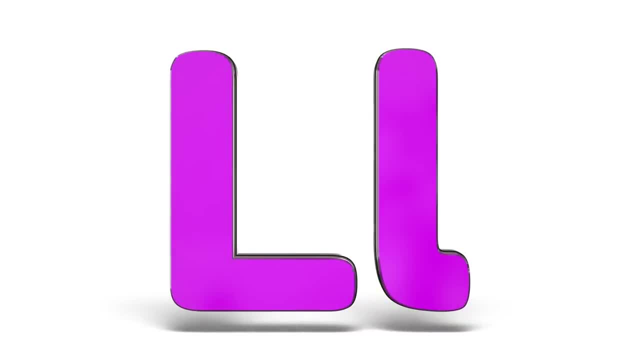 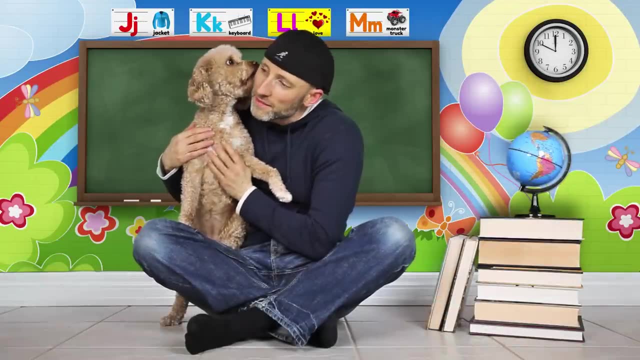 J j j for jacket, K k k for keyboard. Next up we have the letter L and it looks like this: We love Lizzy a whole lot. When she wants to show us how much she loves us, she gives us a lick on the cheek. 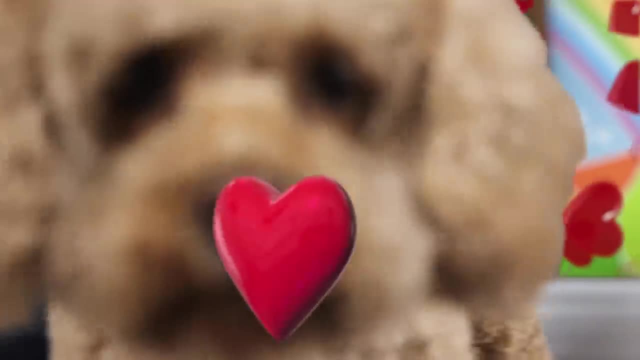 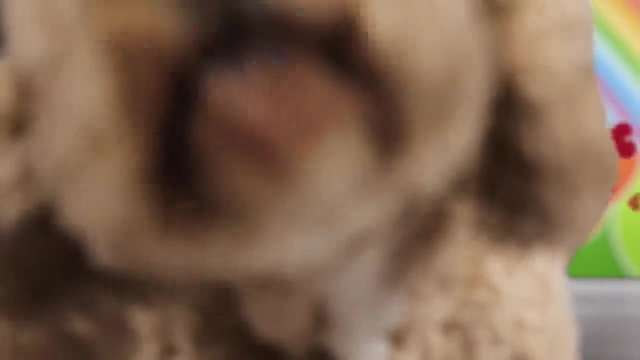 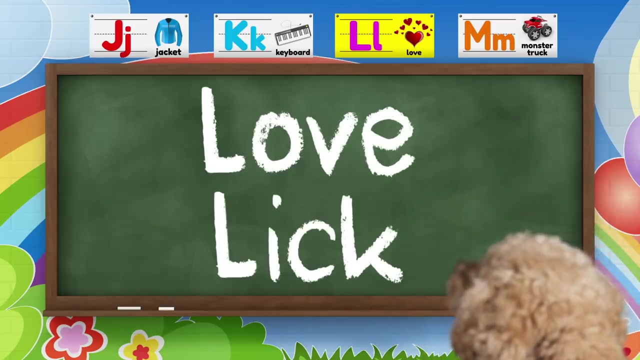 Hey, Lizzy, why don't you show the Brainiacs how much you love them too? We love them because we are all so sweet. We love you, Lizzy. The words love and lick both start with the letter L. The next letter of the alphabet is the letter M, and it looks like this: 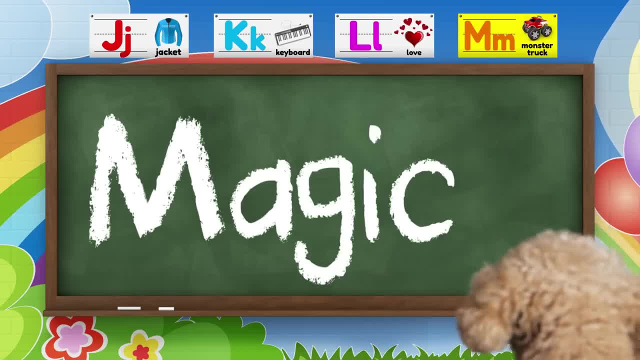 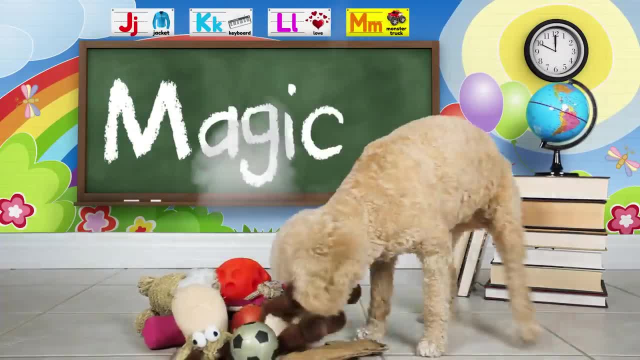 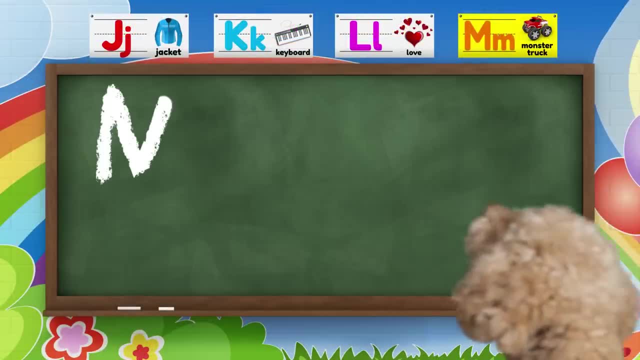 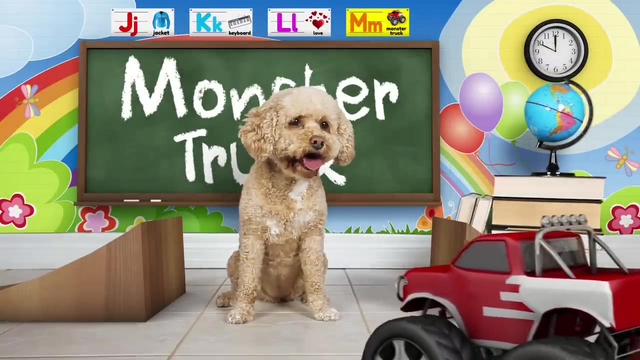 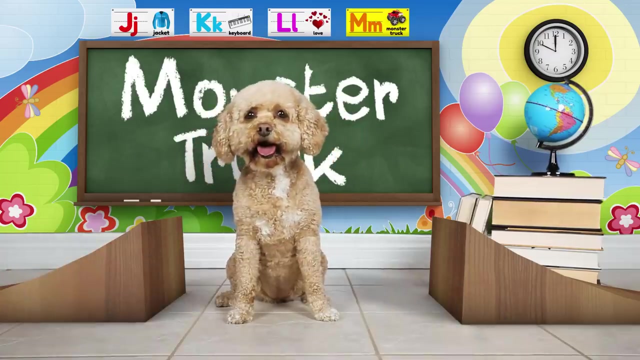 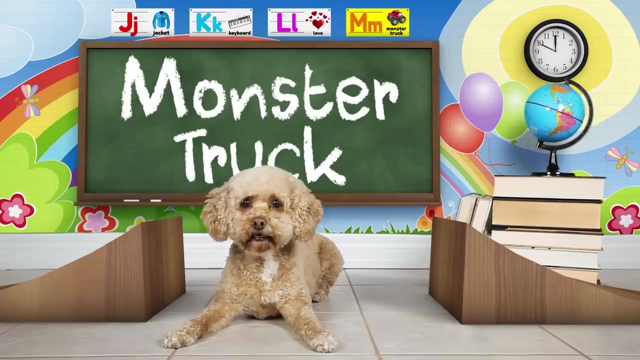 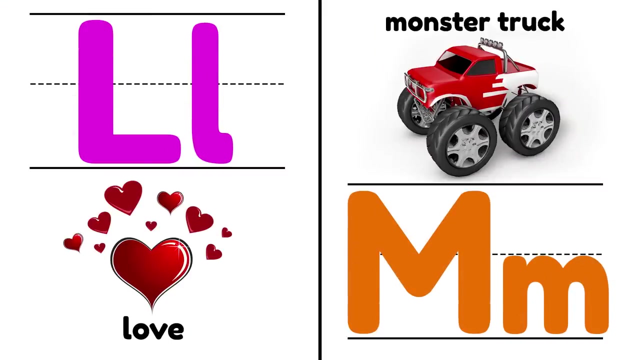 Abracadabra. Look at all those toys. Another thing that starts with M is Monster Truck. Let's see if the Monster Truck can jump over Lizzy Whoa. Listen to that engine roar. Wow, What a jump. L L L for Love. 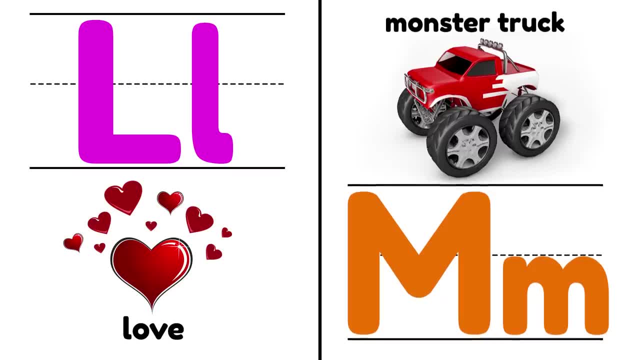 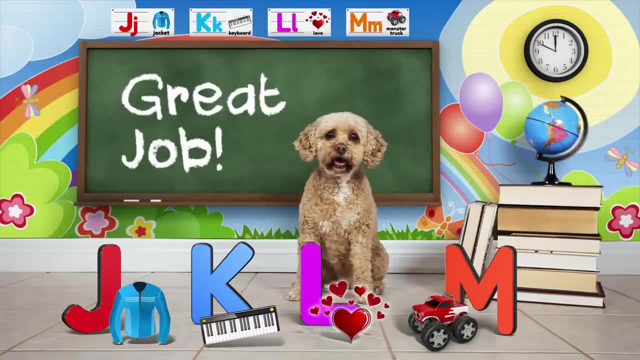 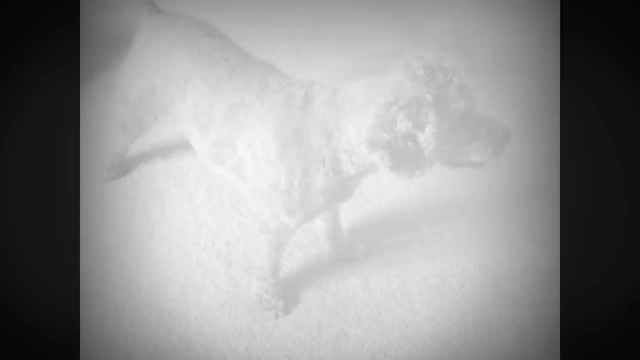 M, M, M for Monster Truck. Great job, Brainiacs. Now you know the letters J, K, L and M. Let's watch Lizzy play and grow from a puppy to 7 years old. This is Lizzy's Story. 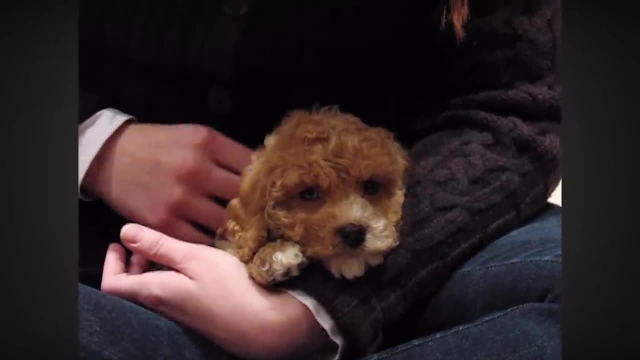 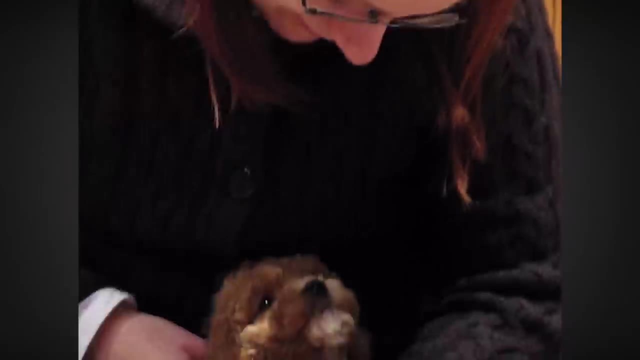 Lizzy was born on October 10, 2006.. Her mom was a cocker spaniel and her dad was a miniature poodle, Which makes her a cockapoo. She was born on a small country farm in Ontario, Canada. 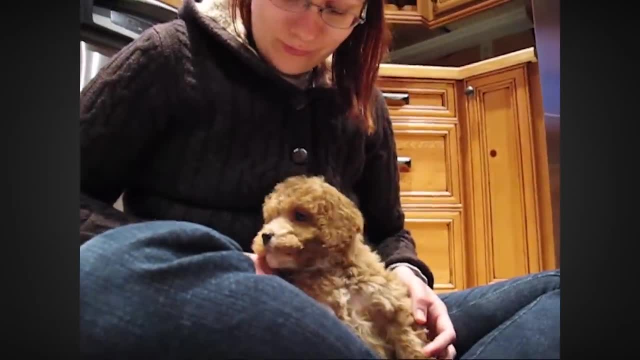 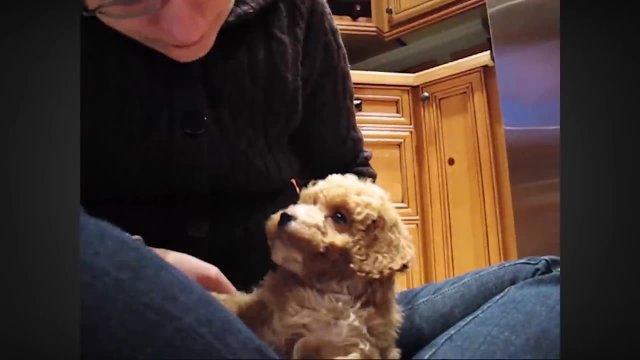 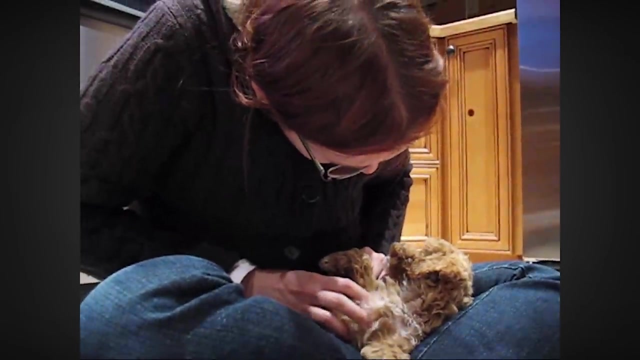 When we got to the farm to choose our puppy, Lizzy followed us everywhere we went And ended up choosing us instead. This is our first day with Lizzy, when she was only 2 months old. What are you doing? What are you doing there, Lizzy? 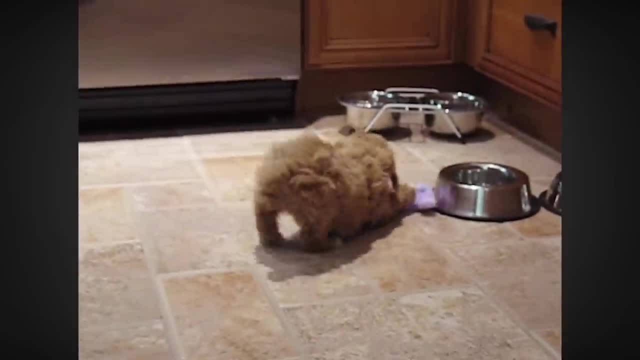 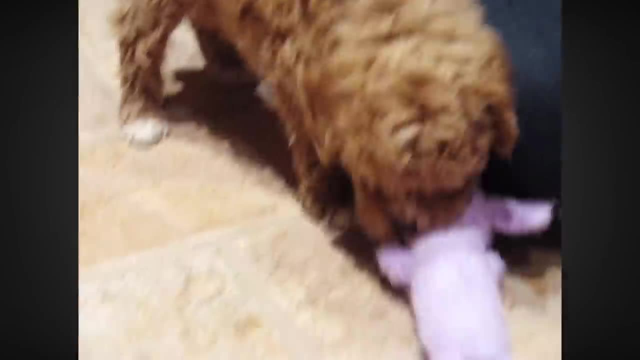 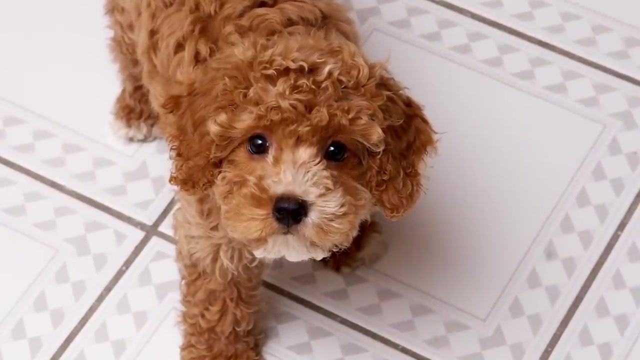 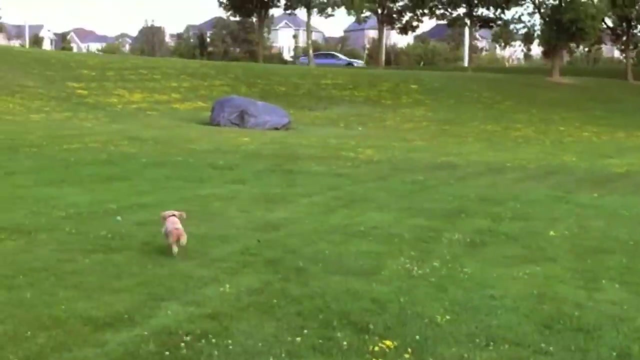 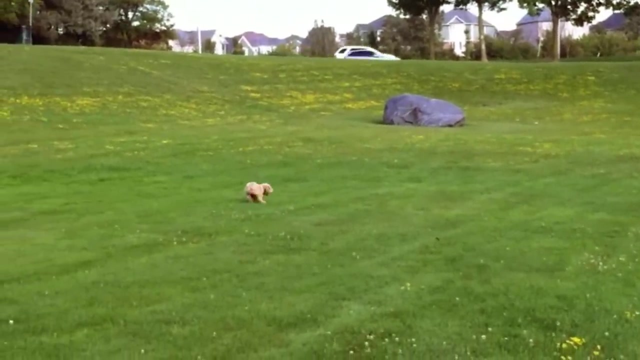 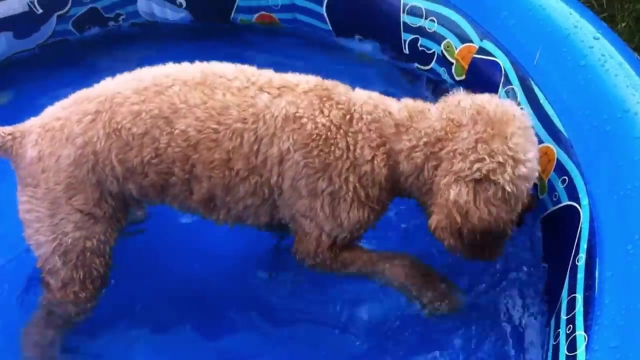 Lizzy's favorite thing in the whole world is playing fetch with her ball, But sometimes she gets a bit too excited. Whoops, Let's see that again. Lizzy loves playing in her pool on hot summer days, Especially when we throw in her ball. 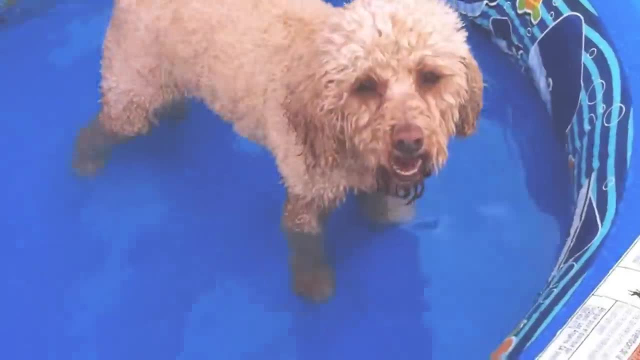 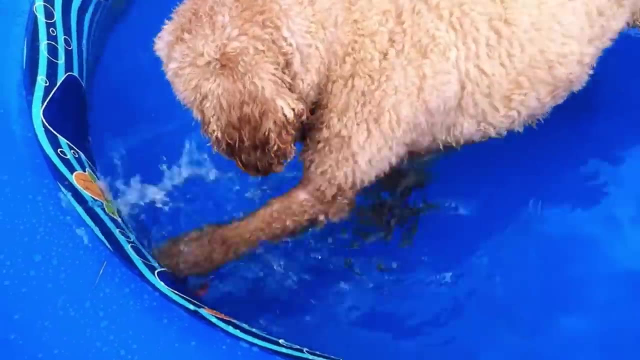 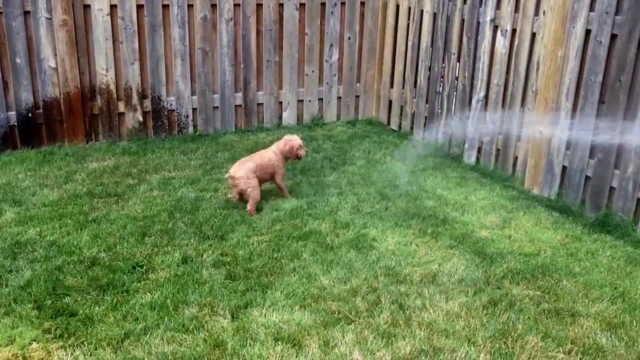 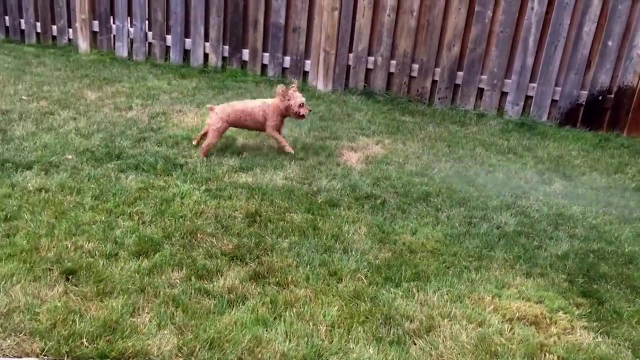 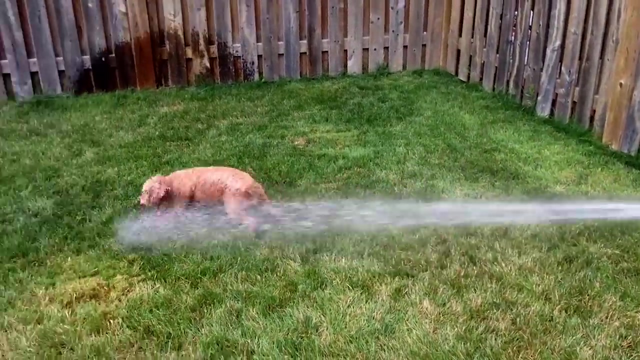 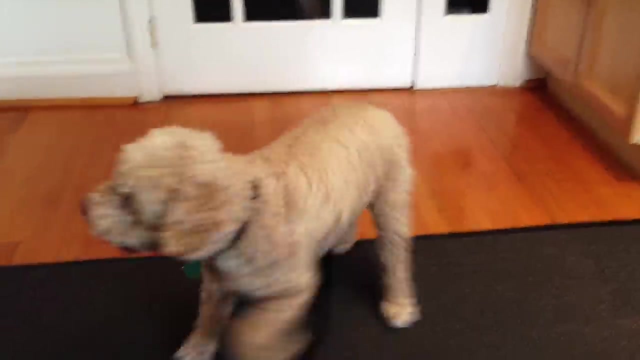 She has so much fun bobbing for her ball in the water. You got it out. One day, when I was watering the lawn, she invented a new game for herself. What a goofball. Lizzy loves going to the vet. She's very brave and doesn't even mind getting her needles. 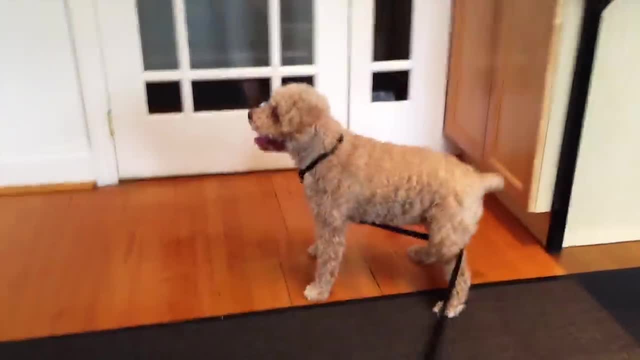 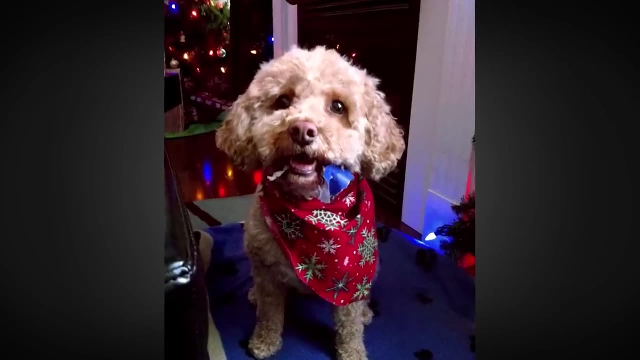 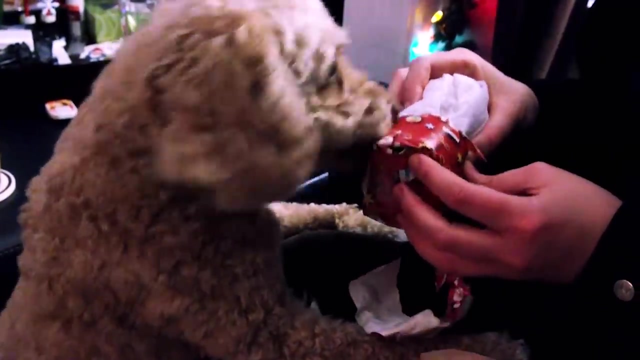 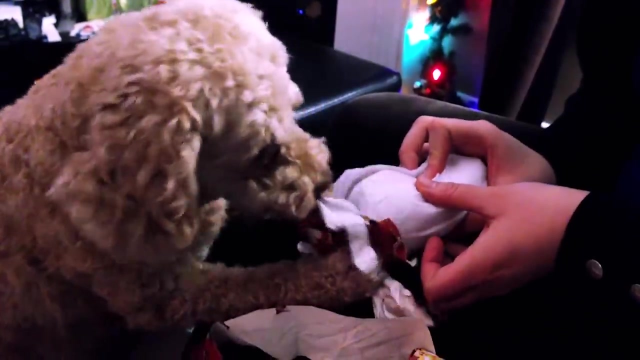 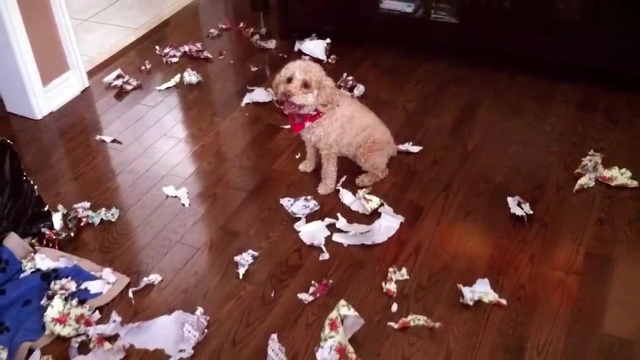 She gets really excited waiting for the doctor to arrive. What's your favorite part of Christmas? Lizzy's favorite part is opening all of her presents. The only problem is she can make a bit of a mess, But look how happy she is. 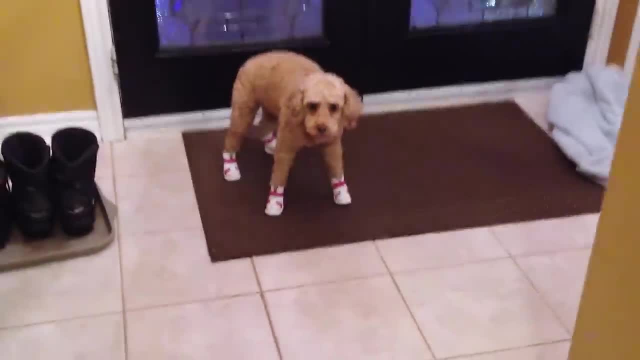 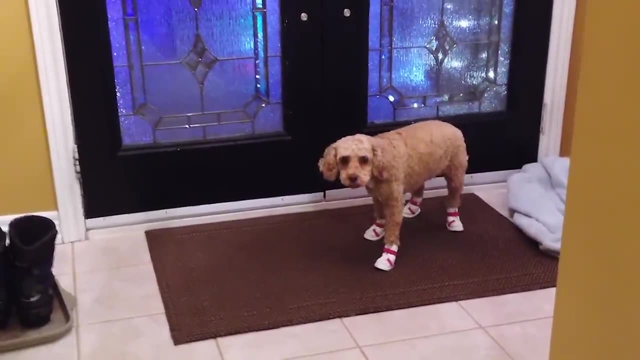 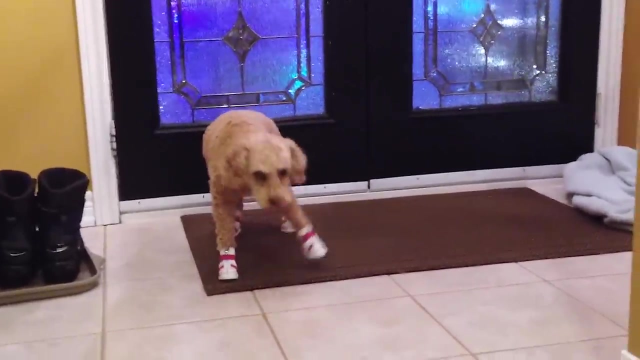 On really cold days, Lizzy's paws need protection from the ice, But she's not sure what to make of her new winter boots yet. Come on, Come on, That's good for you, This one you want. There's one thing that Lizzy loves almost as much as her ball. 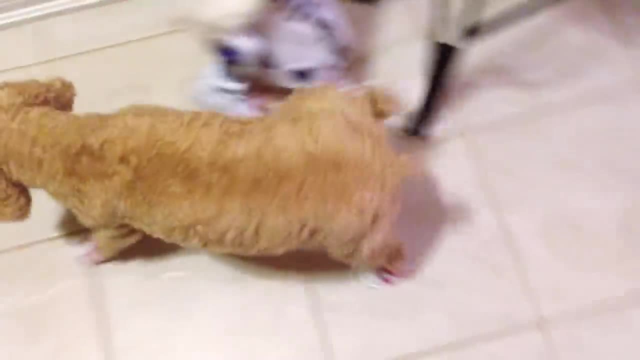 and that's cheese Which I love so much, And it's her обязательно favorite food. She really likes mealnissees. Place them down when you get your one And put the amounts in the bowl. in a bowl It's like plates. 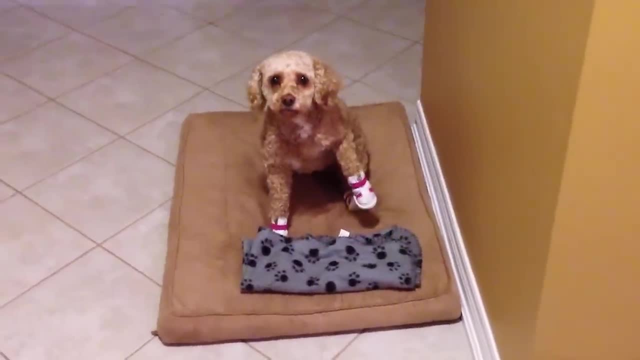 She loves all kinds of dishes. Maybe let me swear she doesn't chip when she makes one. Come on, idols. My name's Lola. I'm a cheese Solid. It's you? My name is Lola, and this is my brother, Nick. 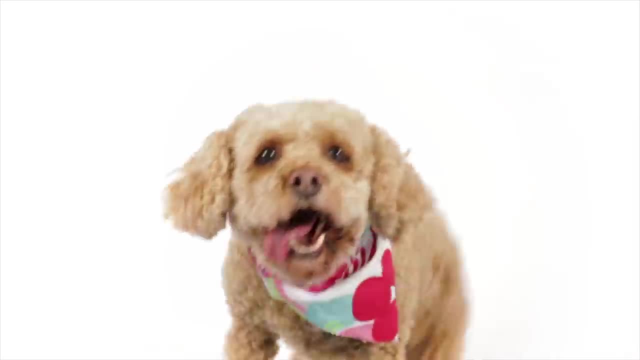 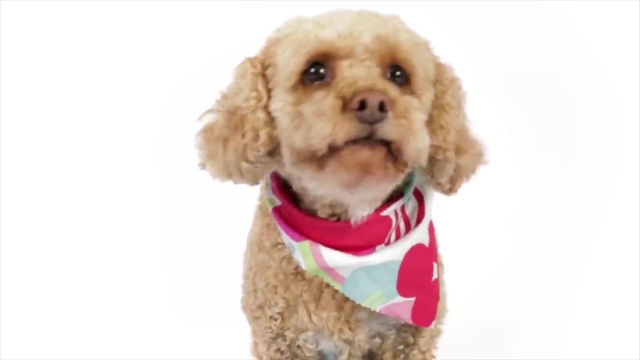 Happy Christmas Miles in the blends. Once a little fluttering ofLaLaB interview Memories Sur consonant să experience it. She'll do almost anything for cheese, And that's Lizzy as she is today. I hope you enjoyed her story. 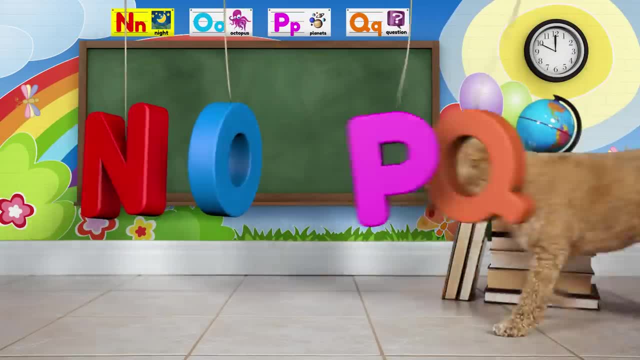 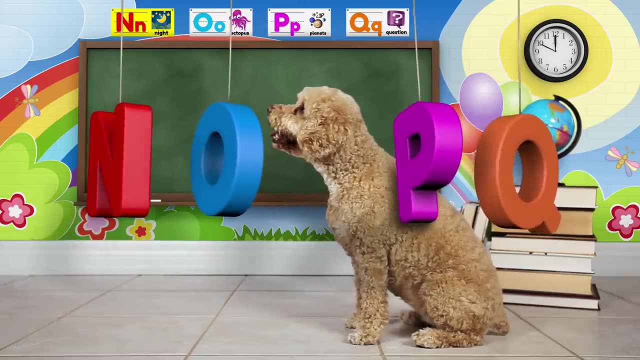 Hey Brainiacs, it's time to learn more of the alphabet with Lizzy. Today, we're going to learn about the letters N, O, P and Q. Alright, let's go. Our first letter for today is the letter N, and it looks like this: 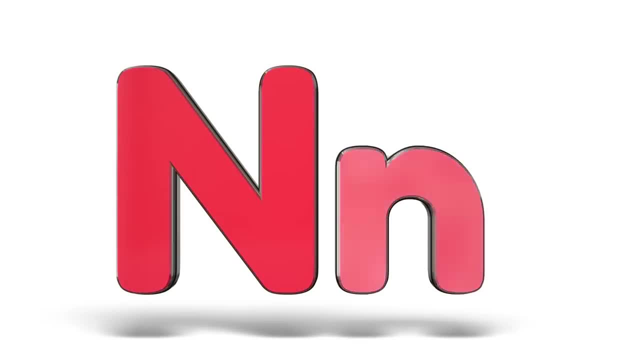 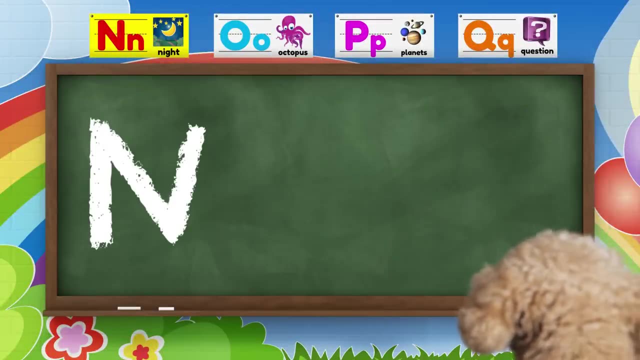 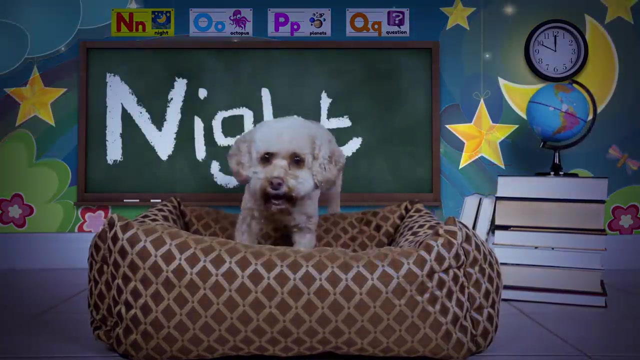 This is a capital N. This is a lowercase n. The letter N sounds like nuh, nuh, like the word night. Okay, Lizzy, it's night time, Time for bed. Lizzy loves to snuggle up in her new bed at night. 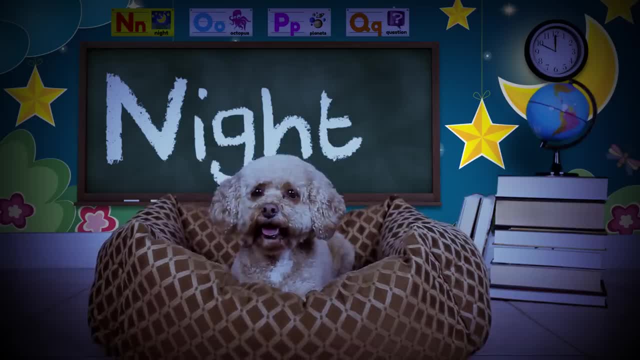 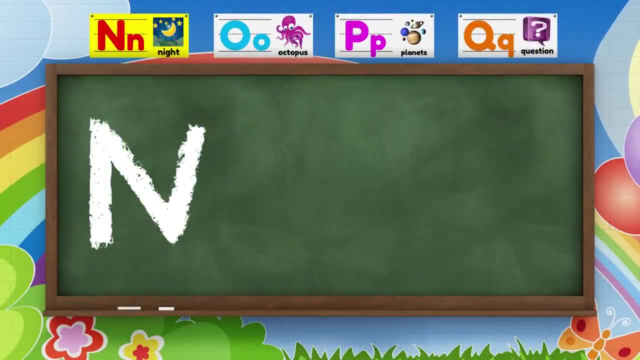 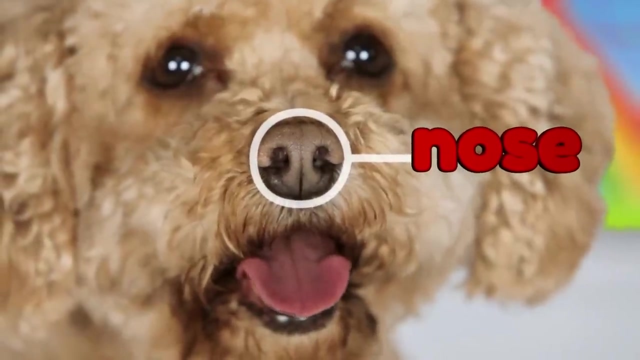 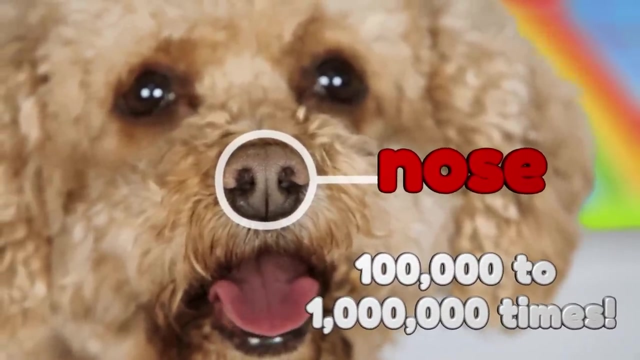 Go on, get cosy. That's a good girl. Another word that starts with N is nose. Lizzy has a really good nose. She can smell 100,000 to a million times better than we can with her dog's nose. Next up is the letter O, and it looks like this: 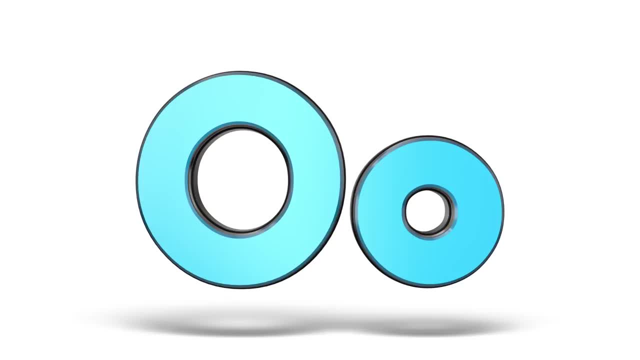 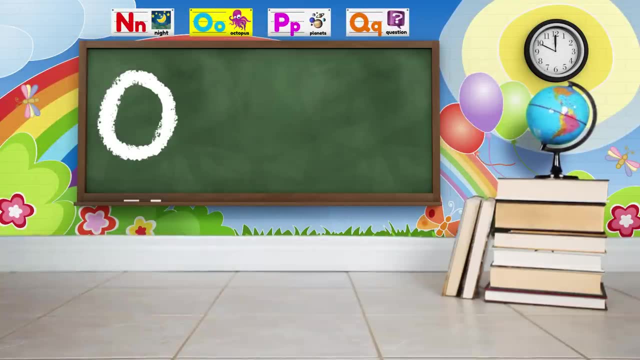 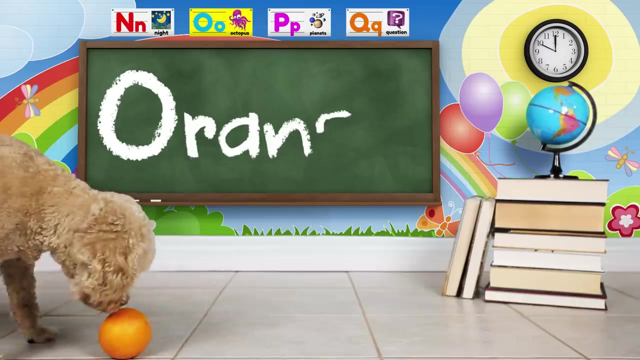 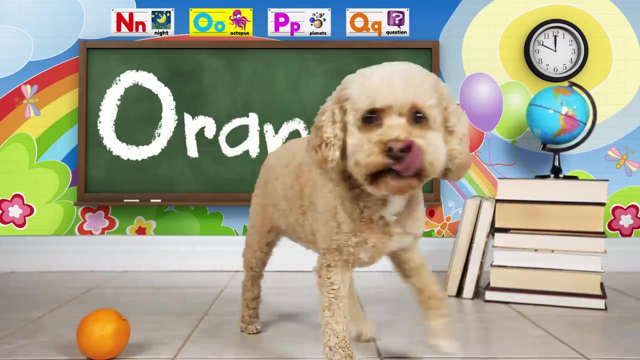 The letter O sounds like oh or ah. Hey, Lizzy, go fetch something that starts with the letter O. That's right, orange. The word orange starts with the letter O. Oranges are tasty and good for you too. What has eight arms? 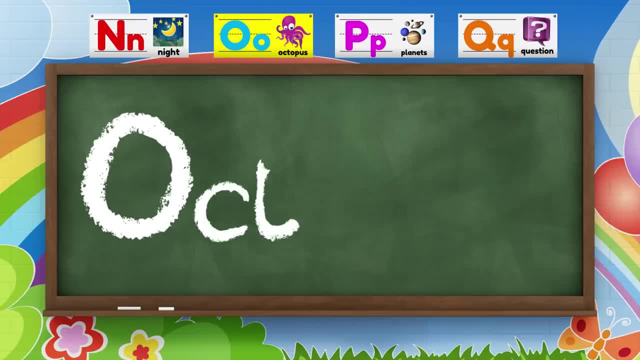 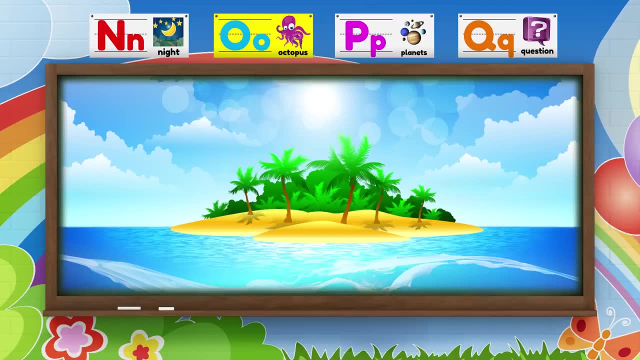 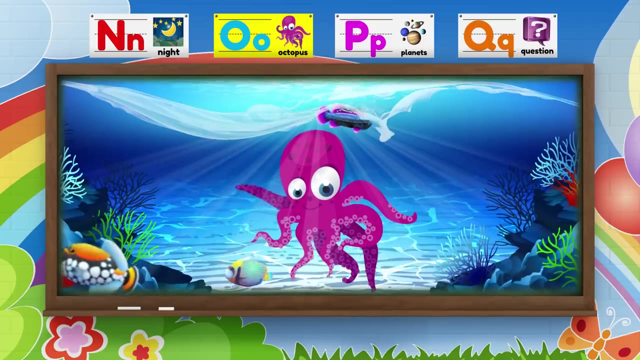 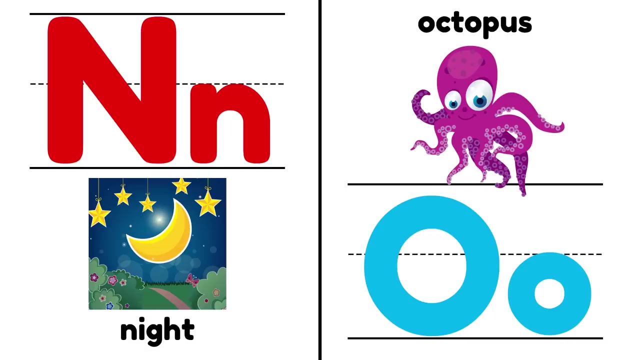 And lives in the ocean. That's right, it's an octopus. Where's the octopus? Can you find him? There he is. Hi, Mr Octopus, Nuh nuh, and for night, Ah ah, O for octopus. 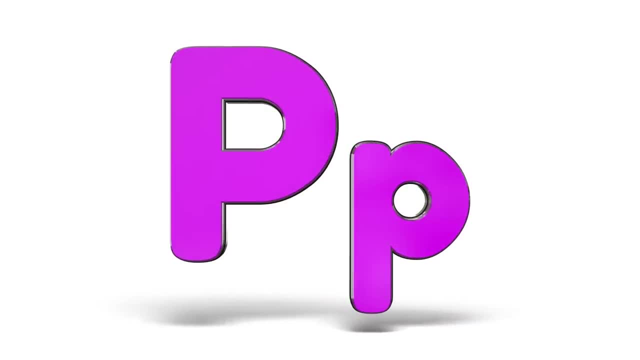 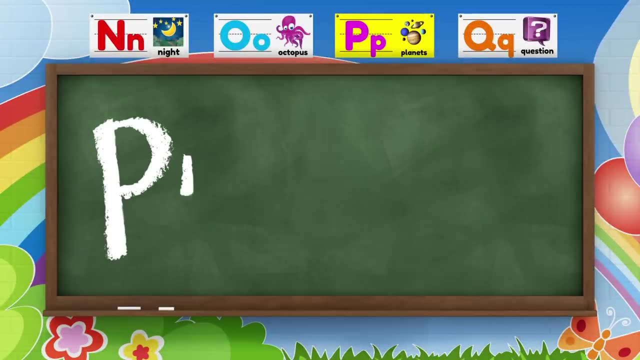 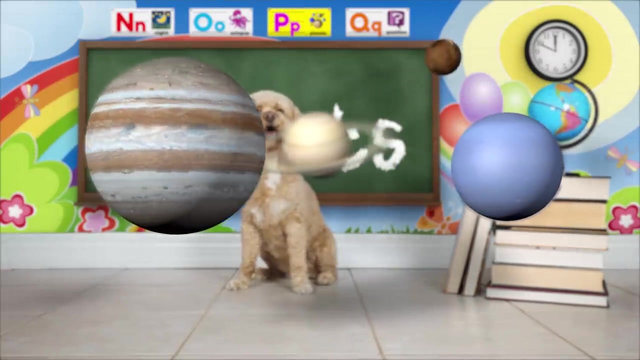 Next we have the letter P and it looks like this. The letter P sounds like puh Puh. One word that starts with P is planets. Planets are so cool. There are eight planets in our solar system. We know that Earth is one of them. 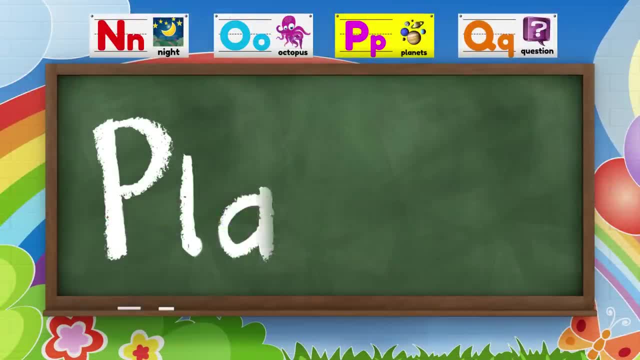 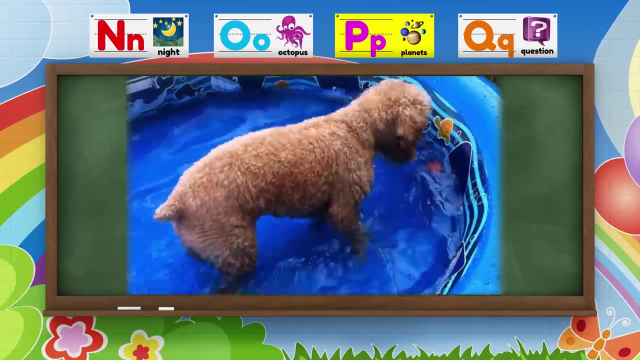 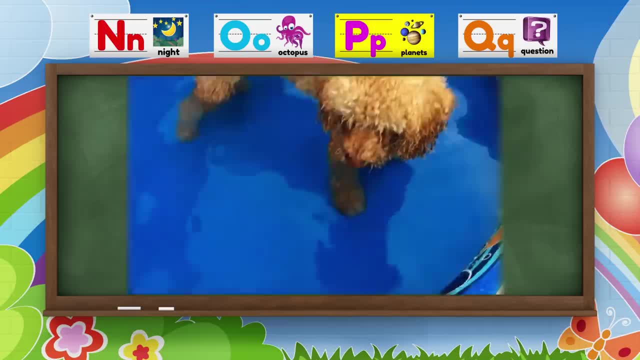 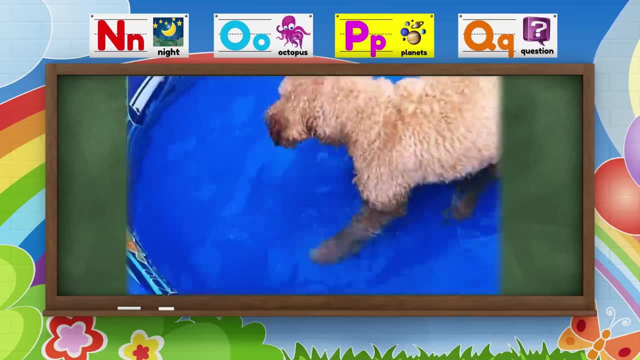 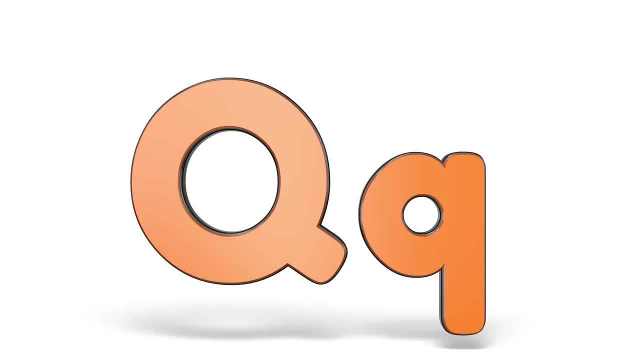 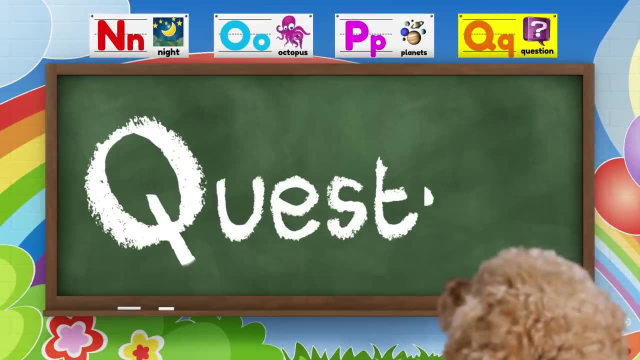 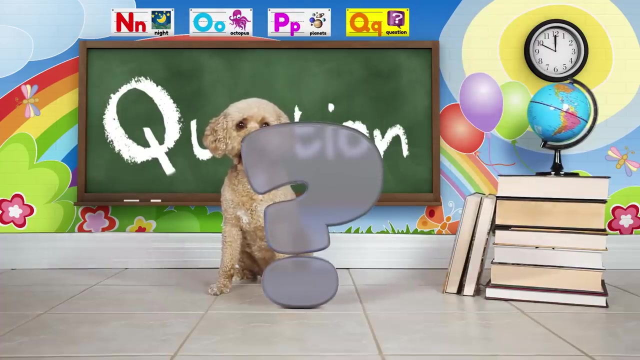 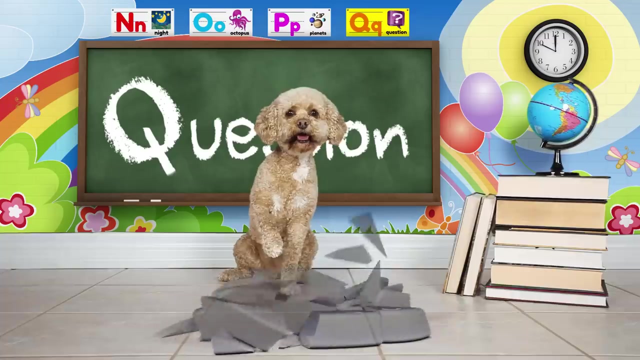 I call this the naturopathic rose. What if it's Poo? What if the lap is Poo? What if it's Poo? the word question starts with the letter Q, like when you ask the question. what happens if Lizzie pushes over the question mark? oh no, she broke it. I guess we know the. 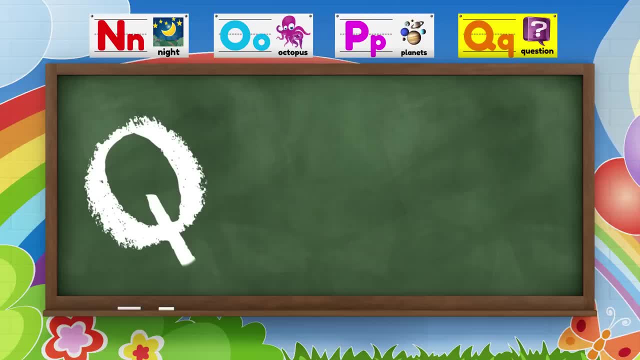 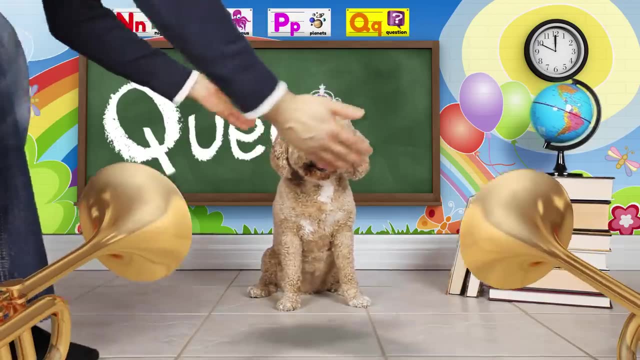 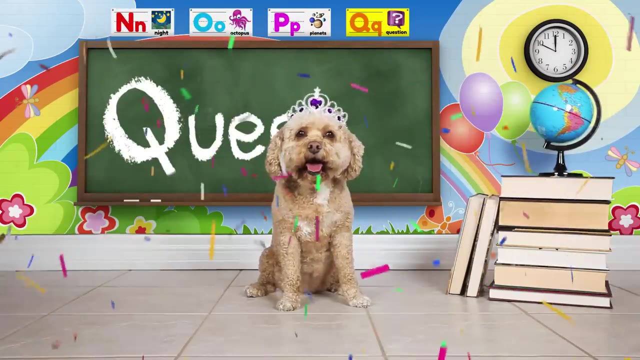 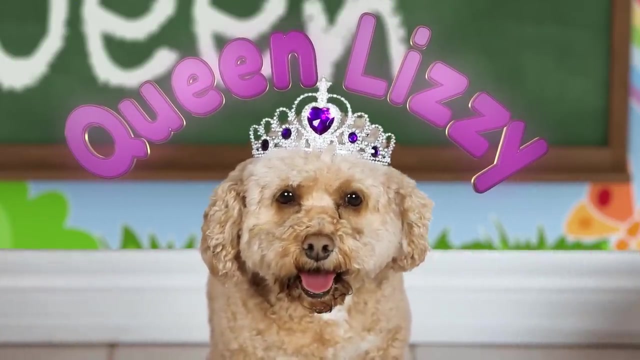 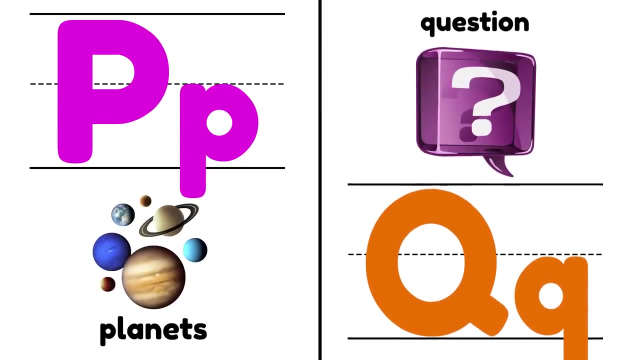 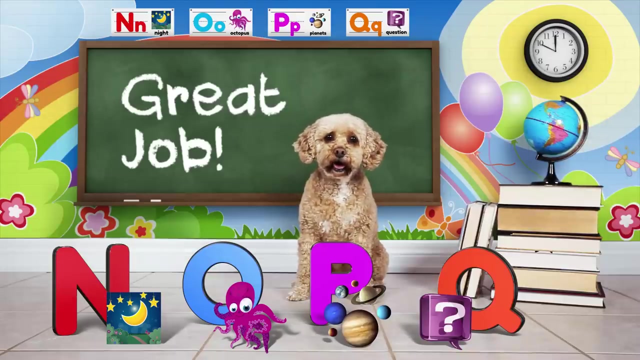 answer to that question. another word that starts with Q is Queen. here I hear by crown the Lizzie Queen of the alphabet: huh huh. P for planets. P for planets, P for planets. huh huh. Q for question. great job, now you know the letters N, O, P and Q. 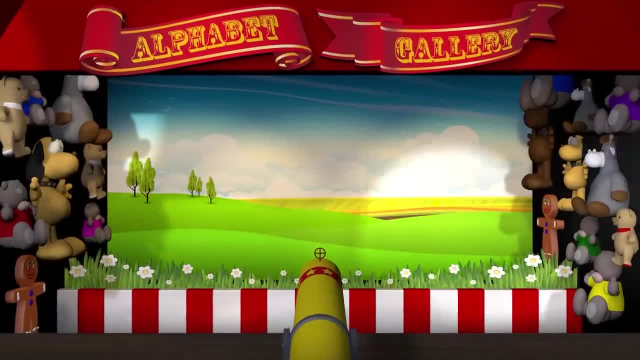 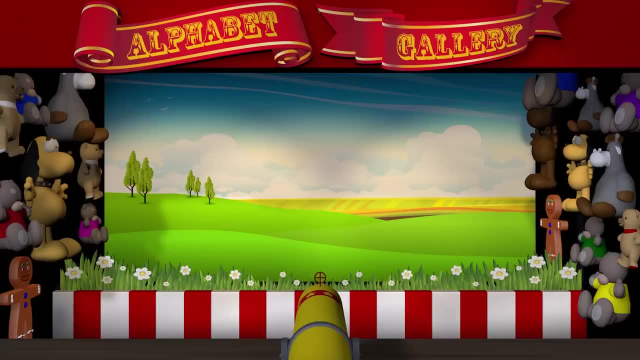 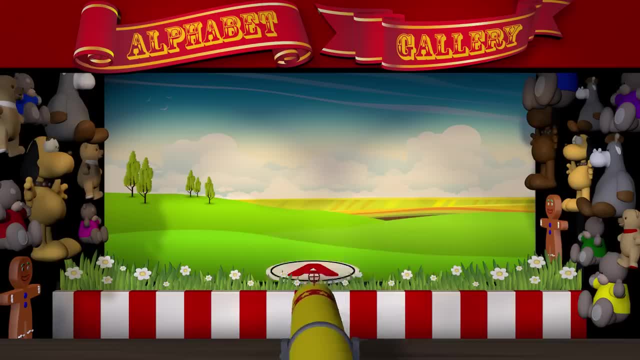 let's see if we can get all of the letters. let's see if we can get all of the letters A, B, B, C, D, D, D, F, G, H, H for Horse, I, J, J- Where'd the ball go? Lizzy, K, L, L for Lion. 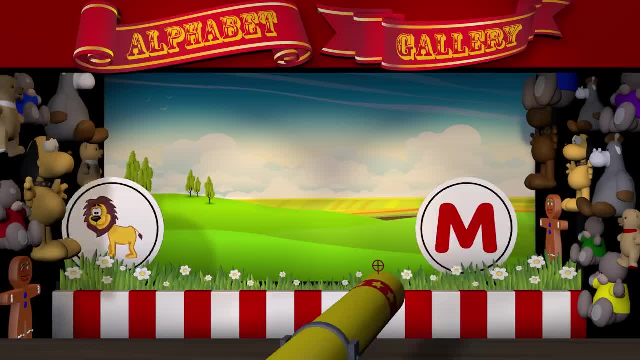 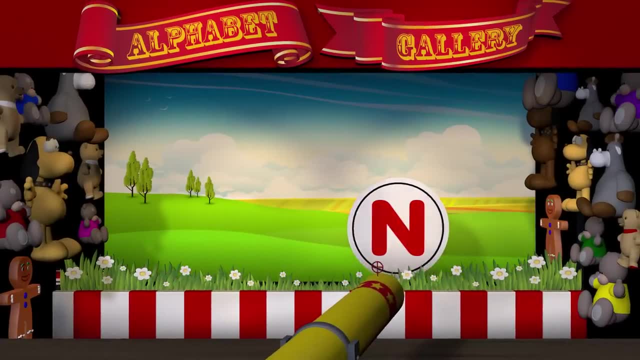 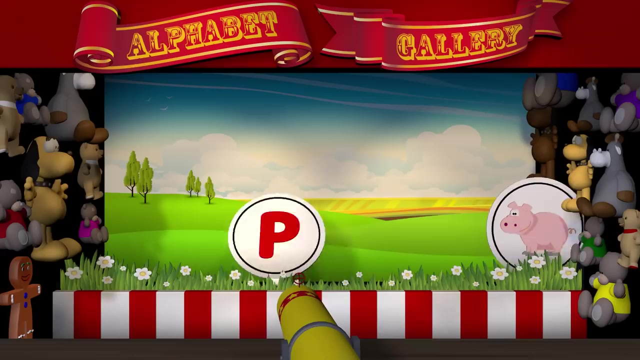 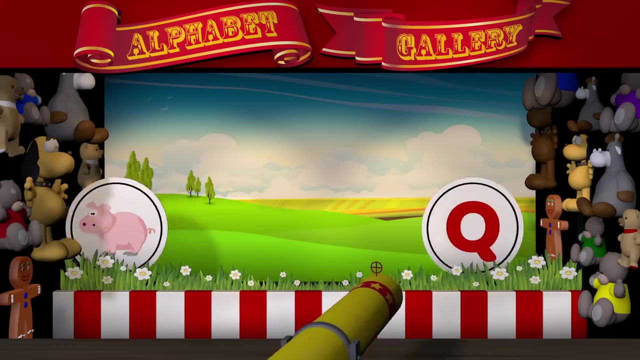 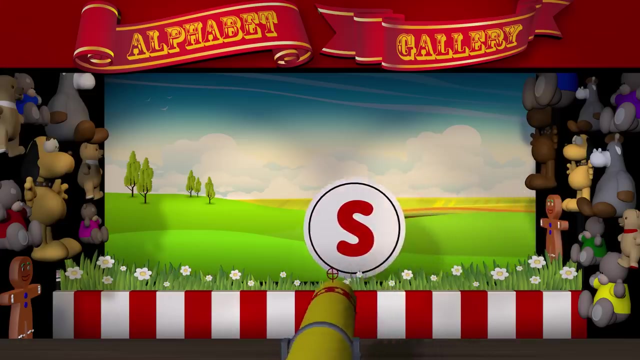 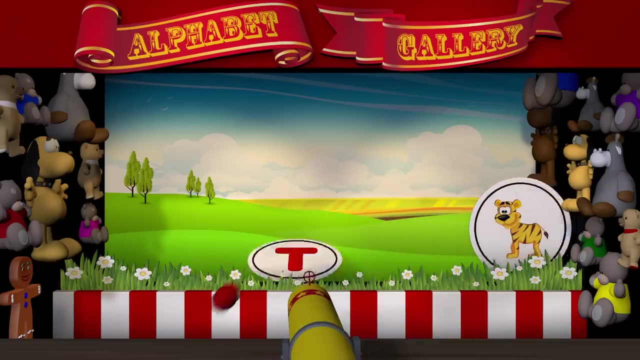 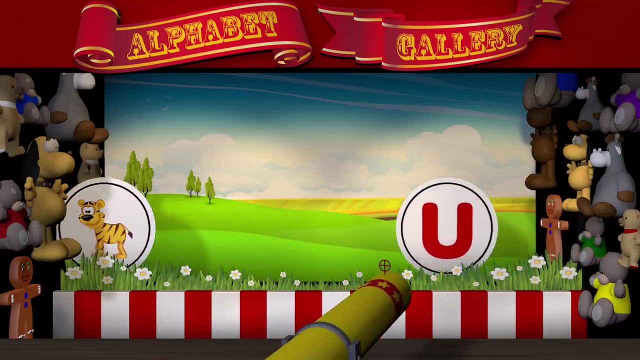 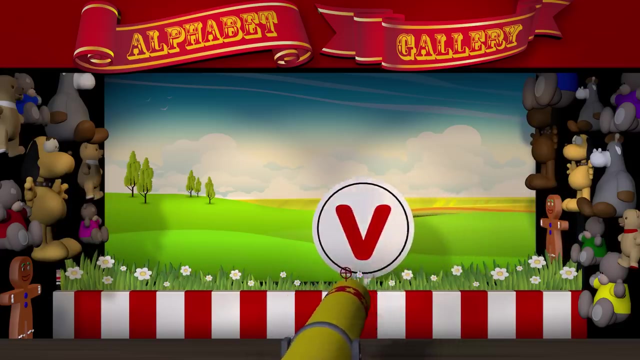 M Look out N? Oops, we missed O O, O, P, P, P, P for Pig, P for Pig. Q, Q, R, R, R, R, S, S, S, T, T. Go get that one. Lizzy T for Tiger, T for Tiger. U, U, V, V, V W. 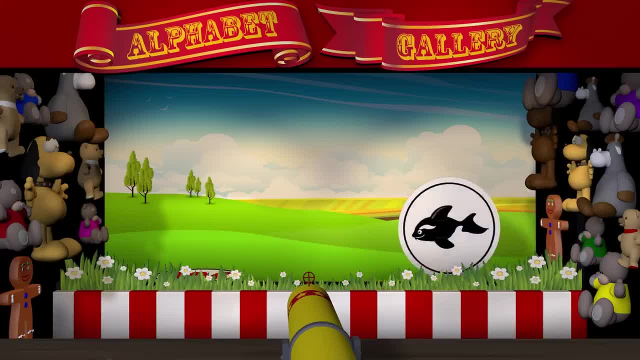 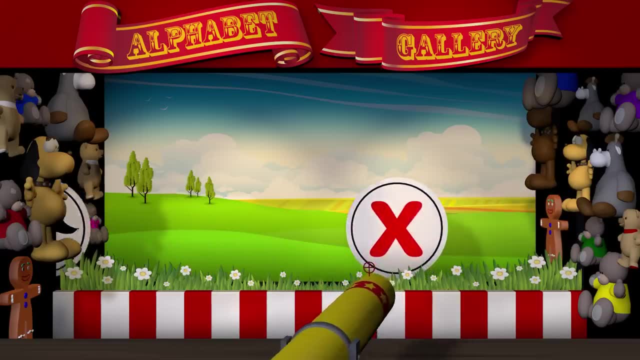 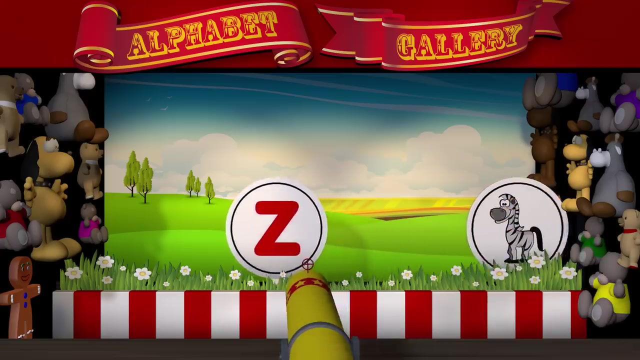 W, W, W for Whale, W for Whale W, X, X, Y, Y. Uh oh, that was our last ball. Quick get another one. Quick get another one. Z Z, We got it. And Z for Zebra, Z Z, Woohoo, We win. 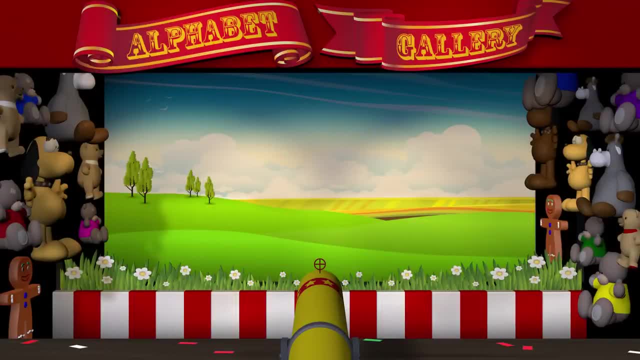 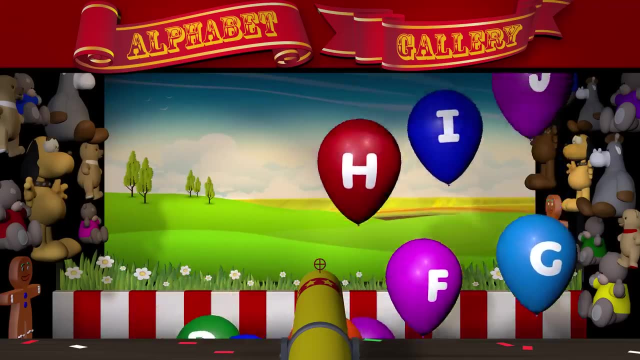 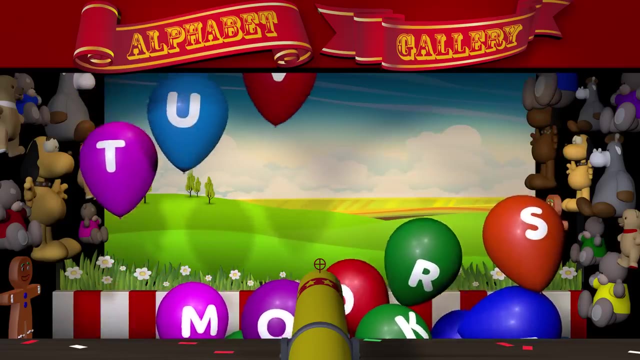 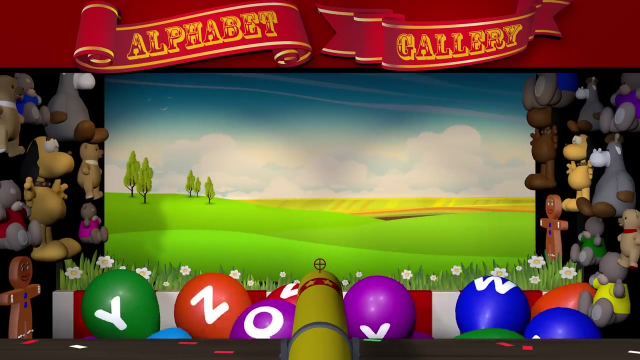 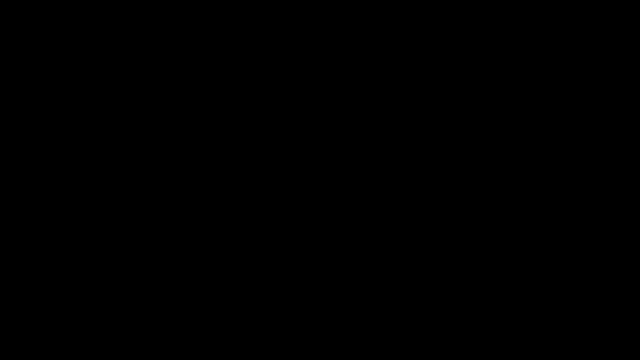 We got them all. A, B, C, D, E, F, G, H, I, J, K, L, M, N, O, P, Q, R, S, T, U, V, W, X, Y and Z. Now I know my ABCs. Next time won't you sing with me, Mark? Hey, that's not even the right ball. 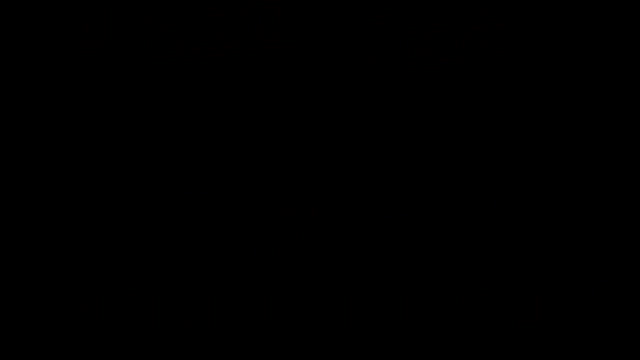 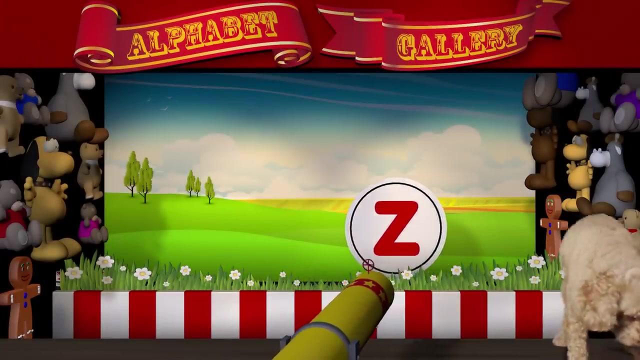 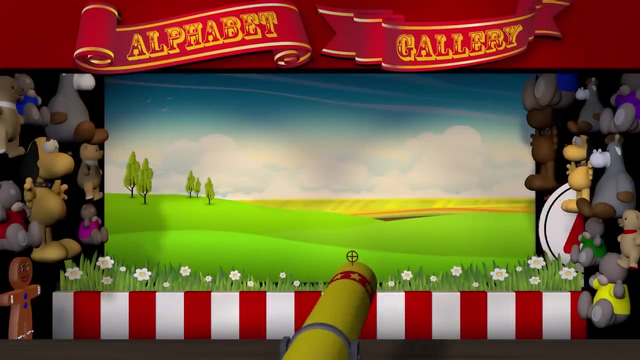 Where'd you get that, Marker? Hey, you forgot the ball. Hey, you forgot the ball. Go get it. Go get it, Marker. Hey, what's wrong with this thing, Marker? Hey, what's wrong with this thing? Hey, what's wrong with this thing? 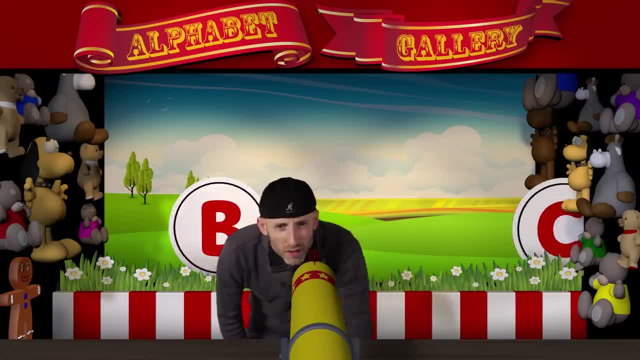 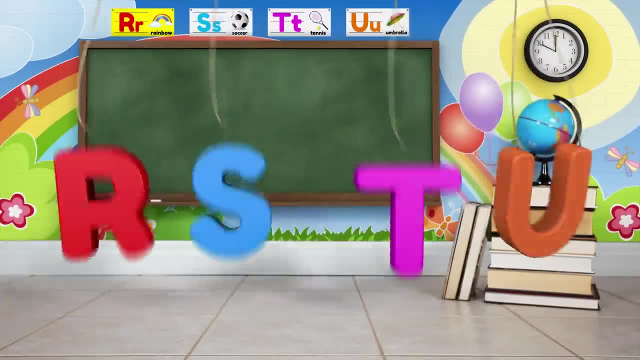 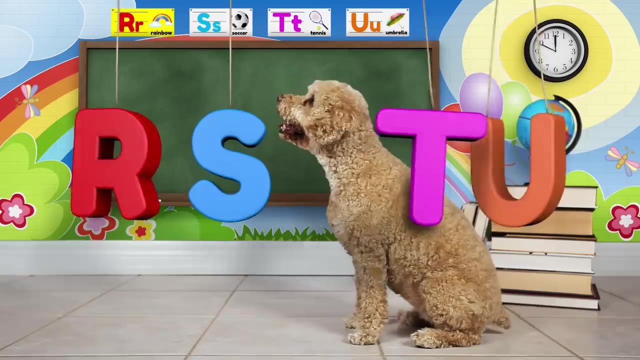 Hey, what's wrong with this thing? Oh Yay, Hey, Brainiacs, It's time to learn more of the alphabet with Lizzy. It's time to learn more of the alphabet with Lizzy. Now we're going to learn about the letters. 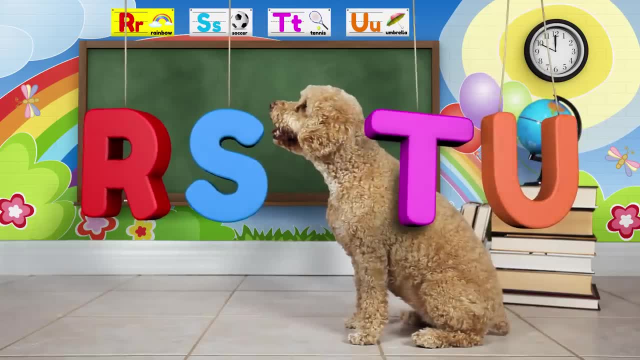 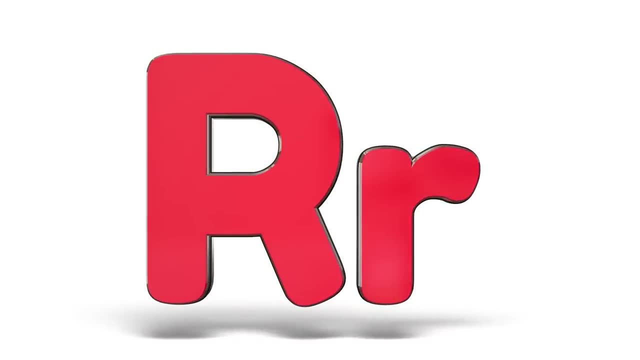 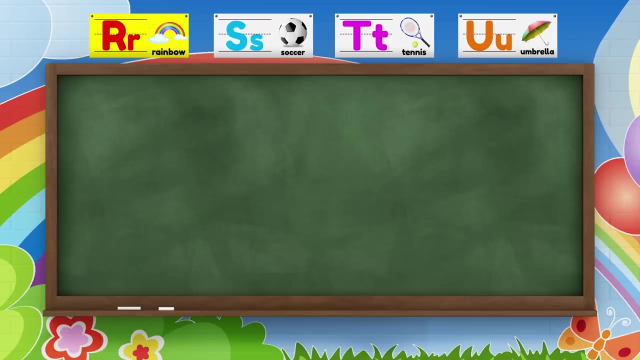 R S T and U R S T and U. Alright, let's get started. Our first letter for today is the letter R. Our first letter for today is the letter R, and it looks like this: This is a capital R. This is a lowercase r. This is a lowercase r. 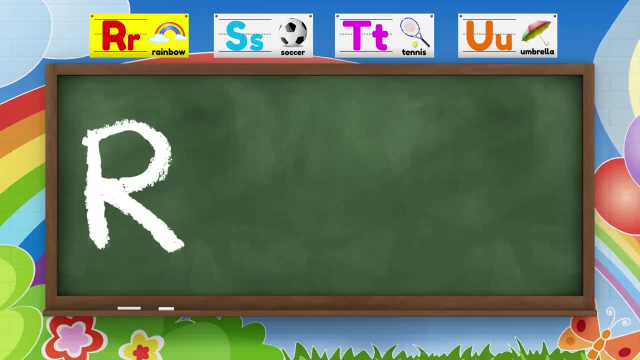 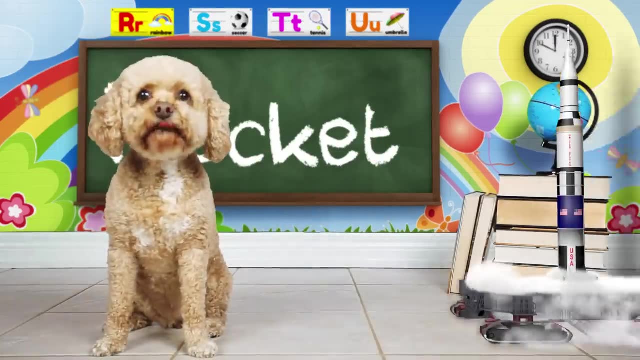 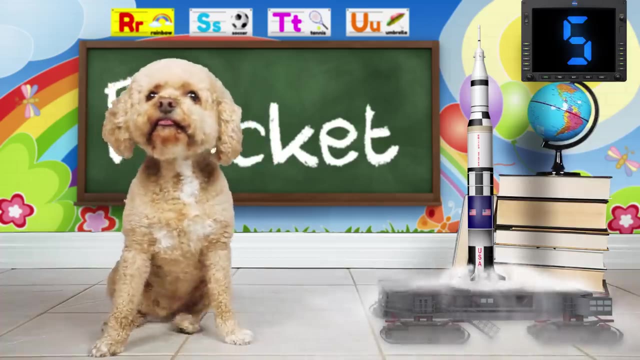 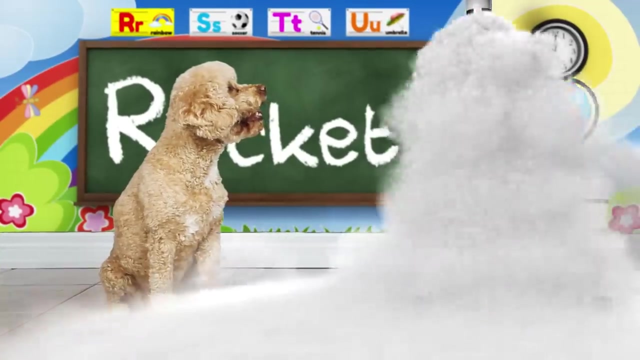 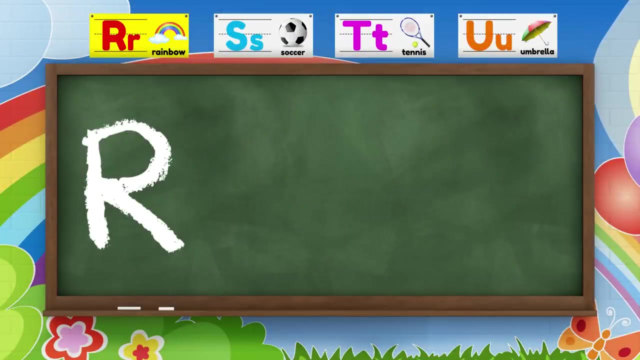 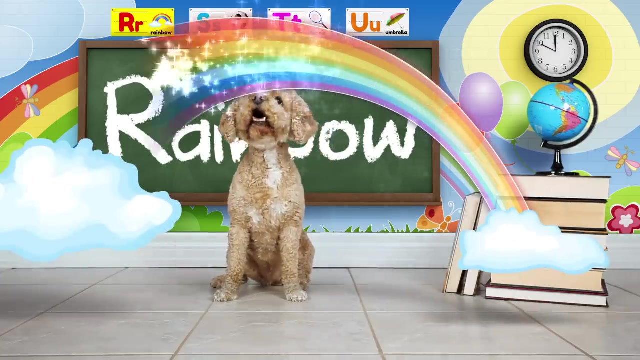 The letter R sounds like R. R like the word rocket, like the word rocket, like the word rocket. Another word that starts with R is Rainbow, Rainbow. So pretty, So pretty. Do you know all the colors of the rainbow? Do you know all the colors of the rainbow? 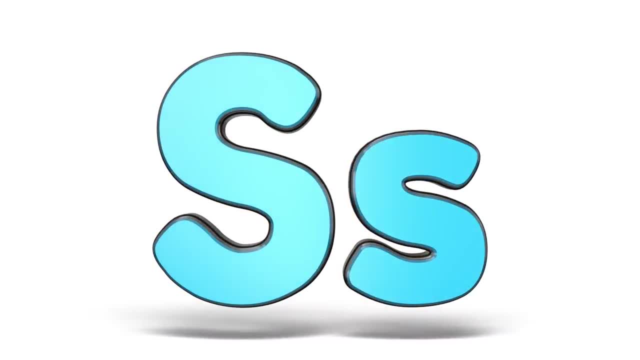 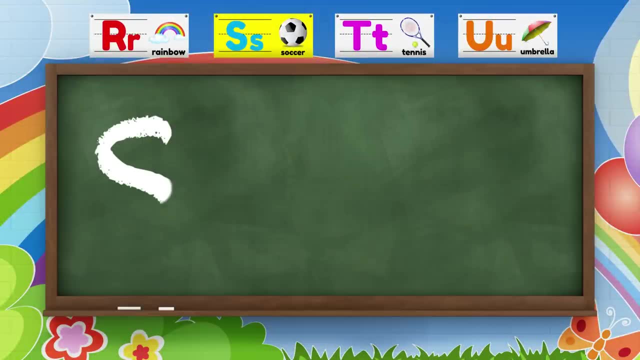 Next up is the letter S, and it looks like this. The letter S sounds like S S. One word that starts with S is soccer. One word that starts with S is soccer. One word that starts with S is soccer. Look, Lizzy, it's a soccer ball. 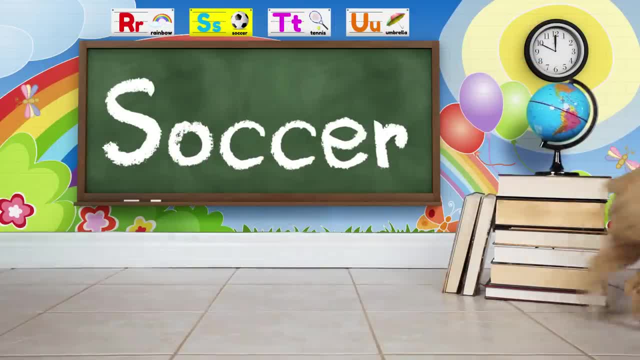 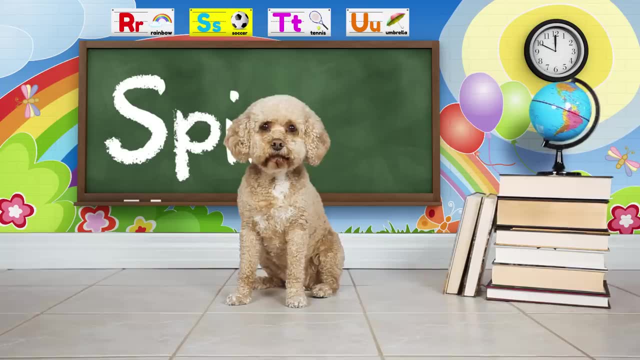 Go get it. Go get it. Another word that starts with S is spin. Another word that starts with S is spin. Another word that starts with S is spin. Why don't you give us a spin, Lizzy? Why don't you give us a spin, Lizzy? 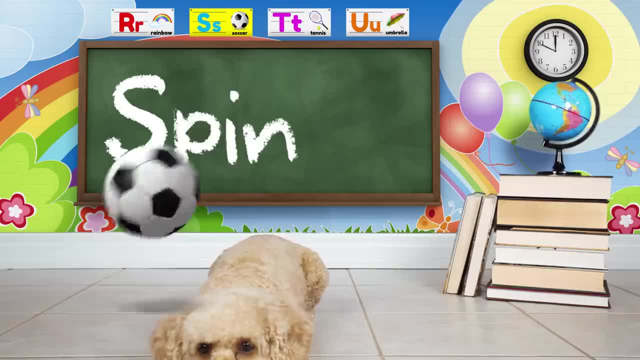 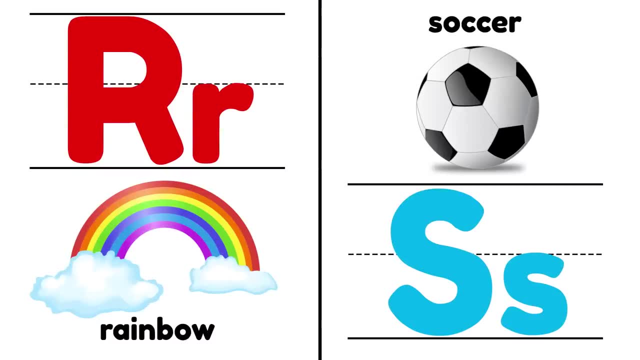 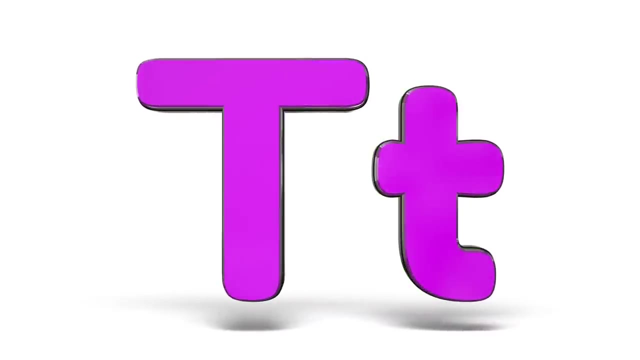 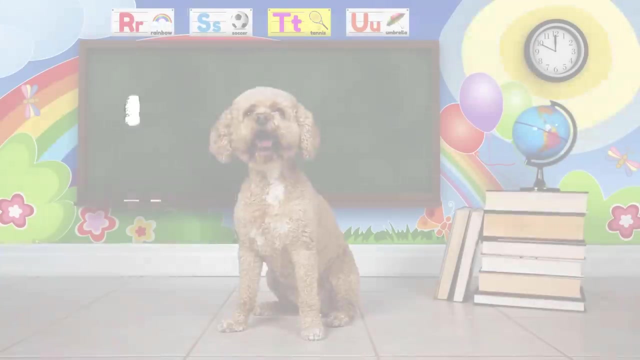 Good girl, Look out, here comes another soccer ball and it spins too. and it spins too R R R for rainbow S, S, S for soccer. Next up we have the letter T and it looks like this. The letter T sounds like T, T- One word that starts with T. 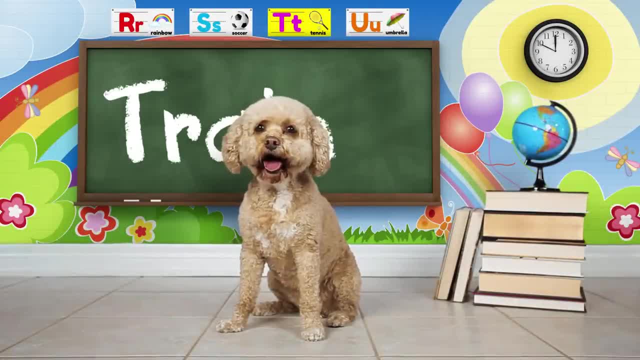 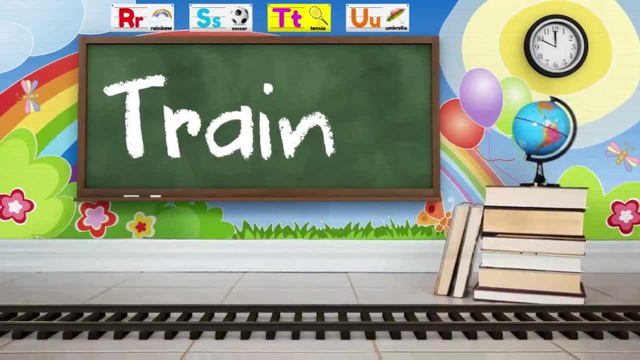 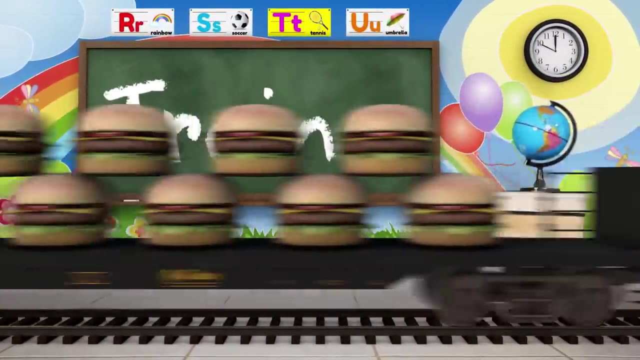 is train. Hey, Lizzy, here comes the number train. Better get out of the way. Better get out of the way. Remember when you went for a ride on that train, Lizzy? That was so much fun, That was so much fun. Another word that starts with T: 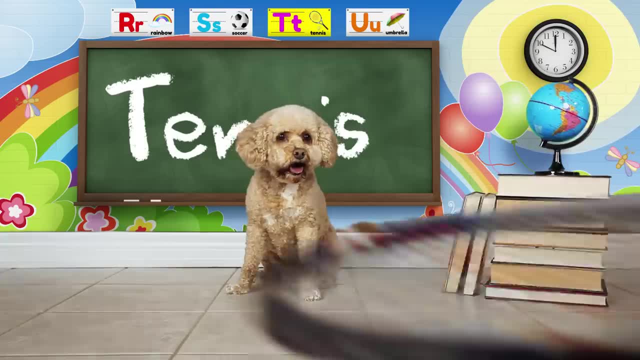 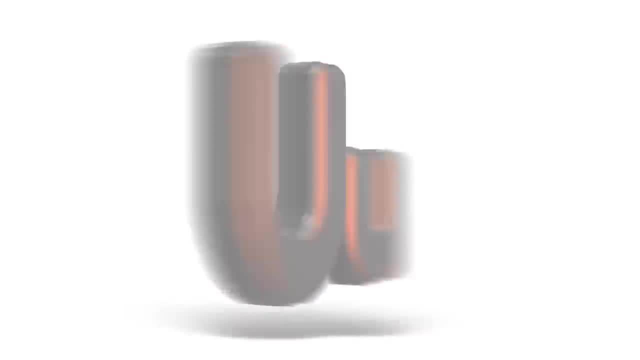 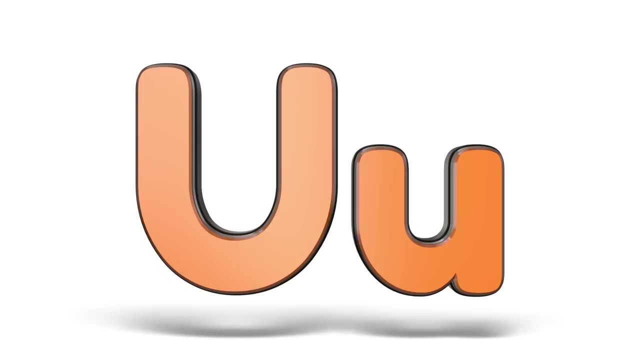 is tennis. Lizzy doesn't know how to play tennis. Lizzy doesn't know how to play tennis, but she sure loves tennis balls. but she sure loves tennis balls. The next letter of the alphabet is the letter U, and it looks like this: The letter U sounds like: 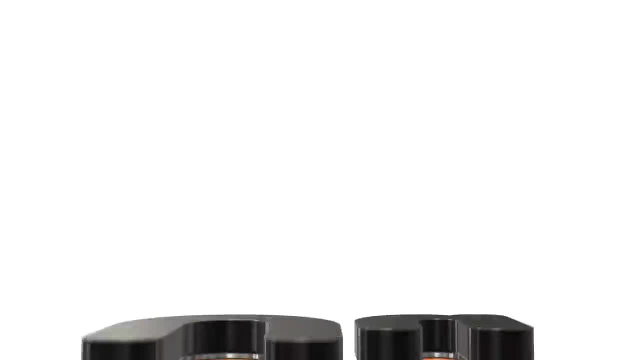 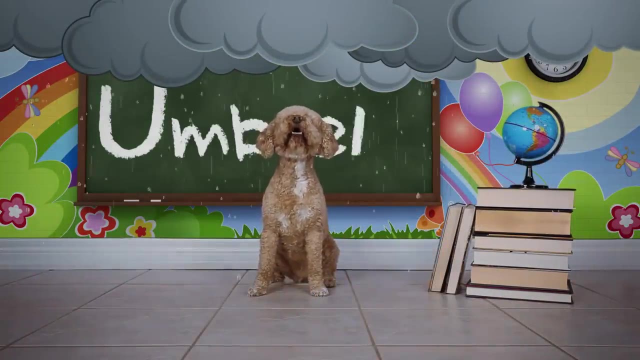 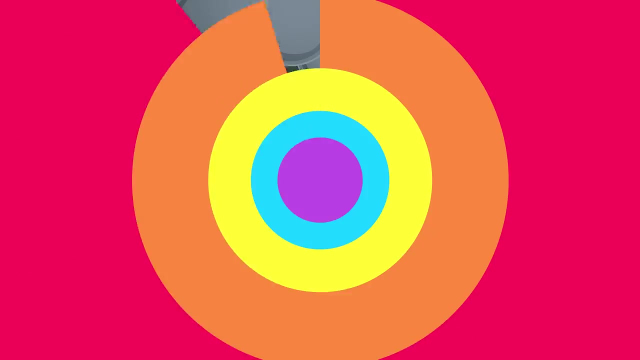 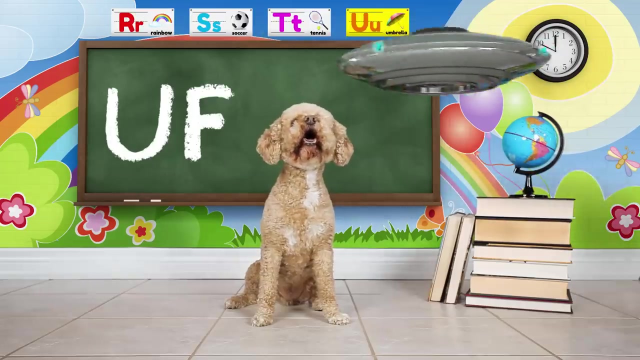 U or U. Uh oh, it looks like it's going to rain. Better get an umbrella. Better get an umbrella. The word umbrella starts with the letter U. The word umbrella starts with the letter U. Hey, what's that? It looks like a UFO. The word UFO starts with the letter U. 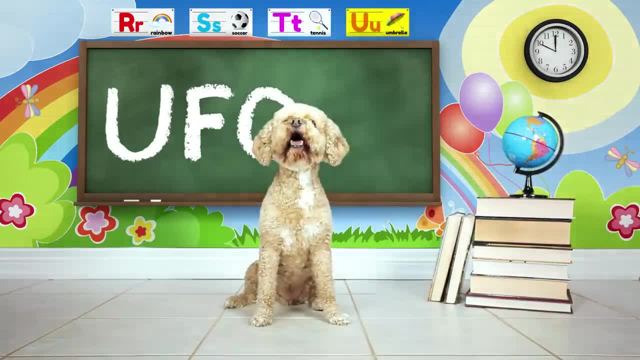 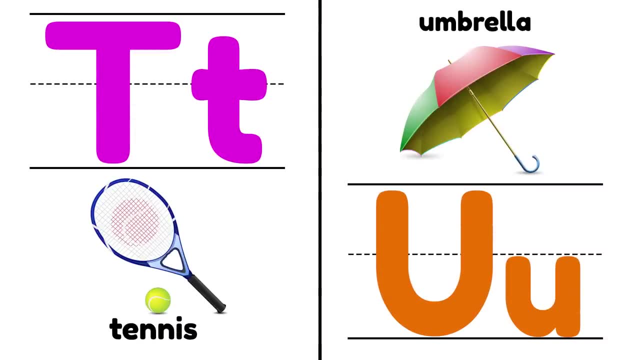 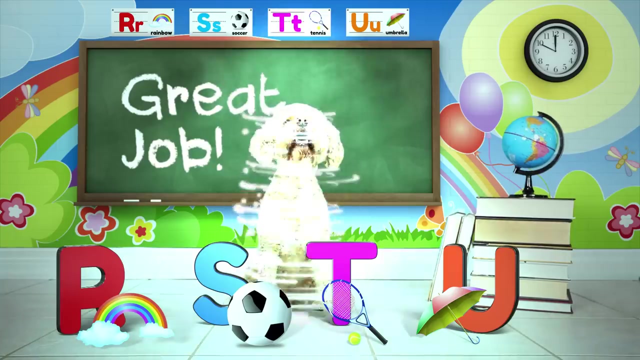 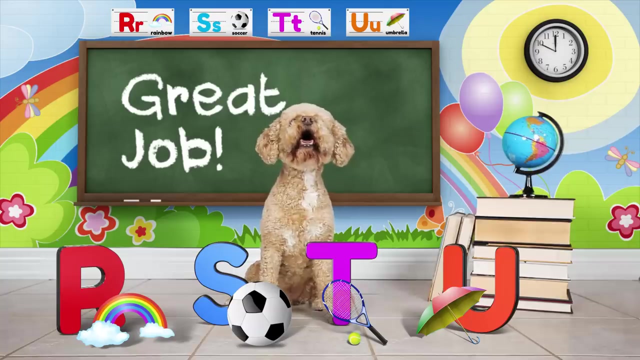 The word UFO starts with the letter U. Okay, one to beam up: T T, T for tennis, T T for tennis, T T for tennis, T T T for tennis, T T for tennis. Welcome back, Lizzy. I hope you had a fun space adventure. I hope you had a fun space adventure. 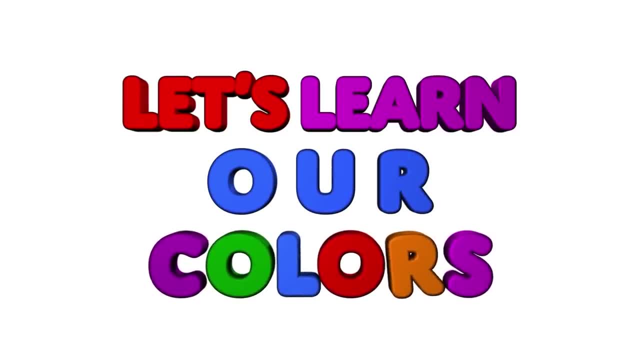 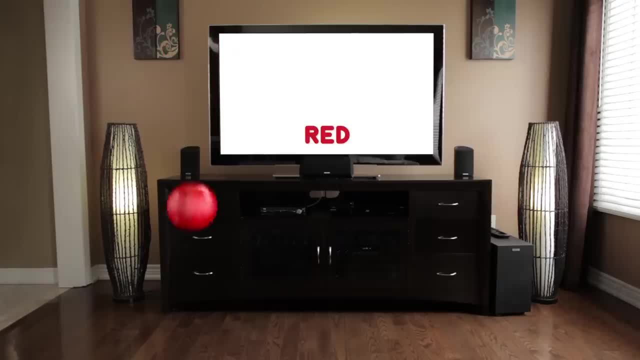 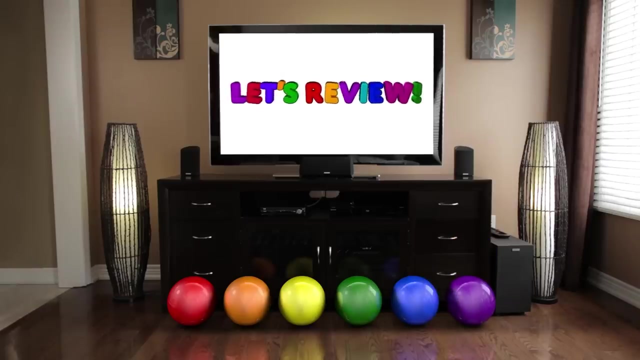 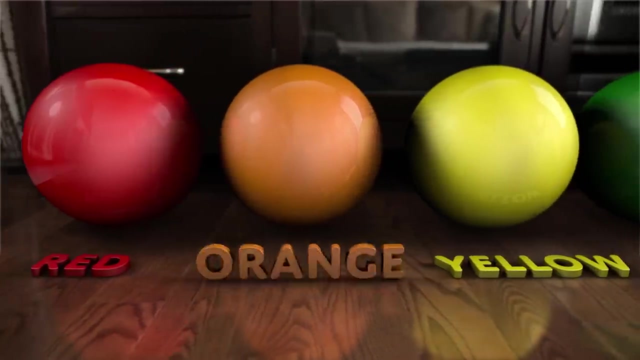 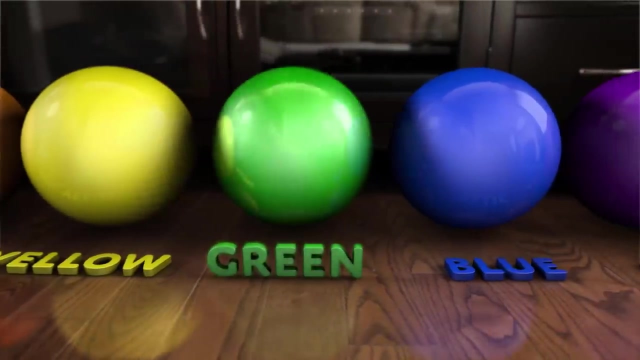 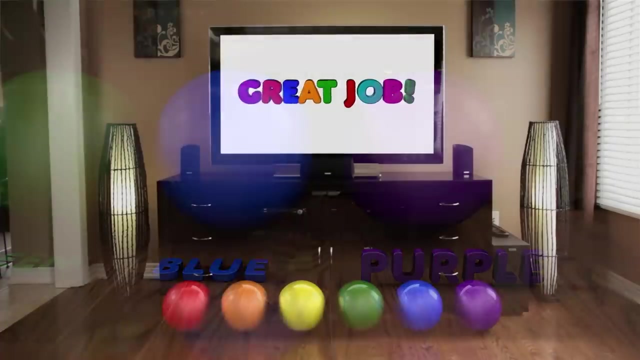 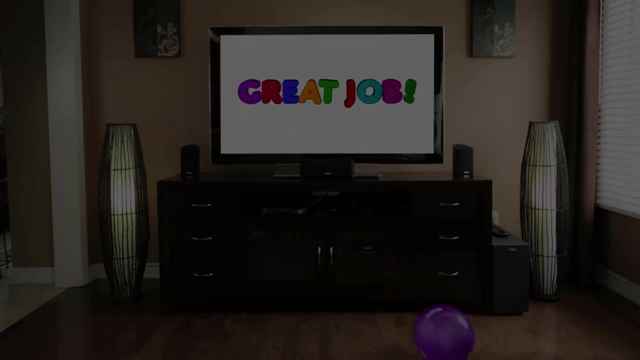 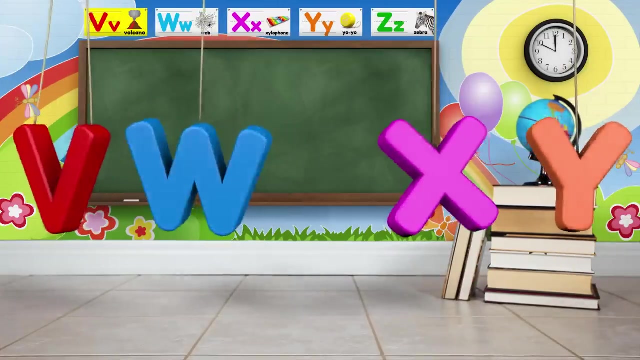 Let's learn our colors: Red, Orange, Yellow, Green, Blue, Purple. Let's review Red, Orange, Yellow, Green, Blue And purple. Great job, Lizzy. watch out, Silly dog. Hey Brainiacs, It's time to learn more of the alphabet with Lizzy. 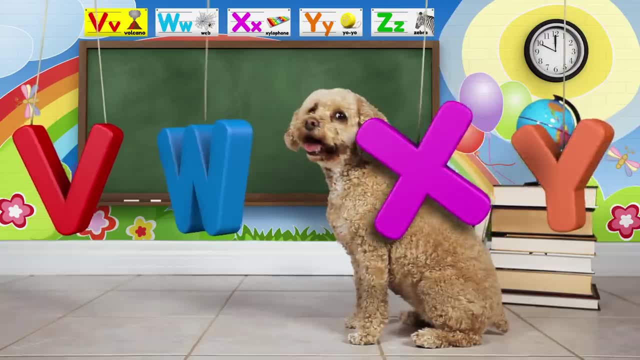 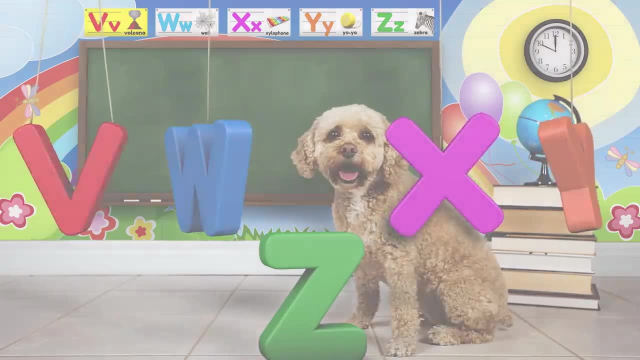 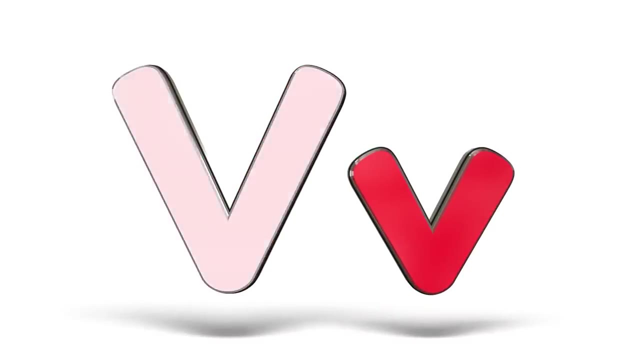 Now we're going to learn about the letters V, W, X, Y and Z. Hey, where's the Z? There it is. Our first letter for today is the letter V, and it looks like this: This is a capital V. 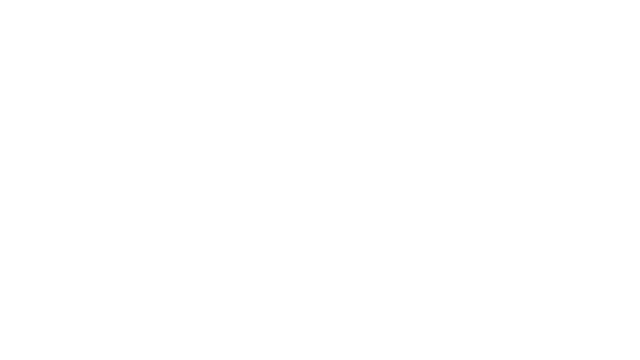 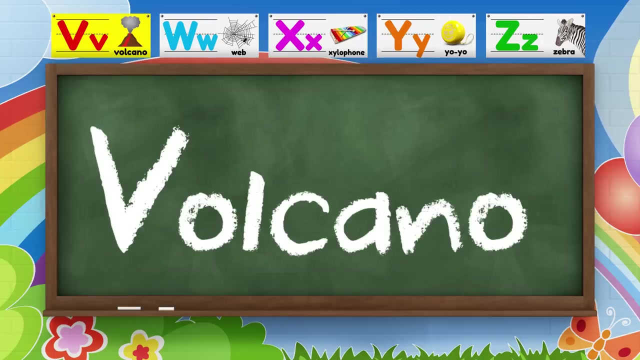 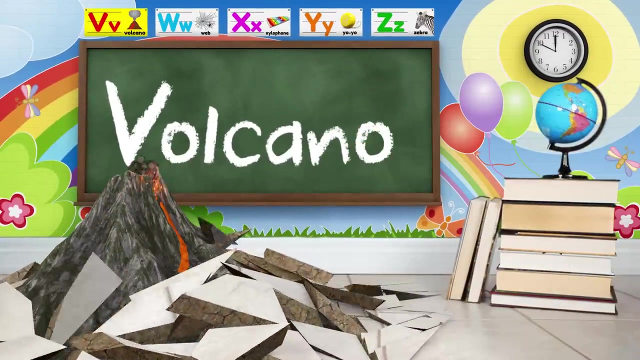 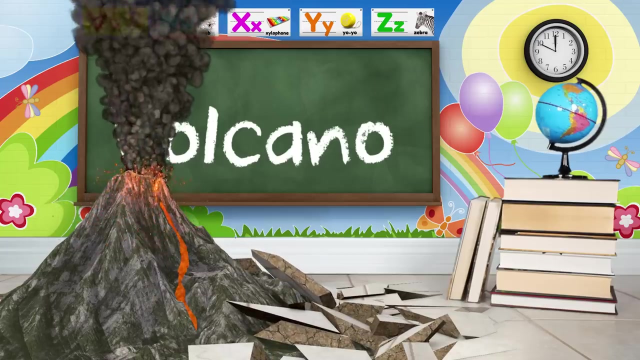 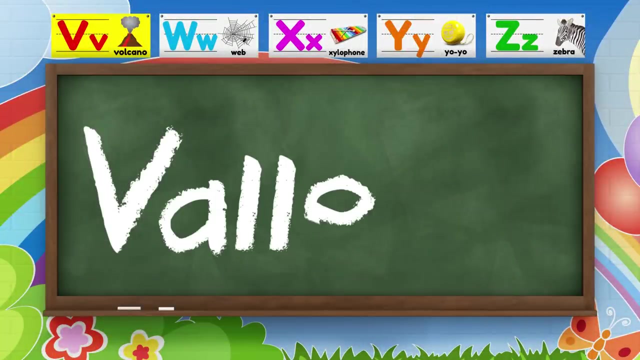 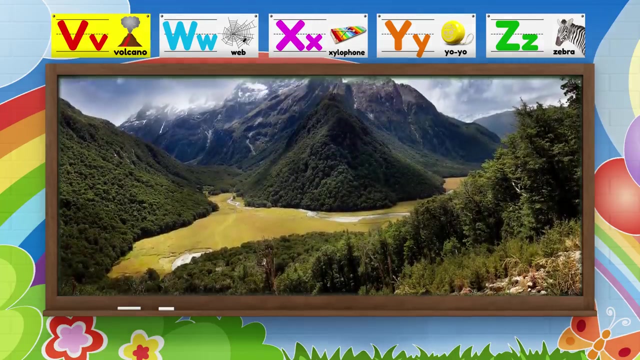 This is a lowercase v. The letter V sounds like V, V like the word volcano. Whoa cool, Look at that volcano. Another word that starts with V is valley. A valley is a flat area at the bottom of mountains or hills. we took this photo of a valley when we 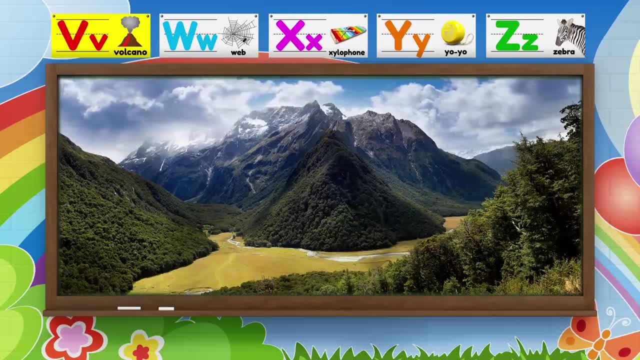 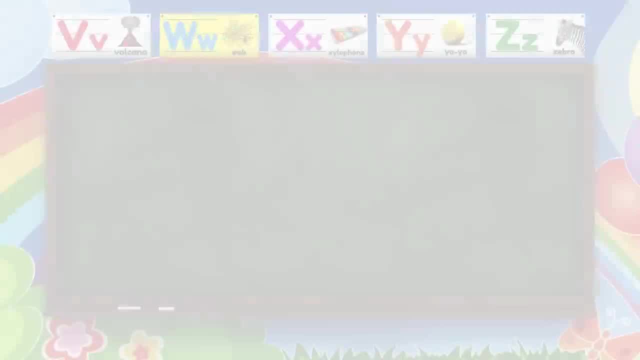 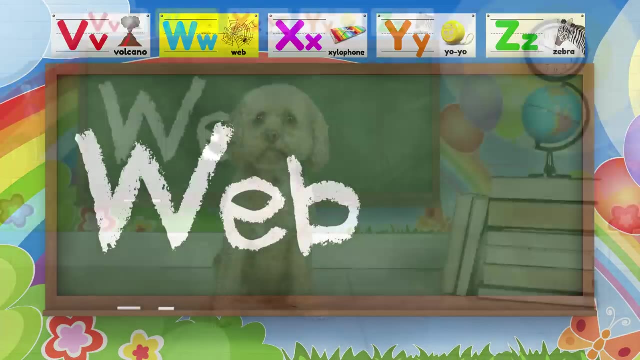 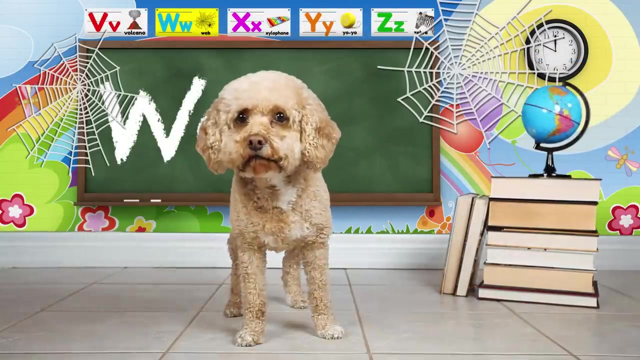 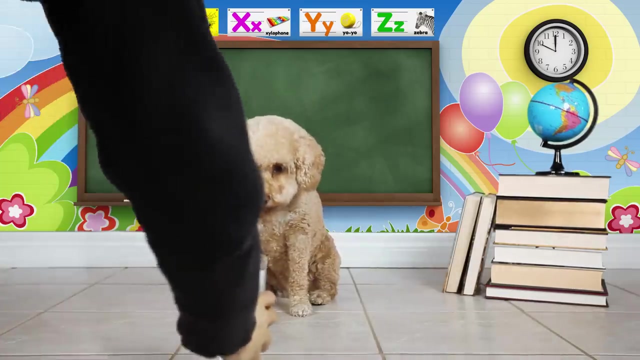 climbed to the top of a mountain in New Zealand. next up is a letter W and it looks like this. the letter W sounds like whoa, whoa, like the word web. hey, what does spider-man do? he shoots webs to stop the bad guys. when Lizzie gets thirsty, she likes a nice, cool glass of water. 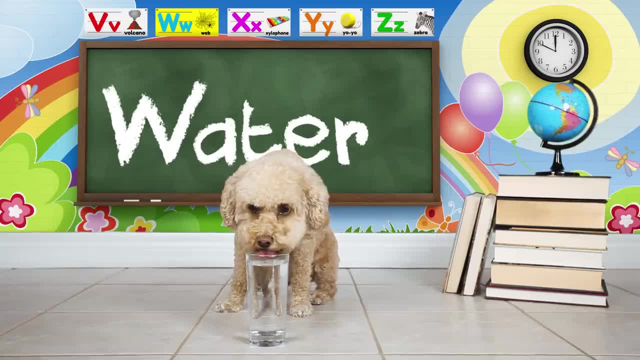 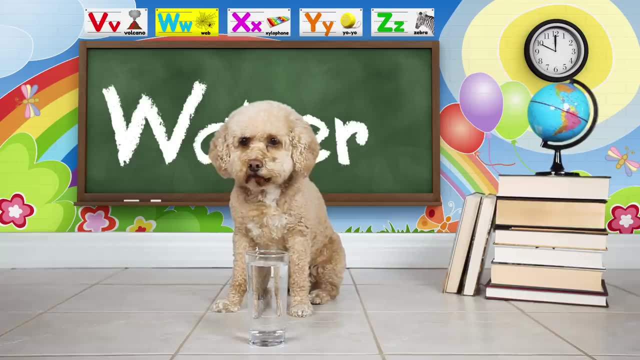 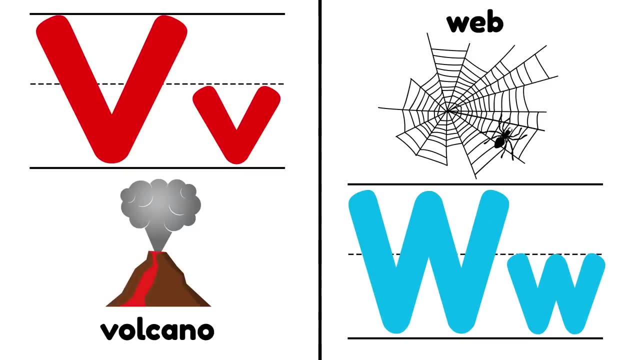 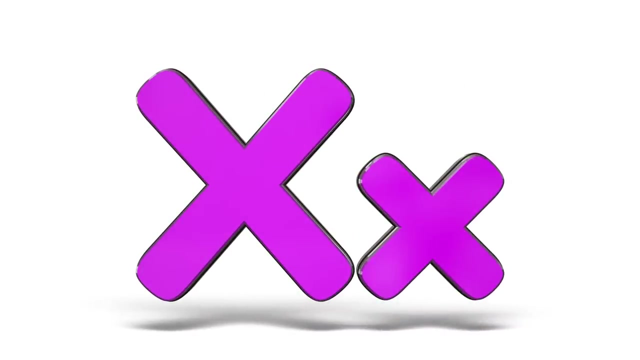 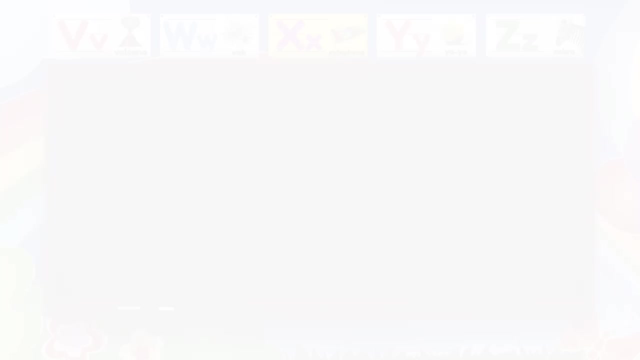 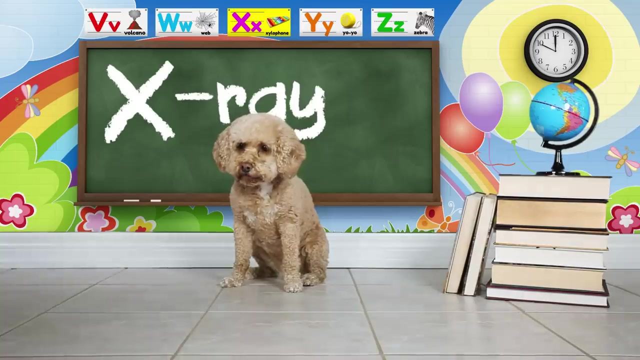 the word water also starts with W, the. the V for volcano, what, what W? W for web. next we have the letter X and it looks like this X sounds like, or one word that starts with X is x-ray. let's use our x-ray machine to see what's inside this box. 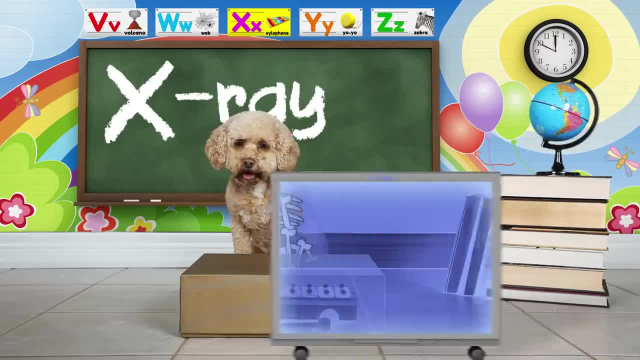 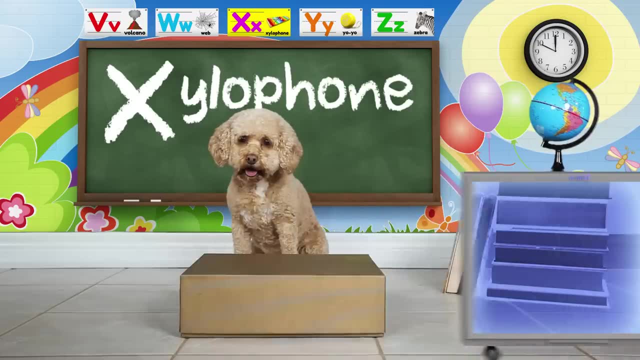 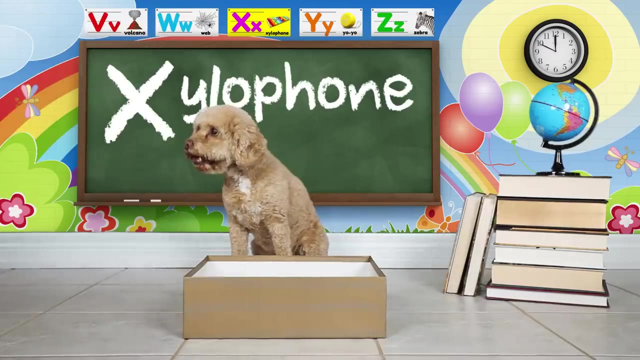 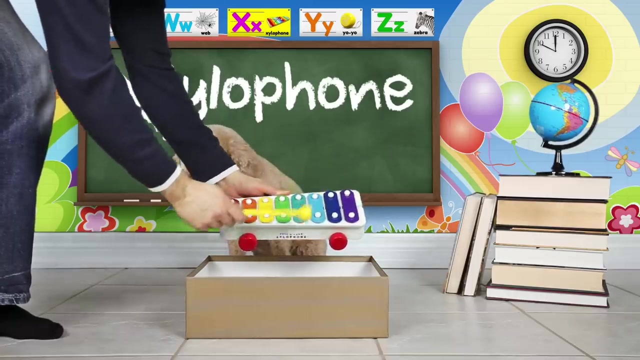 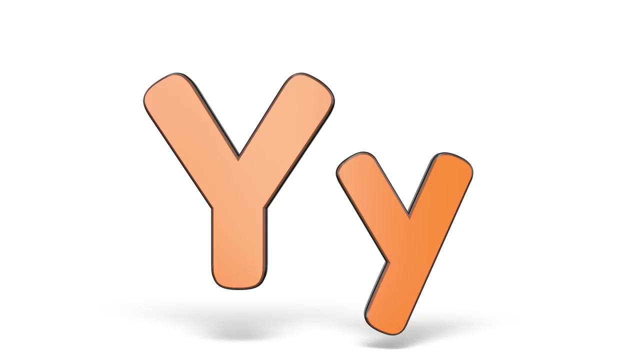 hey, it's a xylophone. xylophone also starts with the letter X. let's see if we can play something on the xylophone. the next letter of the alphabet is a letter Y and it looks like this: the letter Y sounds like yeah, yeah. 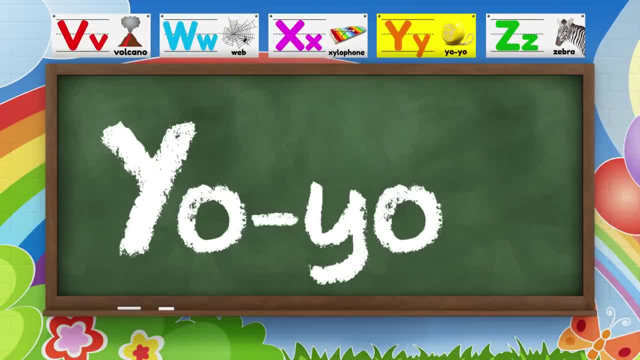 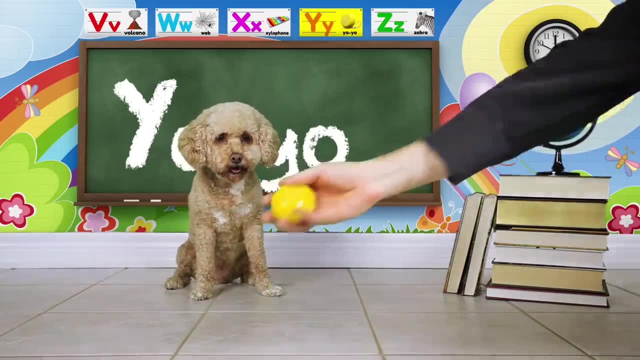 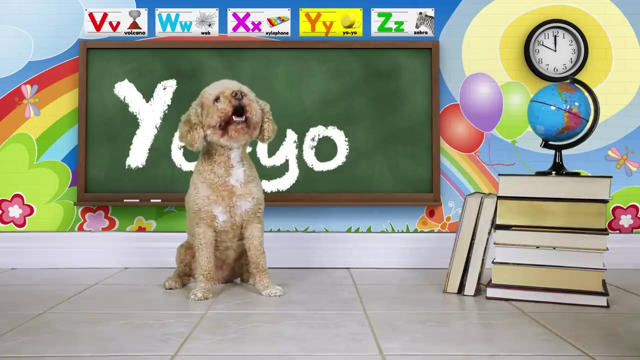 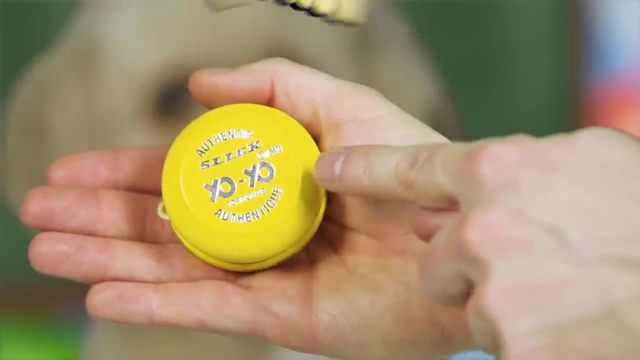 yoyos are a lot of fun, but it takes a lot of practice to get it right. the word yo yo has two Ys. yo-yos are a lot of fun, but it takes a lot of practice to get it right. this yo-yo is the color yellow, and yellow also starts with the letter Y. 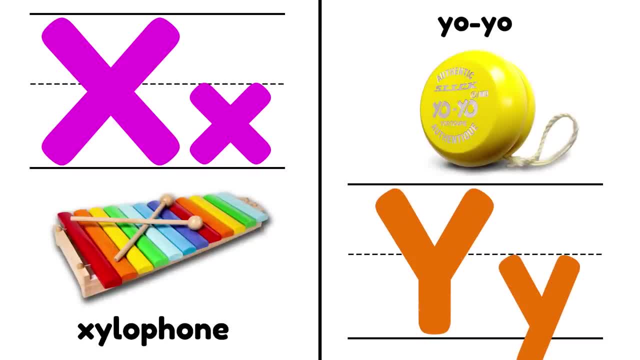 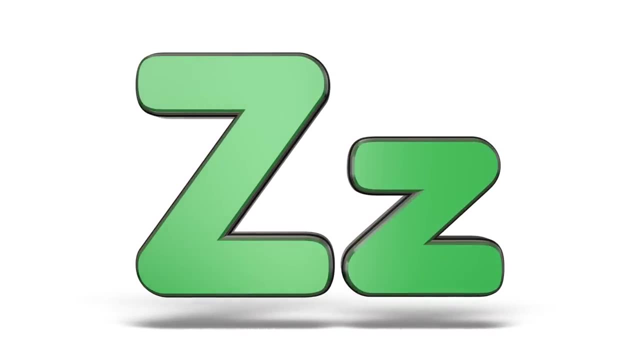 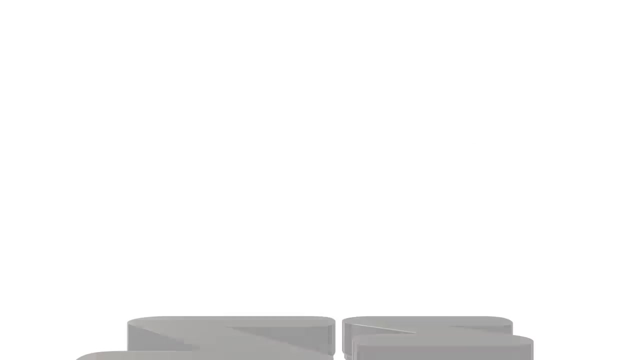 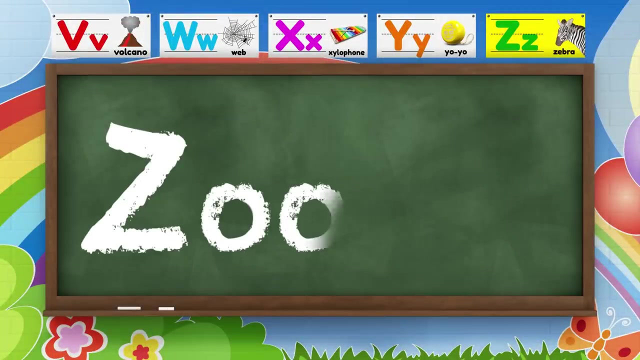 or yellow or yellow, I don't know what that means. X for xylophone, Y for yo-yo. The last letter of the alphabet is the letter Z, which is also called Zed. The letter Z sounds like One of our favorite places to visit is the zoo, and zoo starts with Z.